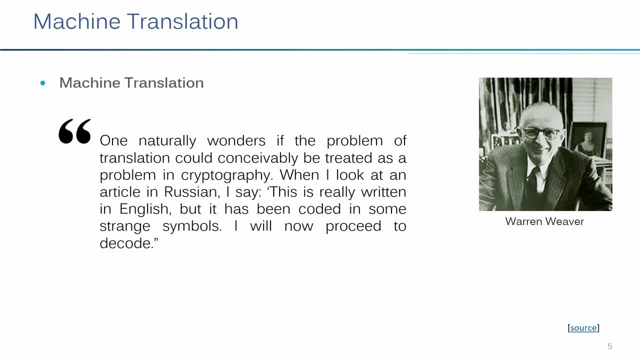 So how he defined machine translation. So one naturally wonders if the problem of translation could conceivably be treated as a problem in cryptography. When I look at an article in Russian I say this is really written in English, but it has been coded in some strange symbol. 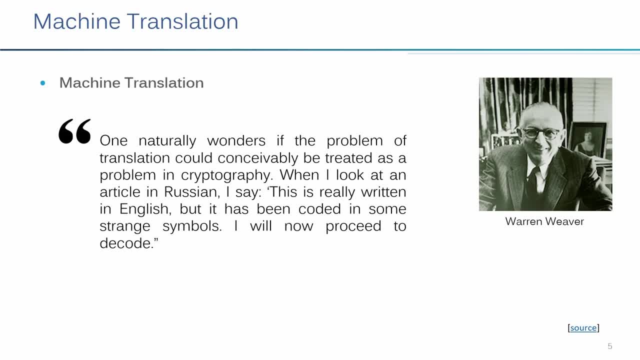 And I will now proceed to decode. So this idea of decoding a symbol that you don't know how it looks like or what the relationship is, it's pretty much the problem of machine translation. Of course, in practice it's not as nice as right here. 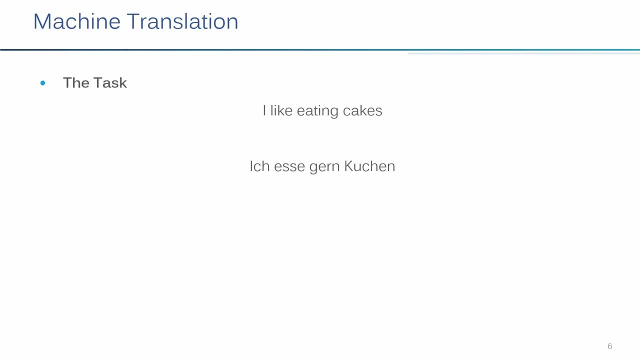 Hopefully we'll be able to show, including some problems that we have with machine translation. So what is the task? pretty much, You have a. In this case you have a source Sentence- I like eating cakes- And then you translate that to: 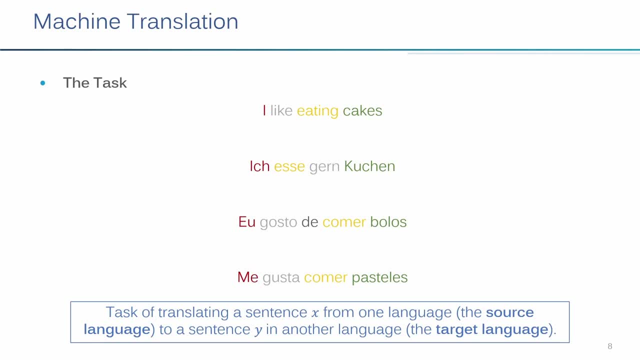 If you're lucky enough, things will align, And that's really nice because you have one-to-one translation. So I, it's ich, ich, eu, Eu has an inflection. it's me Like, gern, gosto gusta. 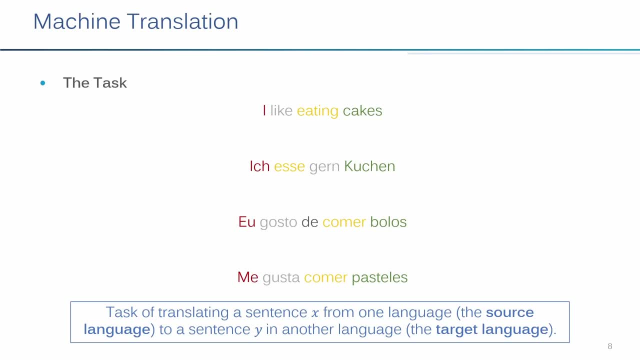 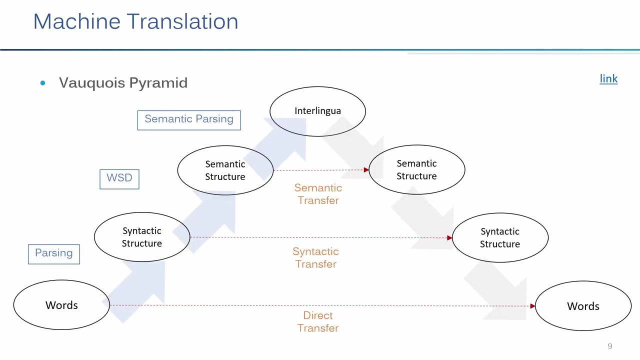 So these words are aligned. However, that's not actually the case for a bunch of scenarios, And we'll see some of them. Okay, Another way for us to take a look into how machine translation is, or translation the task is itself, is through the Vacuo pyramid in a way that we're trying to move from either from words. 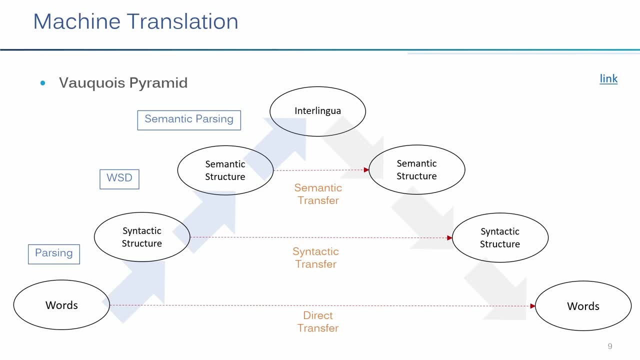 a synthetic structure, a semantic structure, and one target language- Sorry- And one source language, So you can move from one language to one target one, And translation it can occur in different steps on this structure, So you can move directly from word to word if you have this alignment there. 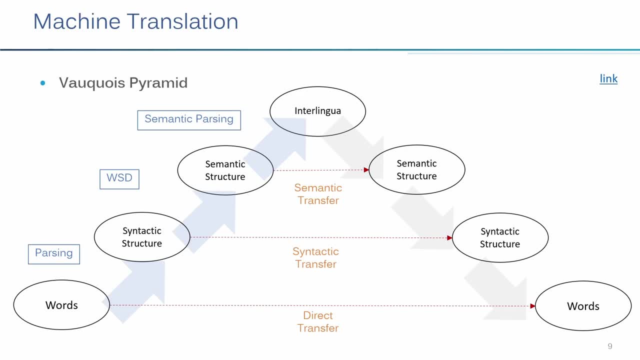 And if you have this one-to-one translation, You can use a synthetic structure. In this case, you have to deal with word sense- immigration. Or sometimes you translate a sentence, the meaning of that sentence, into another meaning, In this hierarchical model. 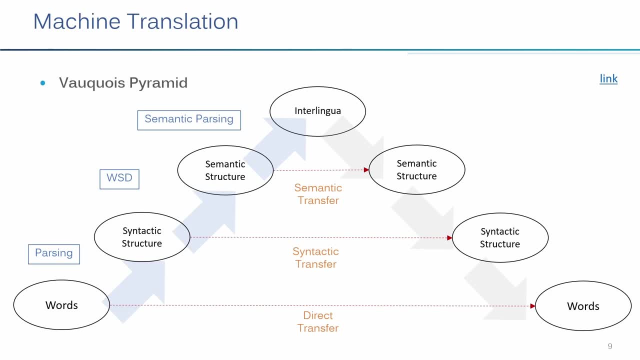 there's also this interlingua, which is supposed to be something as high level that every language should be able to be translating to that And this should be common to all the languages. This is debatable. There was some attempt to do this with how was that language on the Internet? 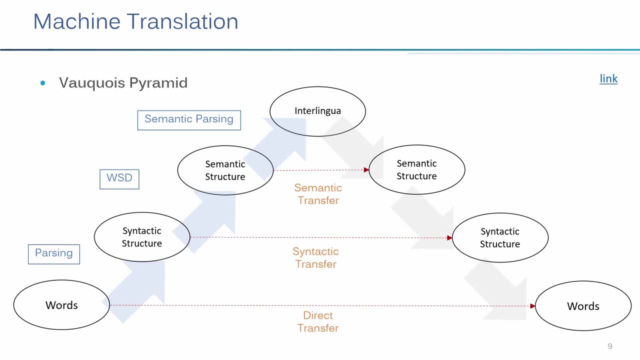 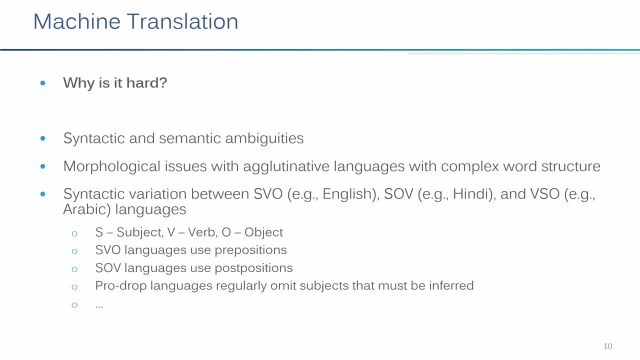 They tried to propagate that It was not working, Esperanto or something. a couple of years, a couple of years, many years ago. But be that as it may, Why? machine translation is quite hard. We have some problems with that. One of them is synthetic and semantic ambiguities. 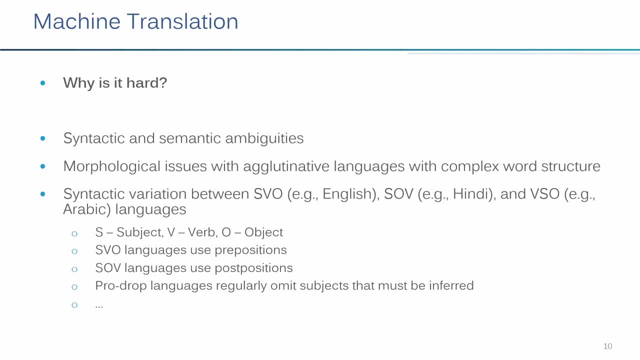 Imagine that when we were talking about words in the same language, we already have problems in disambiguating their meaning. Imagine now that you move this to different languages. And when I say different languages, think also outside the box, not necessarily just natural text. 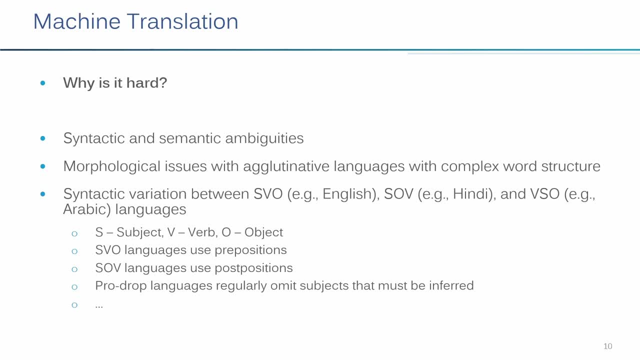 You can have code or signals, for that matter. Although code is weird, It's way less ambiguous than language per se. but in any case also morphological issues with agglutinative languages, with complex word structures, some languages- I think we showed that in the second class or the first with Turkish, also with German. as you keep putting the words together, it's hard for you to break it down. 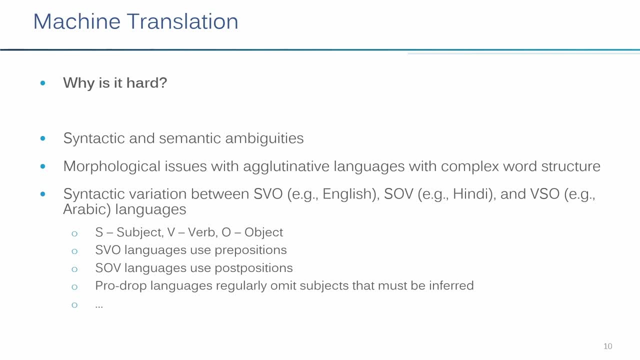 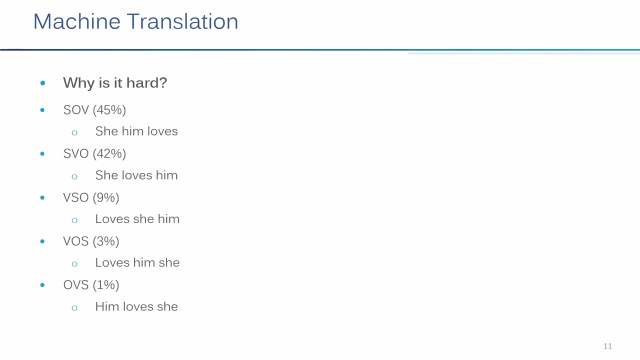 Also the synthetic variation between subjects, Also the synthetic variation between subjects, Also the synthetic variation between subjects: Subject, verb and object. In English we have this order: subject, verb and object. But some of them they don't follow this structure, which makes things a bit complicated when you translate it from one language to the other, because that might change the meaning. 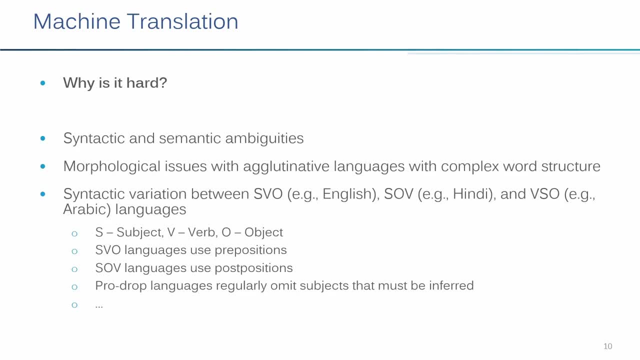 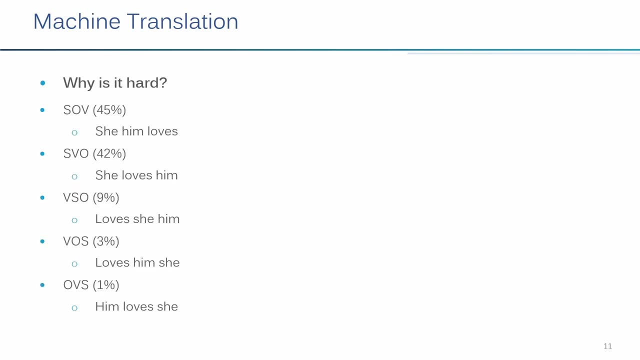 Just to give you some idea how the synthetic variation looks like for us. So in subject, object verb we have, she him loves. If we have Subject verb and object we have, she loves him. 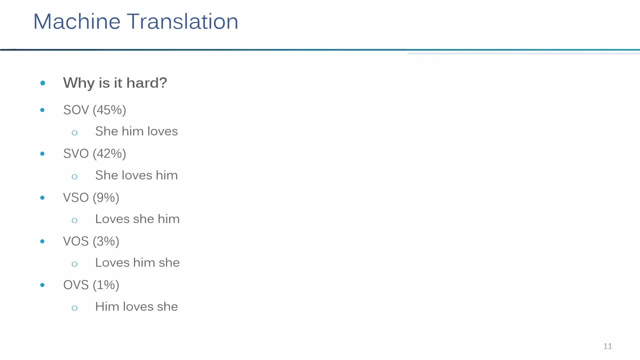 This is somehow closer to our language. And then you have loves- she him, Loves him, she Him loves she, And things start to get kind of confused, Even for us to read. imagine for you to code that. 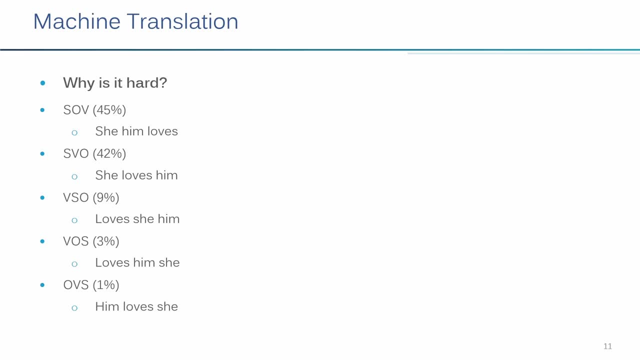 And I'm pretty sure there are way more other complex structures than this. This is just a snippet. Yes, Yes, Oh yeah, This is a really rough estimate. And how languages, non-languages, they are categorized between this synthetic structure. 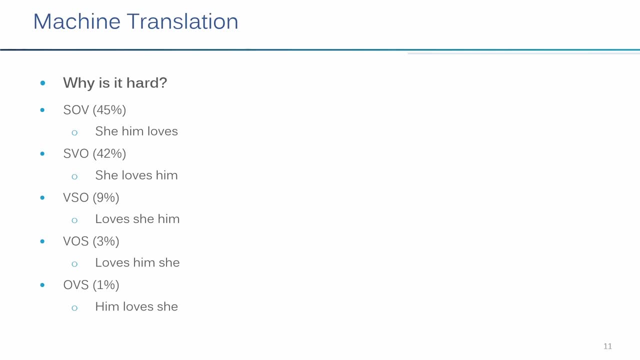 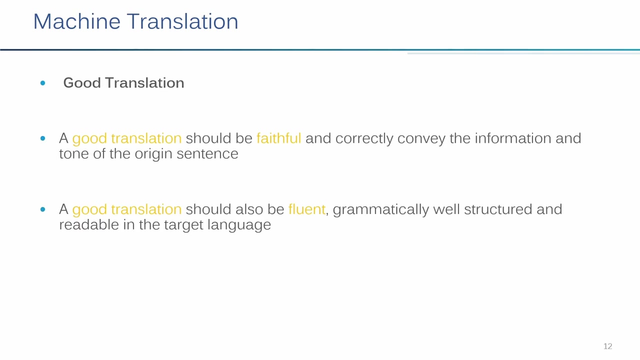 But I highly doubt that this is considered low-resource language. So, if you consider English, German, Portuguese, Spanish and so on, they are divided. This is the division that they have in this structure. Okay, So what is a good translation? 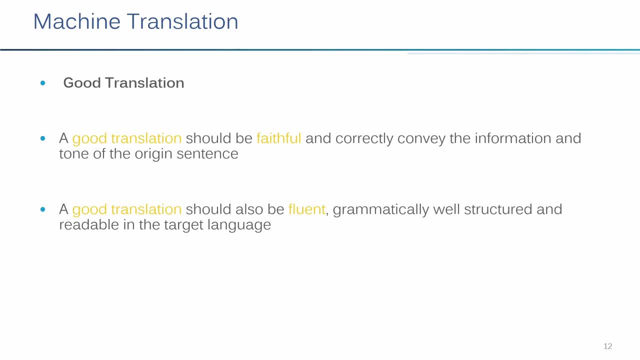 It's pretty much what we have for a good language model. If a translation Is faithful and correctly conveying the information and tone, it is debatable also of the origin sentence. This is a good translation And of course it should be fluent. 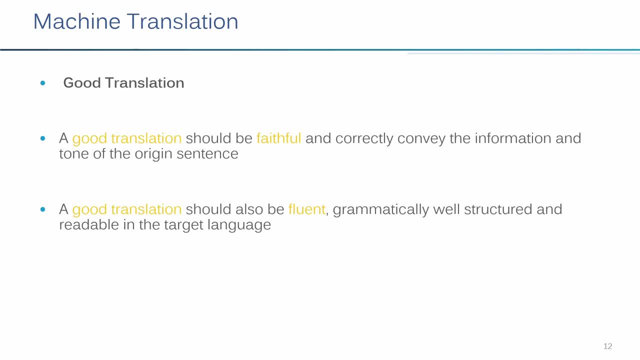 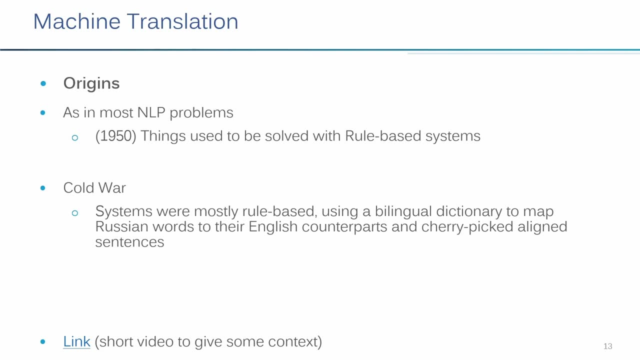 Otherwise it's not a good translation. So what are the origins and how things actually work out for machine translation back in the day? As- And Hopefully we didn't? We don't propagate this that much, But again, NLP is always divided in three parts. 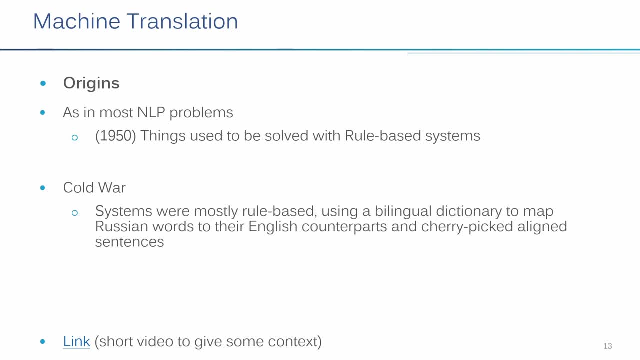 Rule-based systems, machine learning with statistical features, handcrafted features and then neural network architectures. So around the 50s things used to be solved with rule-based systems, a lot of rules And very cherry-picked rules and cherry-picked alignments, which was also a big problem. 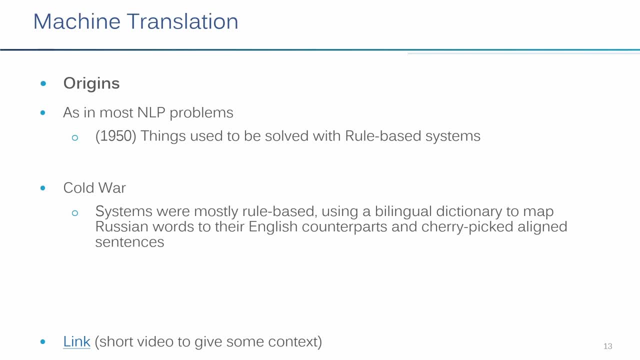 So systems were mostly using this Very specific, Very specific rules to create this bilingual dictionary to try to map one language to the other, Just to give you Later on if you have time. this video is like five minutes. You can take a look how. 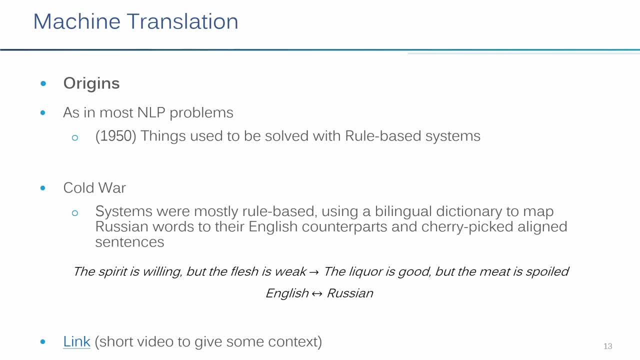 What are the problems And people, when they were using machines to do machine translation, they were already saying that, yes, if you have to translate technical terms, this will be done in the next five years. Haha, It was definitely not. 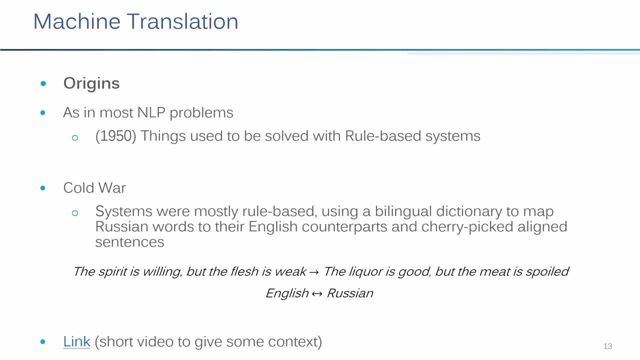 But now it's Kind of: But poetry and more creative text. this is hard to do And we don't think. We, as in that time, don't think that this will be possible. Things change a bit, But just to give an example, because of this cherry-picked alignment that they had in words, things like, if you would translate: the spirit is willing but the flesh is weak, to Russian: 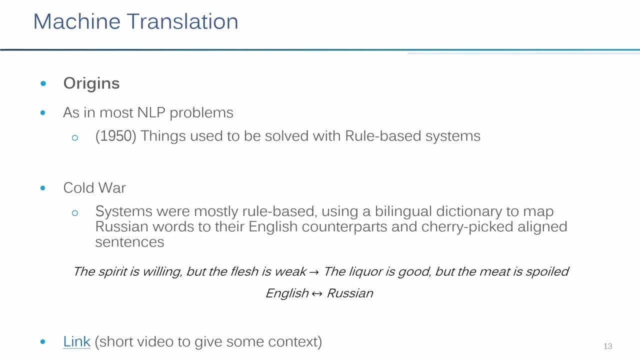 And then you get back to this translation to English. because of the words that they use, This sentence here the translation would be: the liquor is good, but the meat is a spoil, So not actually the meaning that we're hoping for. that 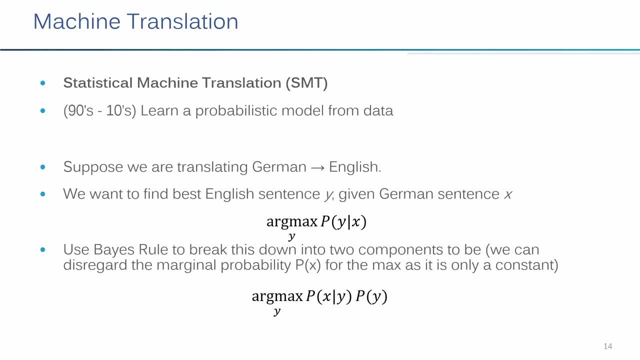 But yeah, They have a bunch of other examples. So, moving on to the 90s to 2010s, the idea was pretty much to learn a probabilistic model from our data, a lot of data. And then suppose we're translating German to English. 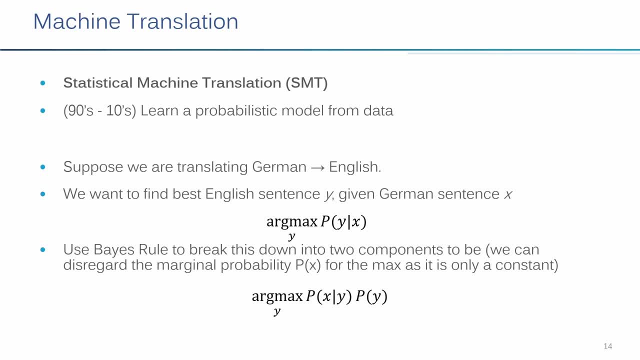 Pretty much we want to find the best English sentence Y given a German sentence X as our context, whatever the size of that sequence is. So in other words, and we can wiggle this around, and pretty much you would have two models. 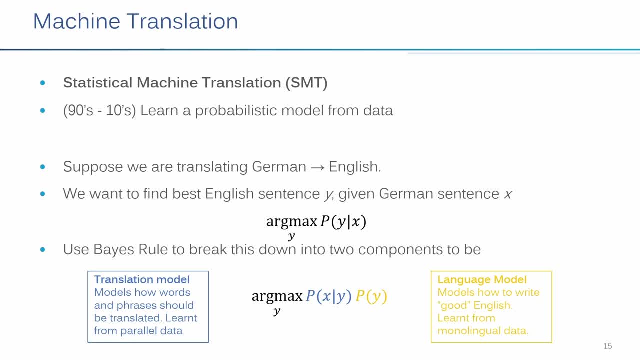 One translation model that models how words and phrases should be translated, And you learn this from a parallel data, And this is done since the dawn of days, pretty much. We still use a lot of Parallel data. in fact, There are ways to cope if you don't have a line of parallel data. 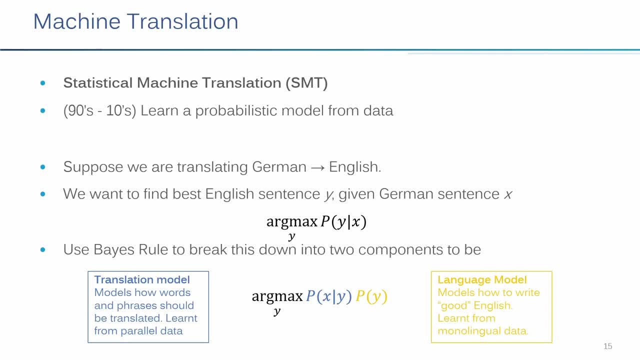 You can create them relatively easy, really, between quotes, And on top of this translation model, you also have a language model, which is pretty much what we have done so far. So this model: how to write good English and learn from normal monolingual data- 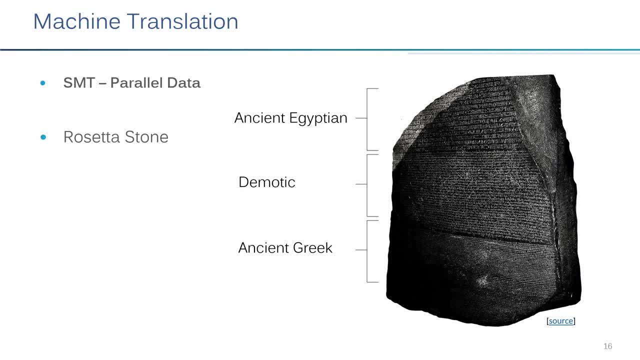 Okay, Just to give you Some idea. And again, every single class that talks about machine translation, they will talk about Rosetta Stone as well. This is one of the very first attempts to kind of align and produce- Not exactly align, but to produce a parallel data in which you would have ancient Egyptian Demotic and ancient Greek. 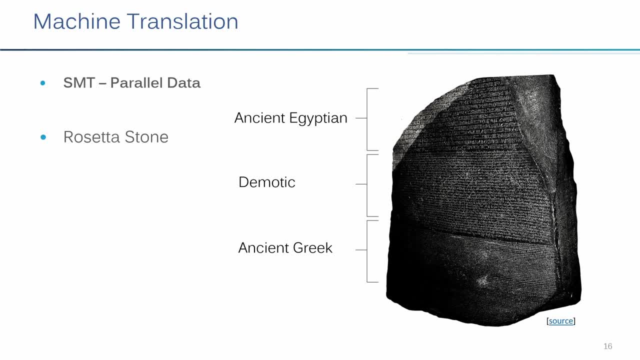 And this idea to use text in different symbols, in different quotes, to convey the same meaning and explore these relationships, for you to have some sort of translation. People have Using this for quite some time. There is a twist on this: On top of parallel data, you still have to deal with alignment. 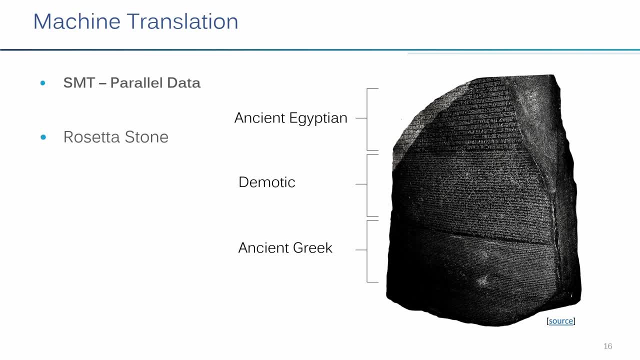 Sometimes this works. Most of times this does not, Not only from different languages, from the same language as well. When you're, let's say, Let's say we're working with paraphrase generation or paraphrase detection, which is pretty much the same language in the context. 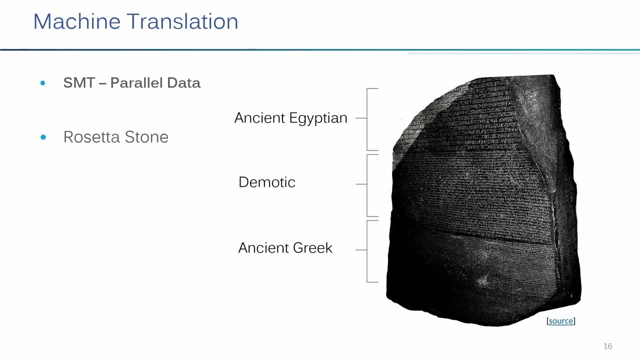 It's not likely. when you paraphrase something in your assignments, in your report, in your thesis, You have a one-to-one word on what you're reading. You have an idea and you transform that into a different sequence, And so you don't have alignment there as well. 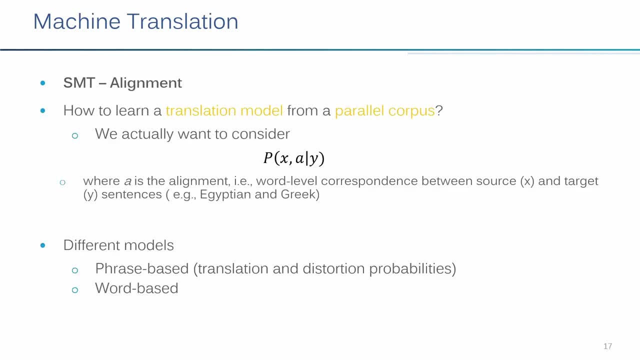 So it's ideal to have alignment, but it doesn't happen in practice- that often So, and how we incorporate alignment. So we actually want to consider what is a sequence target that we have here. an X Gives us, Given our context and our source language, with whatever alignment that we have between those two languages. in this case, 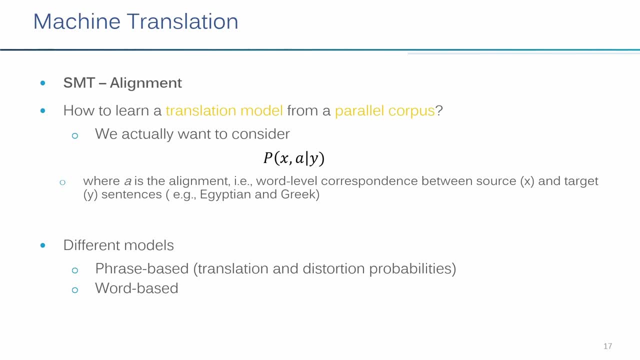 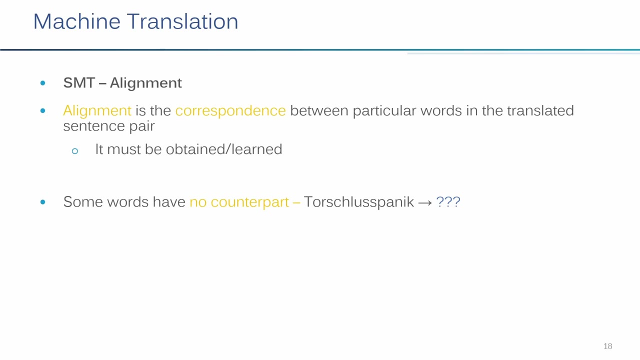 And you have different models how to deal with this. You can work with phrase-based models or we can use word-based ones, But we'll talk about word-based ones. So, yes, Alignment, And I don't think I need to say this, but it's the correspondence between particular words in the translated sequence pair. 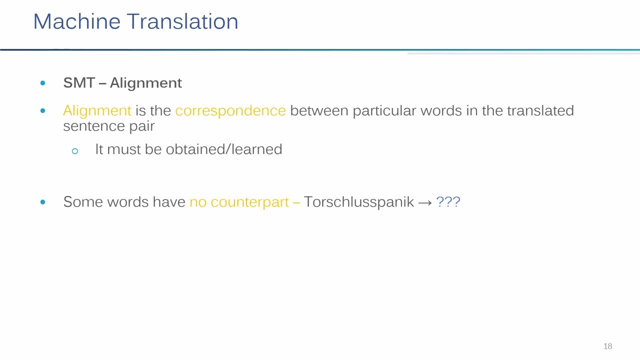 And it must be obtained or learned either by manual alignment or you try to enforce this semantic alignment. Let's say Well, before I give you the solution for this, Can you think about the semantic alignment between different languages automatically? Can you think about 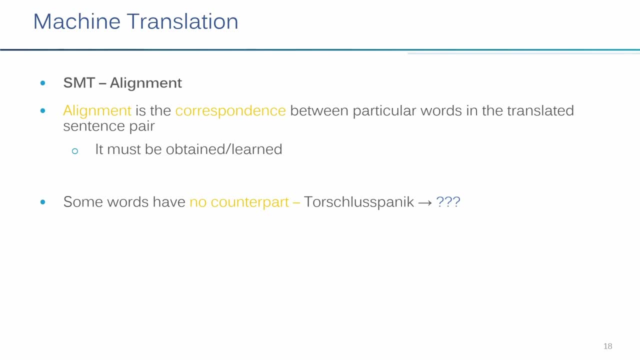 One of the. We learned this approach, by the way. Let's say, I have different languages and I want to align what different languages they mean. How do you put this? How do you align them? Not necessarily going to have different language, the same part of speech. 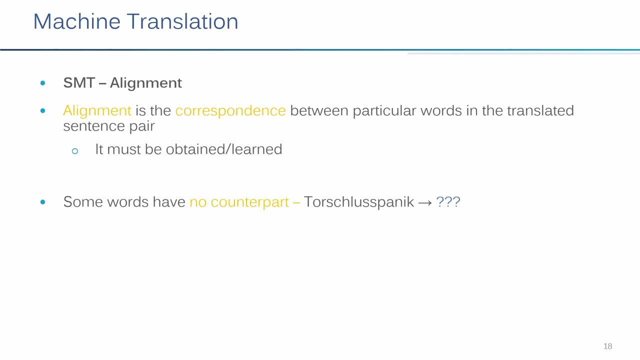 In the semantic level. to make a bit easier: Which technique we learn how to do? Which technique we learn how to transform a set of words, a bag of words, a corpus, into some vector representation? Exactly So if you do, different models for different languages and a set of corpora. 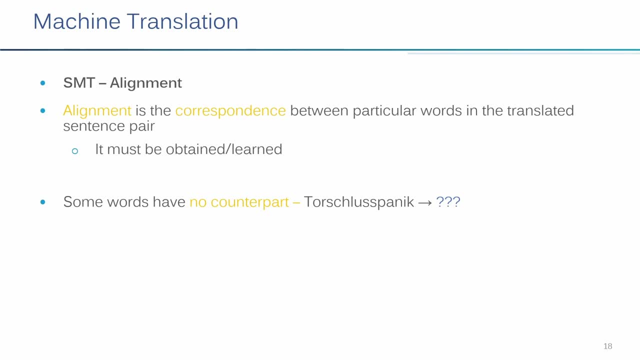 And you, let's say, use the vector space representation from those words in different languages. If they have the same meaning, hopefully it will be some sort of alignment between those words And actually people have done that In 2016,, 2017.. 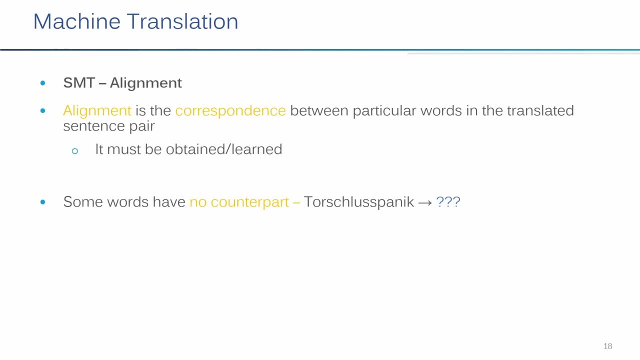 If I remember correctly, Google did this And they found a really good overlap. They use Wikipedia pages- Most likely you have the same Wikipedia page in different languages- And they found out an overlap between Japanese, Korean, Portuguese. There's a fourth language, but I don't remember right now. 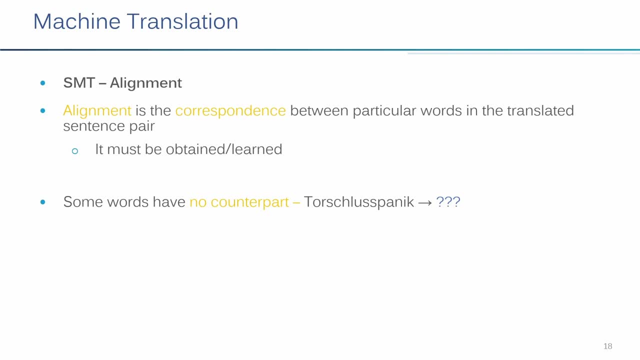 So they were able to provide this rough alignment of semantic Without actually saying: this word here is this word there, Which is actually pretty cool. But coming back to machine translation, Some examples how alignment is not that straightforward. Let's say, you have some words that have no counterpart. 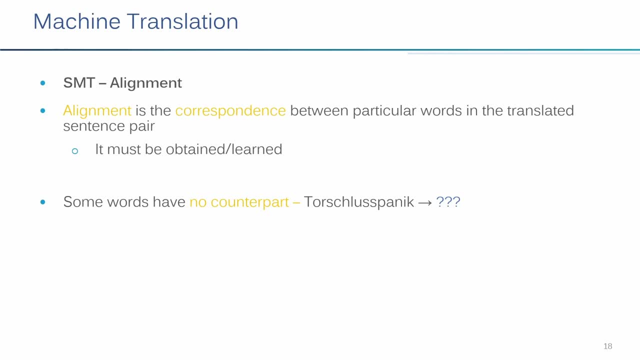 Like. How do you translate that? So, according to my notes, Fear of gate closing is a fear of something is about to finish or end, And then you have this. Well, that's the internet saying, Not me. However, we have some more, let's say, concrete examples. 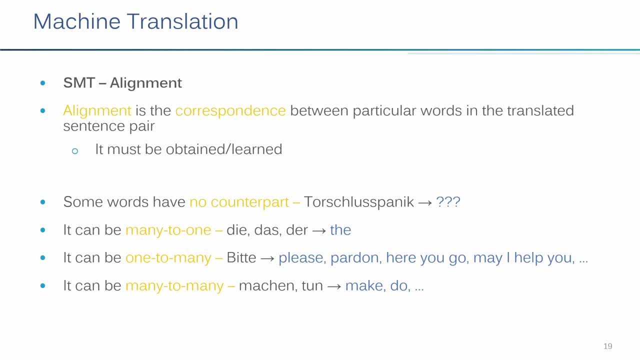 And how things do not align that clearly. We can have many to one Like di, das and der. They all go to der. This is somehow easy to solve, We can be. it can be one to many Like bitter, And then it can be many to many. 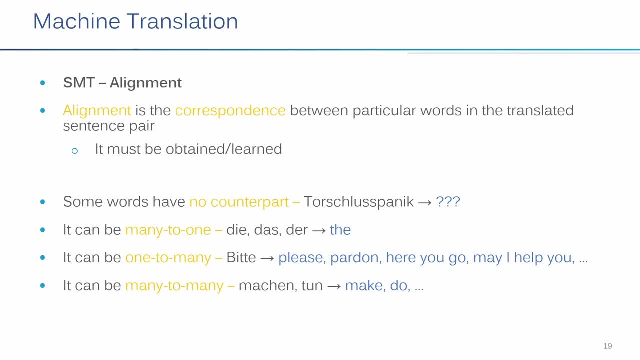 Like mach and tum, And on top of that we have doch Which. how do you translate doch? It has five meanings, by the way. Or halt eben. How do you translate these things Mal in a sentence? Yep, It's really hard when you have those words there. 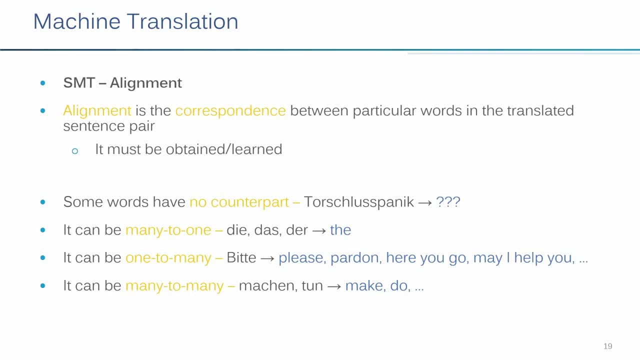 Also- And this is also subjective, I mean people might understand this translation differently. So imagine if to people it's already hard. Imagine putting this into a machine Not fun. So how we do with statistical machine translation. We could enumerate every possible target. 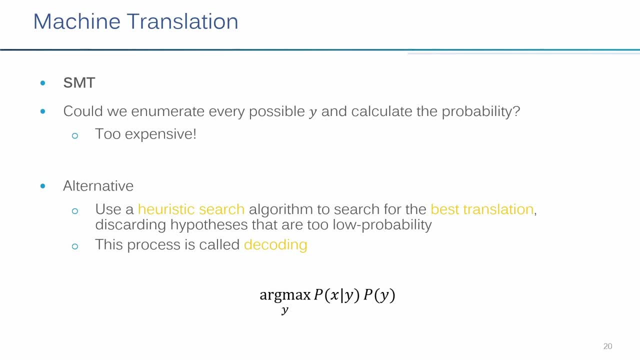 Sentence and calculate their probability. Needless to say, that's the same problem we had with language model. This is simply too expensive. It's too expensive. It's too expensive If you have to compose every single possibility. It's not feasible. 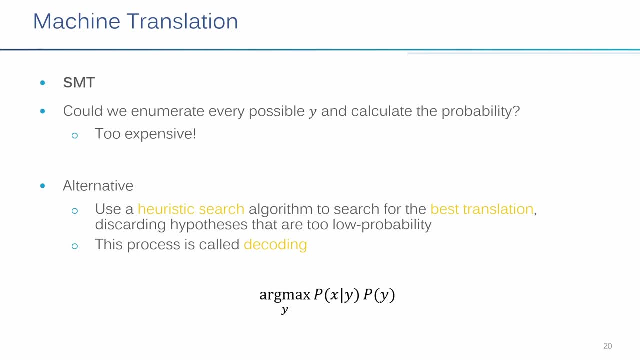 Or we can use an heuristic algorithm to search for the best translation, And this is actually heuristics they use most of times, Every time you have to generate something, Either a new sequence Or a possible chat dialogue system. New text on text generation. 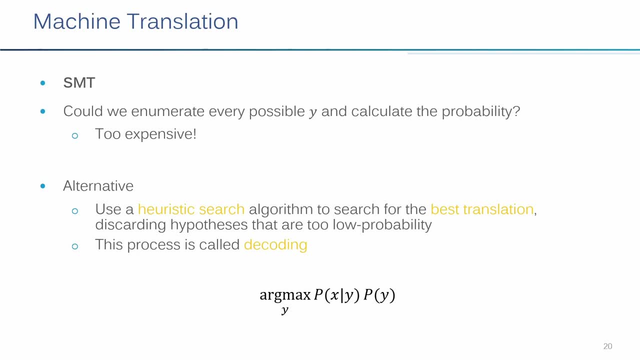 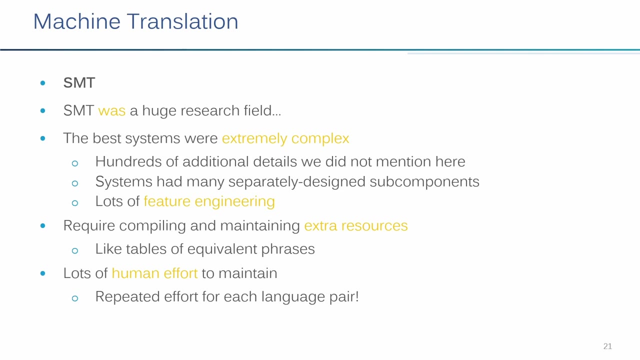 We use things to prune and trim. how much Or how are the most interesting ones you're generating? We'll go over some of them when we talk about sequence-to-sequence models, And okay. So statistical machine learning was a huge research field. 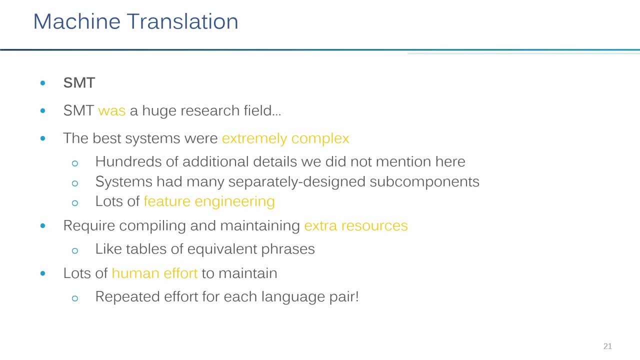 And the best systems were extremely complex And I cannot stress this enough- How many rules they have for very specific cases. Systems had a bunch of different subsystems, A lot of different sub-components, A lot of hand-featured engineering. They use a lot of external dictionaries. 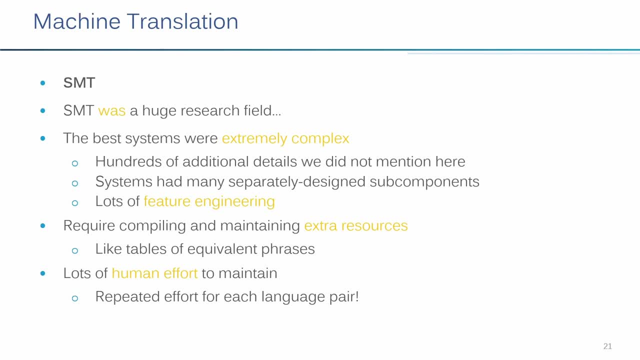 Glaxo databases, A table of equivalent phrases. when things don't translate automatically between them Or you don't have a natural alignment, A lot of human effort to maintain those, And not to mention that you would have to do the same task between quotes for every single language pair that you had. 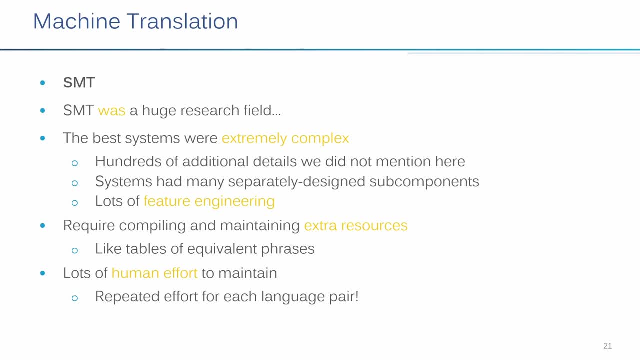 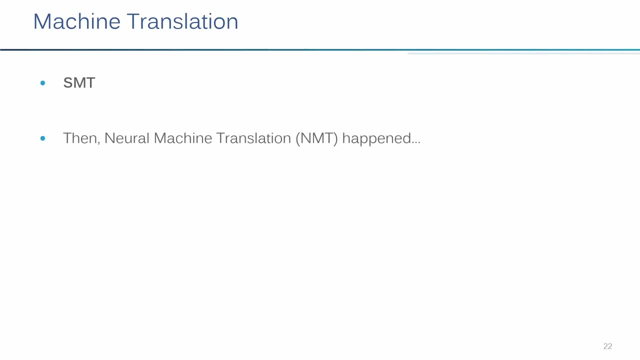 In other words, It would not scale. So what happened? And this really nice anecdote is not from me, But I really like how they portrayed that. So then neural machine translation happened, And to give you an idea how fast and how complicated, 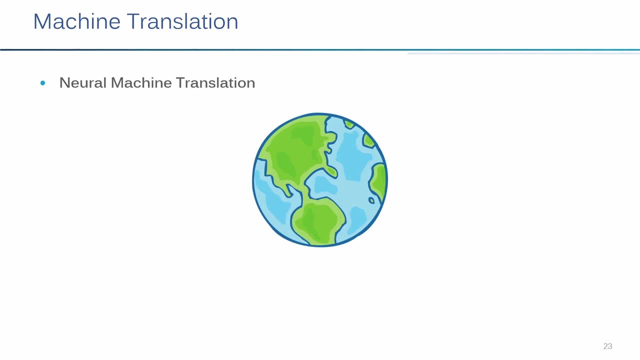 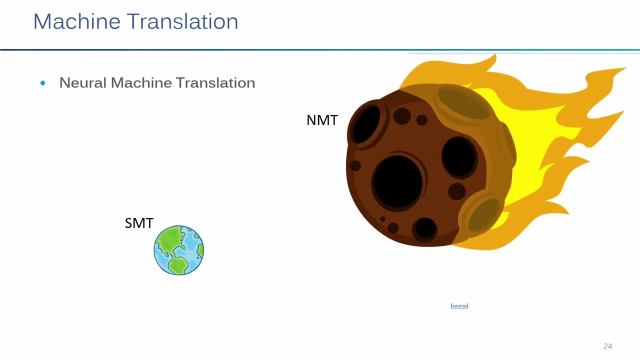 Let's say how fast-paced it was. Imagine that this is a statistical machine translation And this happens. This is neural machine translation. Needless to say, what happened with the field Right? I hope I don't hurt anyone's feeling. 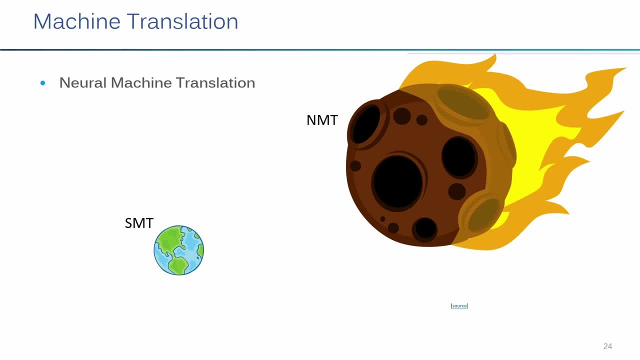 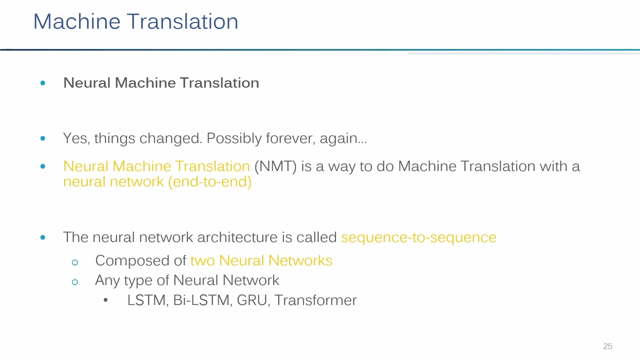 But this pretty much killed statistical machine translation, Like in the space of two years. Again, if you're working for a low-resource language, things are a bit different, But still it killed the field. Anyways, With neural machine translation, the field, it changed again. 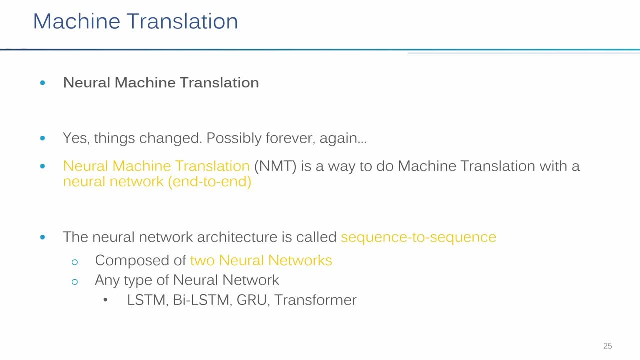 Simply because we found a way, Or we found an architecture to train end-to-end, And this architecture would be able to scale for any kind of language you want, As long as you have data, As long as you have data, Hopefully some parallel data. 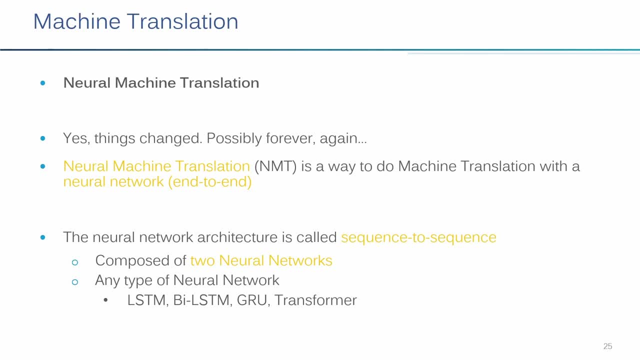 You'll be able to do this And the idea is to use this neural architecture. It's called sequence-to-sequence. People don't actually use vanilla sequence-to-sequence nowadays. They use with attention And later on we use with self-attention. 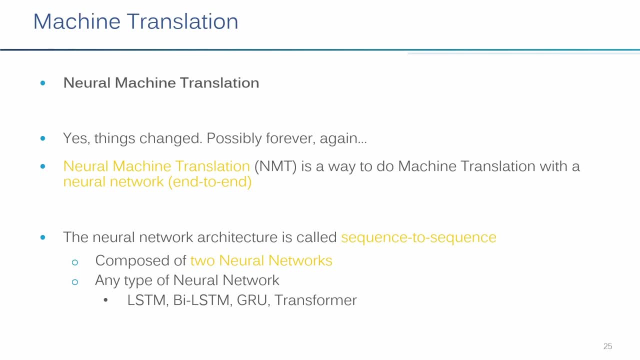 And so on, But the main idea of sequence-to-sequence- How you can look from the second part to the first part in the conditional matter- This is actually quite important for us to understand what comes next- And the idea to use two neural networks. 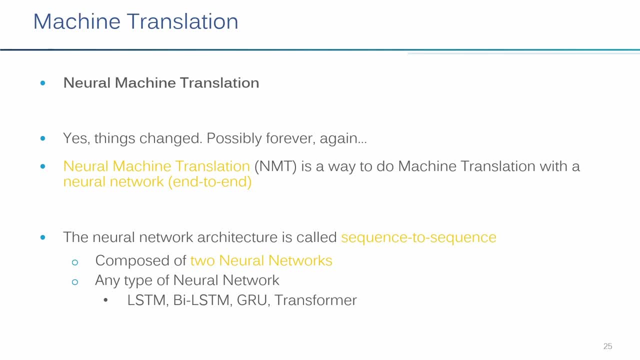 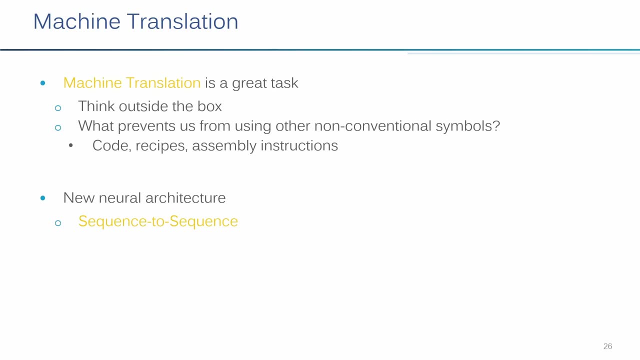 It can be of any type: LSTMs, bi-LSTMs, transformer, GRUs and so on, And I think I mentioned this before. When we talk about machine translation, Don't think just for natural text. Two natural texts. 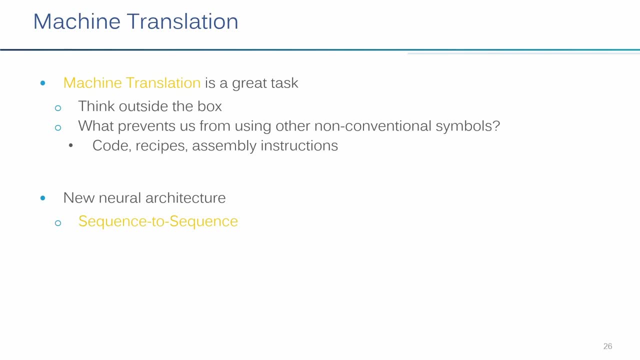 The same, Now that we're moving from this architecture, That we The scenario, This paradigm, That we need to know all the rules from a language. Now, this is really between quotes. This is irrelevant, Because we have enough data to capture those relationships. 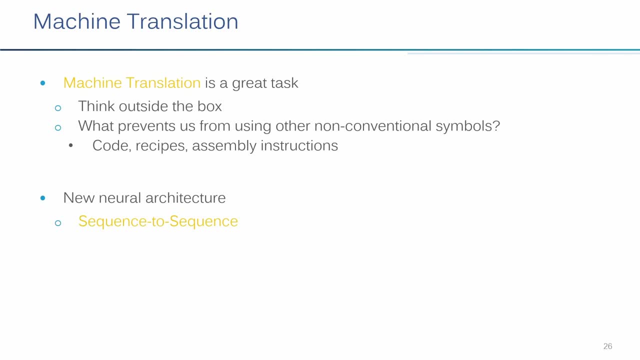 You can apply to any kind of sequence you have From input and output. So if you can correlate this, Even words from the sequence From the same language, Text to text. Let's say you want to summarize a text from a large sequence to a smaller one. 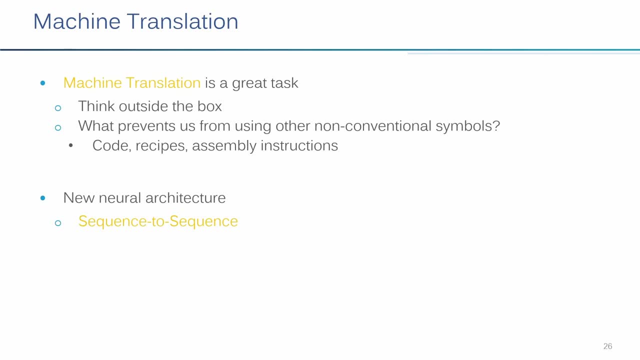 Or you want to transform code into natural text, Or the other way around, Or codes with different kind of languages And so on, Or recipes, And there's literally limitless possibilities with this. And then we'll talk about next class, About sequence to sequence. 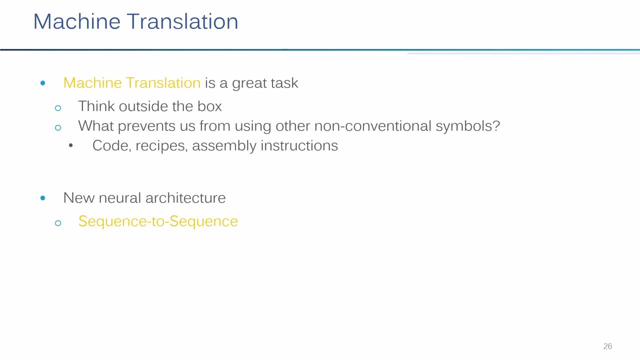 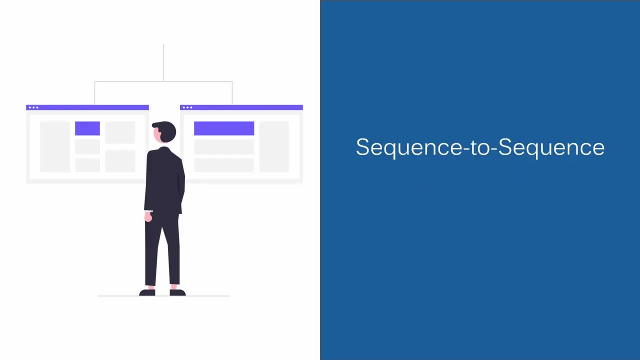 Not next class, This class About sequence to sequence And later on also about attention. So, as we were talking about how we can combine two neural networks to come up with this new architecture That will help us in neural machine translation, 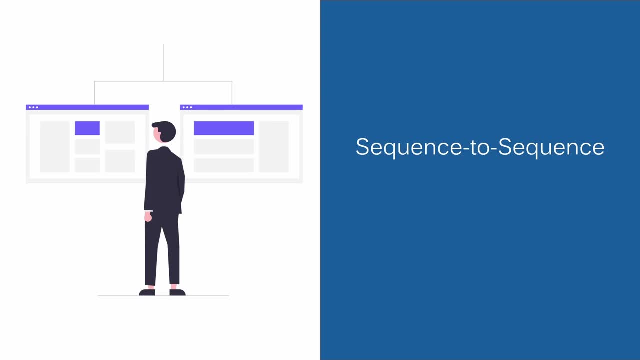 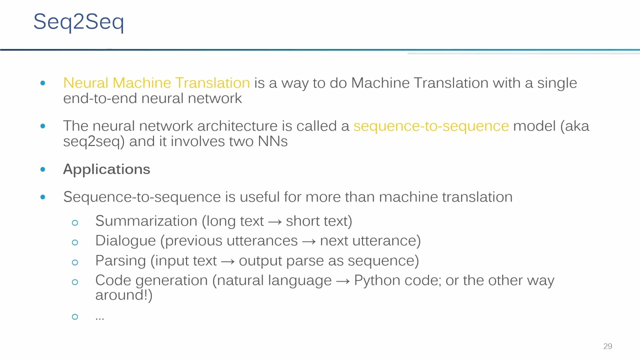 Last week, Last class, We were talking about how statistical machine translation was substituted or overpowered by neural models or neural machine translation. Okay, So neural machine translation is a way to do machine translation with a single end-to-end neural network. So instead of us taking care of all those alignments and handcrafted features that we were talking before, 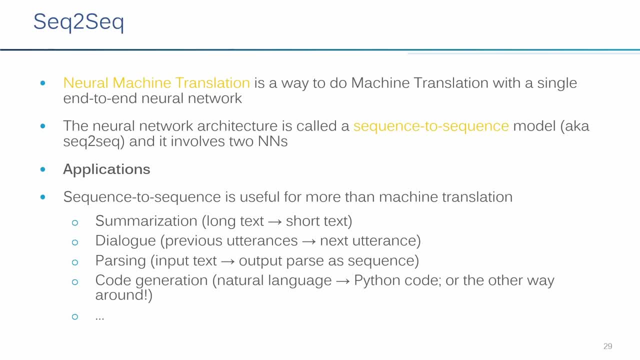 Now we'll simply use two architectures, Two neural networks. It can be for any type. We'll play around with RNNs, But it can be two LSTMs, Two GRUs And so on, And we'll pretty much obtain the same thing that we had before. 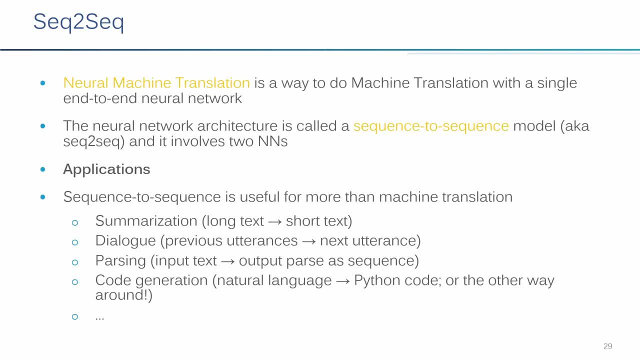 With statistical machine translation, But without getting into details such okay, how can we align these things Or how can we account for how much of the context we have? I mean, we'll do this kind of automatically, So there's no need more for us to do this by hand. 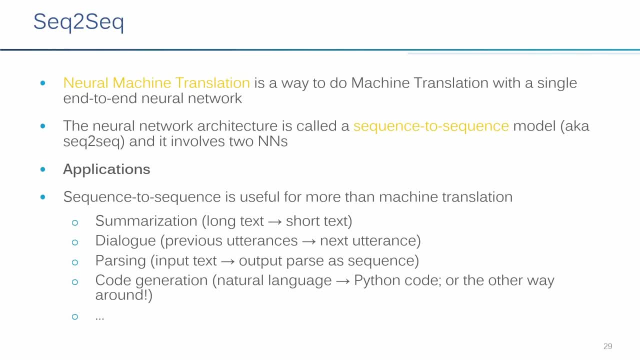 Some applications that we can have for this sequence to sequence- And this is still used a lot today- On a more text-to-text fashion, We can use- And I think we mentioned this before, We can use this For summarization, Such as long text and short text. 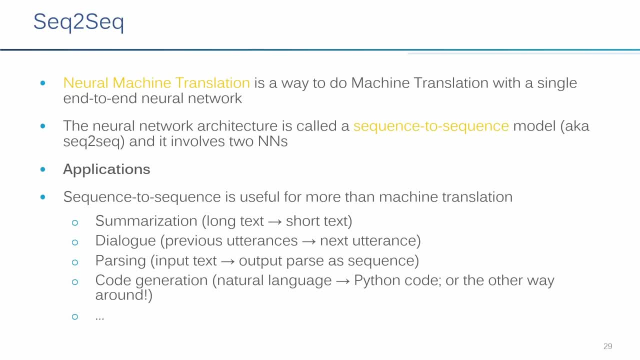 Dialogue: Previous utterances. for the next one, Parsing Code generation, Anything that you can organize- Either your training activity Or pre-training, for that matter- And you can combine this in two sequences Or text-to-text Input and output. 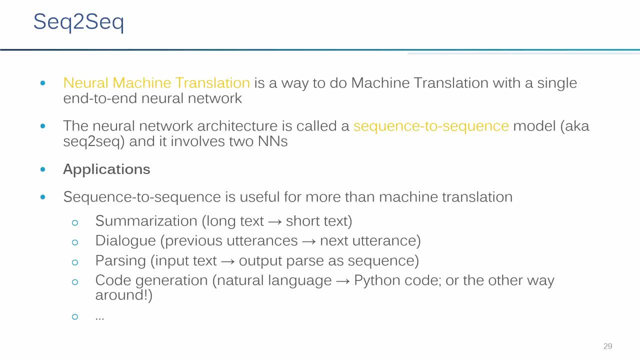 You can use this architecture And it's quite powerful. We will go over the vanilla sequence-to-sequence. Nowadays people don't use that anymore, Simply because they're more powerful architectures, At least in NLP. But we'll take a look in some of them. 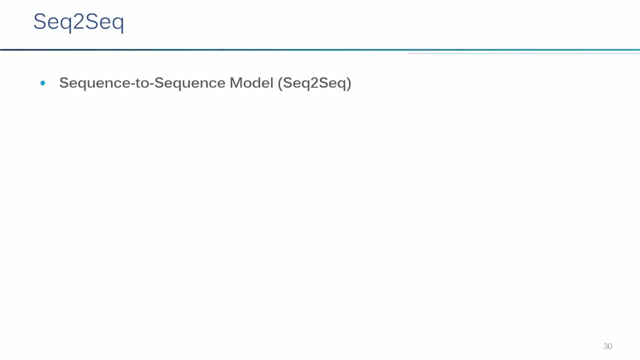 Right. So how the sequence-to-sequence model works, You'll see a lot of similarities And hopefully you'll see how we're simply building up on a new, let's say, block On everything that we learned before with RNN. 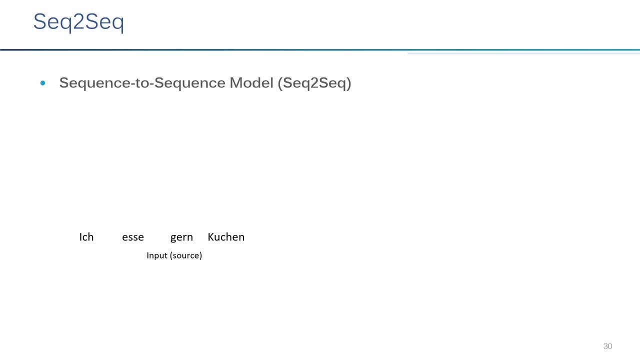 It's pretty much the same thing. So we're going to have an input source And then we're going to code this with whatever embedding that we have, And then, for the first part, we'll have this encoder RNN, And again, we are using here RNN just for the sake of simplicity. 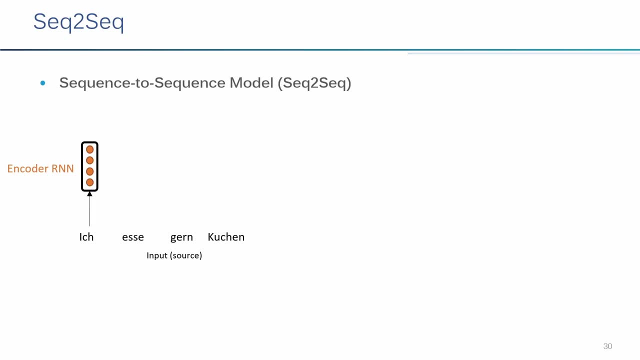 We can use any architecture here, Right? And then the idea is the same way we were doing language modeling before, In which we carry out the hidden states from the previous layer to the next one. We'll do this for the entire sequence in this first part, as we call the encoder. 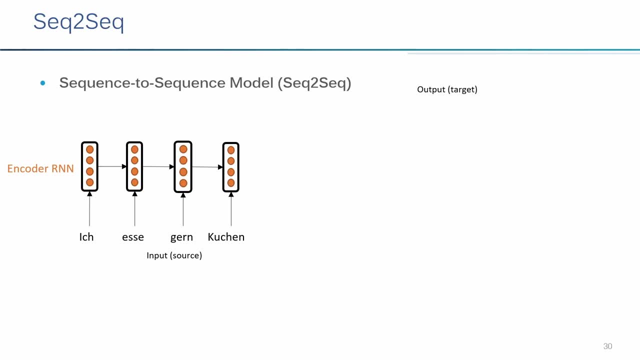 And then the idea is to do this, To transform this input into a target output. So we're going to start decoding or derolling everything that we coded before here into a language model fashion. So instead, if you remember correctly when we were doing language modeling before, 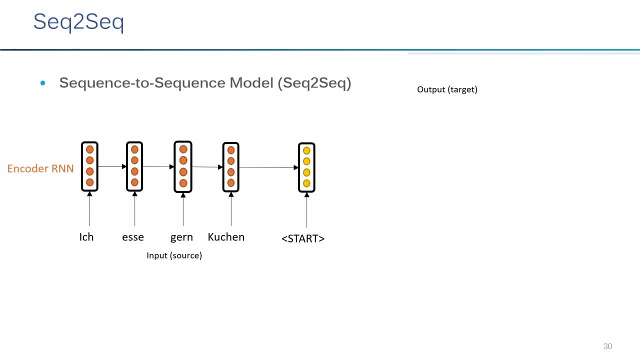 We had an artificial hidden state And which will simply ultra-aggressively predict the next word over and over again. Now, instead of us starting from scratch With some random values, We already encoded- hopefully. enough meaning, enough relationship between words. 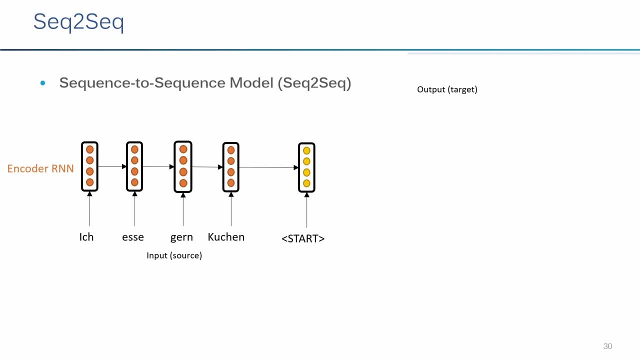 So we don't have to start this from scratch anymore. So our previous hidden state is going to use the entire context that we have for whatever input source that we had before And the idea is after. I have this first part here on the left coded: 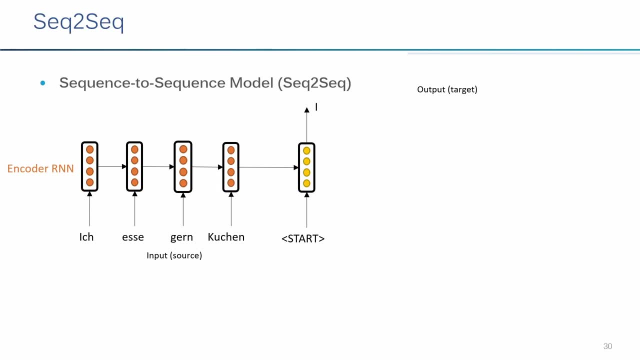 I'm going to start predicting the next words, the same fashion as we had it before, And this part right here, It's simply using another recurring neural network. So from our previous state, Which is the entire sequence, right here, We have a start which will pretty much 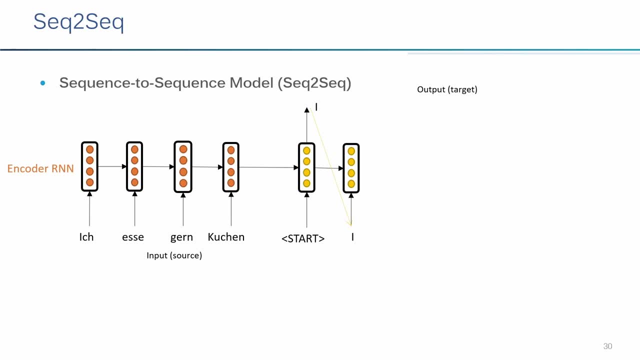 And this idea of using a special token to say, Okay, this is where things start, Or where this end, and mark, Let's say, the break between sentence and so on. This is still used today a lot for the Transformers architecture. When we see BERT. 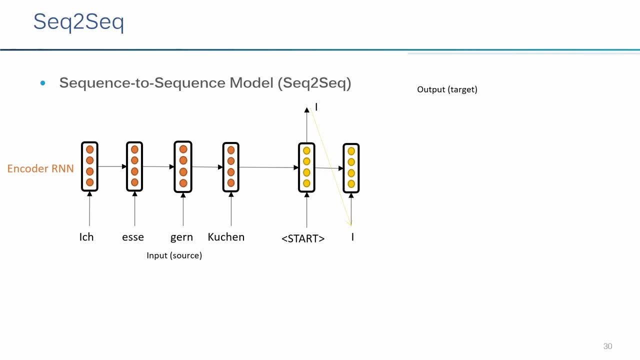 We see that they still use special tokens to do this When you want tag positional encoding for more fancy architectures and so on. So this idea to use a signal to give a hint where things should start or where things end- They're still used today. 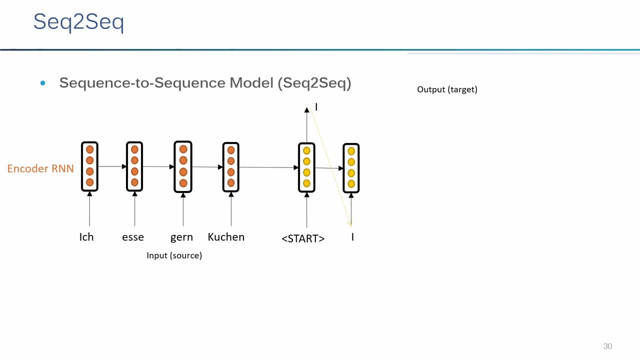 Which is pretty cool, But in any case. And then, after we have our initial state right here, We start decoding or predicting the next word all over again. So in the first start here I know that the first word is I. Hopefully with training you get into this. 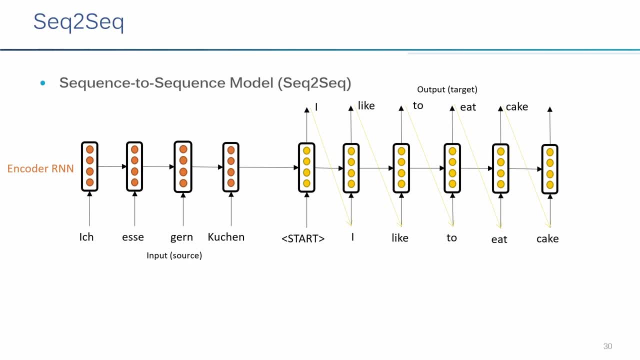 Although this here is test time, So after I generated I, I provide I as my input And also all the hidden states that I had before, For the next one is like: So I put like as an input here And again the previous states from this neural network here on the right, 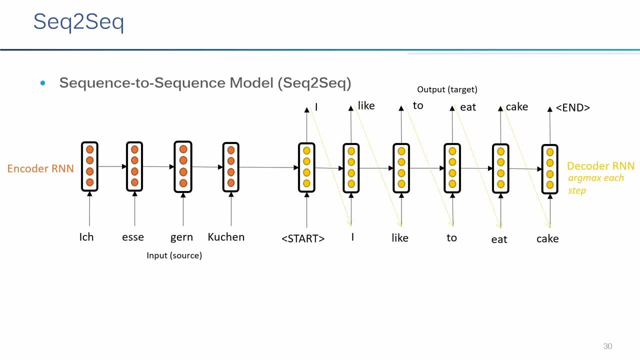 That we call a decoder, And all the previous states that were in the hidden states from our encoder And then on each step on our decoder, Until we hit a specific end point, A specific end token. We'll simply take what is the word with the max probability. 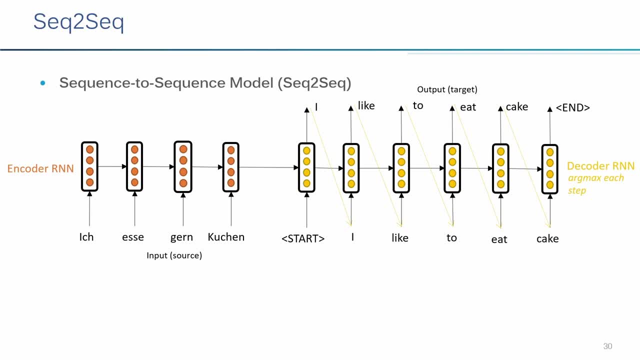 Or the highest probability, That makes sense to be here as the new sequence. All right, So the encoder RNN, Or this part here on the left, Produces an encoding for off the source sentence from our input. Hopefully you can already see some concerns about this architecture. 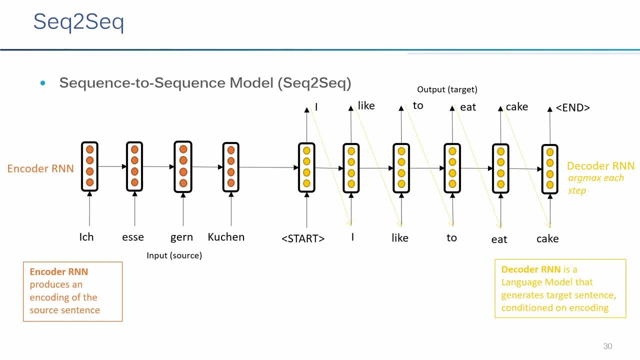 Imagine that we have to encode everything here And our decoder is nothing more than a language model That generates the target sentence or the word by word. Given all this context that we have here, All right, Yep, The very last state from our encoder encodes the source sentence as a whole. 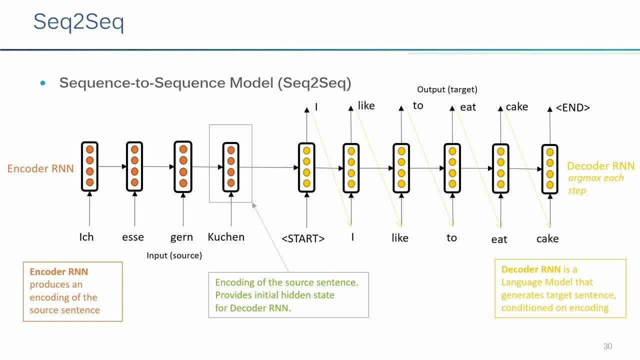 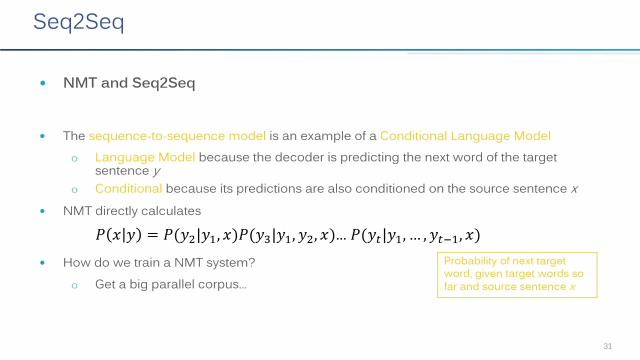 So hopefully, when we get to the last state in our encoder, We'll be able to capture, Let's say, a good representation for the sentence to use as a context In our decoder. All right, Our sequence to sequence model is an example of conditional language model. 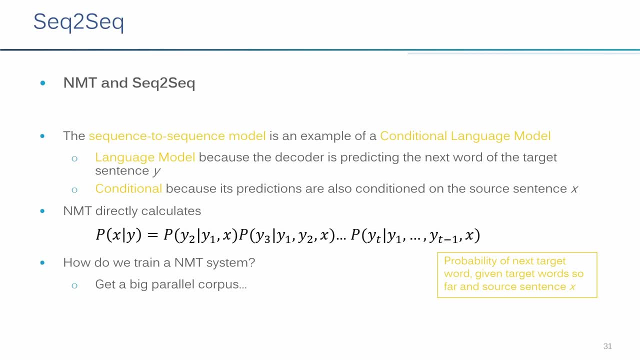 Why The language model? because our decoder is not doing anything new. It's simply predicting the next word over and over again, According to the previous state. So it's 101 language modeling, But it is conditional because its predictions are also conditioned to. 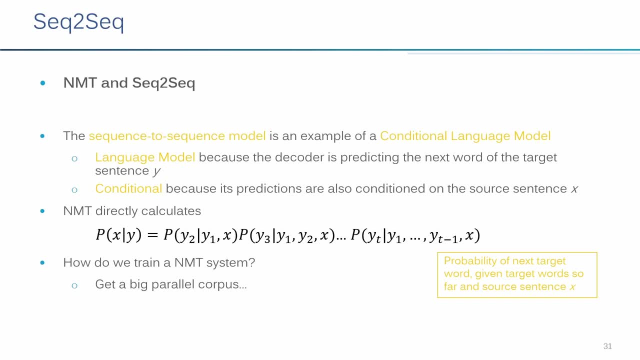 On the source sentence x. So before we had the probability of x, given y, Our target and source sentence, We wouldn't have this second parameter here, This x. So for every new word that we have in our decoder, For our y here, 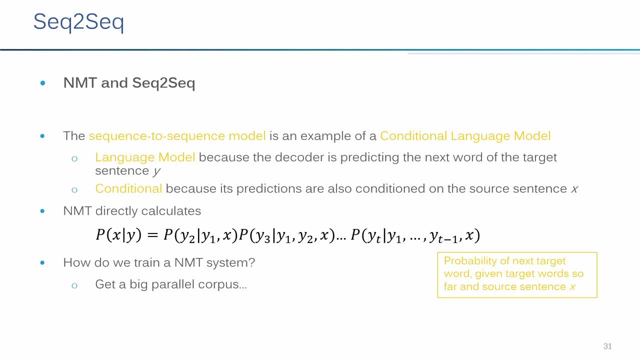 You see that we are carrying out all the encoding from our encoder part, So represented by this x, And A natural question is, of course, How do we train the system? As before, You need a parallel corpus, Somehow aligned with input sequences. 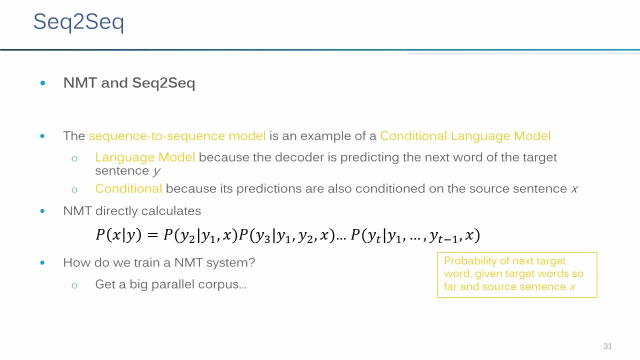 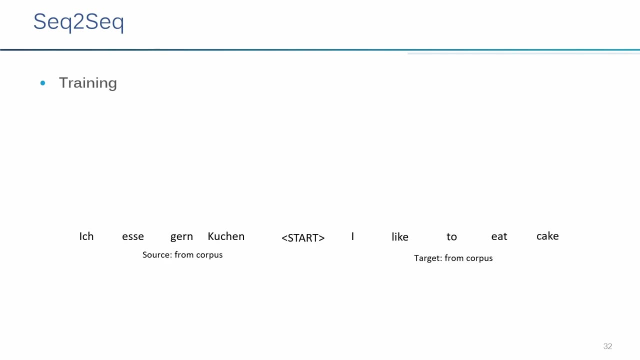 Input sentences and output sentences. Right, And I think that's it for this guy. So, and how training it works for us. So we still have the two sequences, But the difference is We don't need to actually use the predictions that we have. 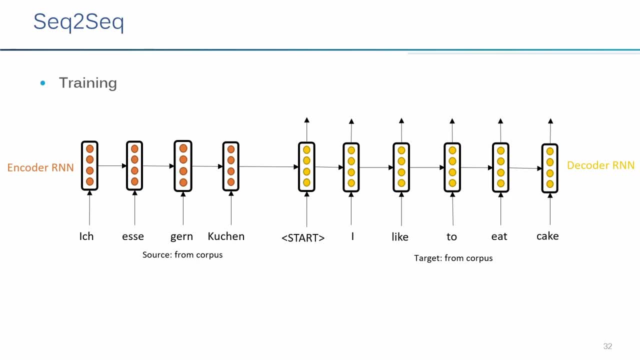 Other than just calculating our loss. We can simply use the actual words When we are trying to predict what the decoder should output for us. Pretty much the same way when we were doing language models with RNN. So instead of using the actual prediction, 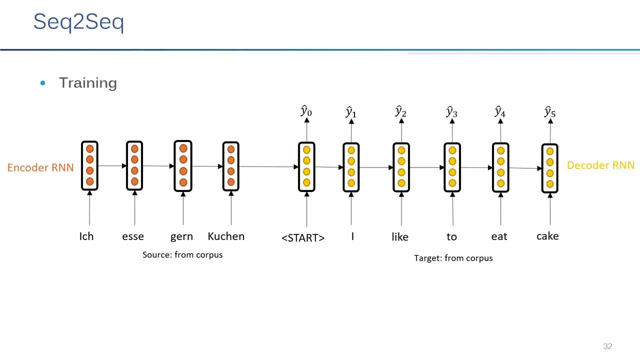 It could be some gibberish. We use that to calculate, Okay, how far away we are from this target sentence That we are trying to predict, But at training time We actually use The actual word that we have aligned from our corpus. 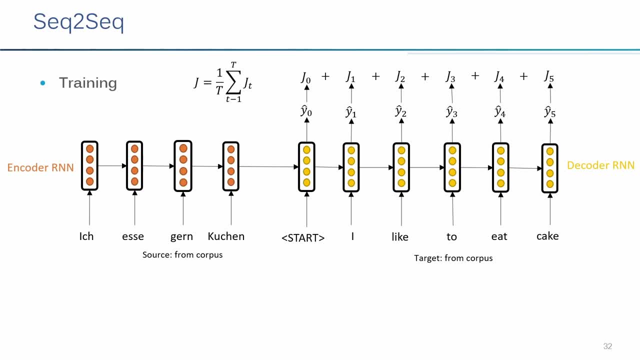 The source sentence And also the target sentence, Right. The cool thing is, Even though we are using two sequences for this, Or two RNNs, The training, The optimization for this Is done from end to end. So we back prop from. 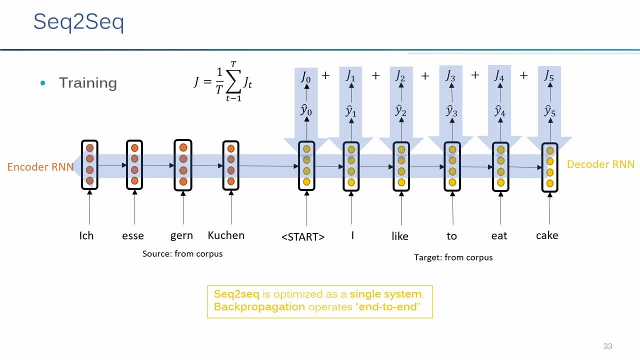 Let's say the very last state from our encoder Decoder, sorry, To the very first state in our encoder. So the back propagation operates end to end, So you don't have to take care. Okay, I will do optimization for one part. 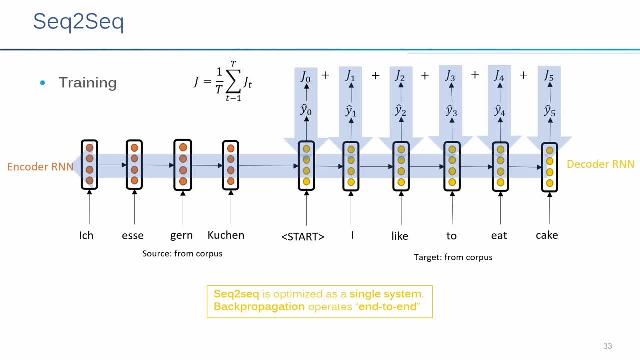 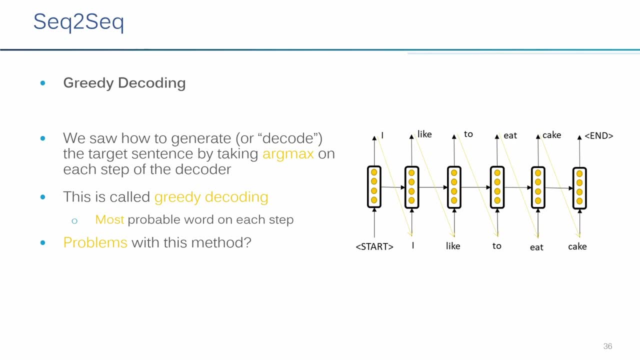 And then I do another one for the second part. This is simply done automatically for you. And then How do we guarantee That, given whatever representation that we have for our encoder, I make sure not to produce some trash, Because this is a bit hard to control. 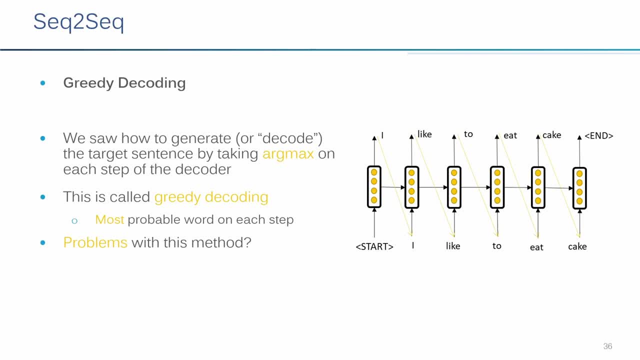 Right One approach for doing this language model on the decoder part Is simply use greeting Decoding In a way that we simply optimize for the max probability on the next word Given whatever input that we have. So we don't care about. 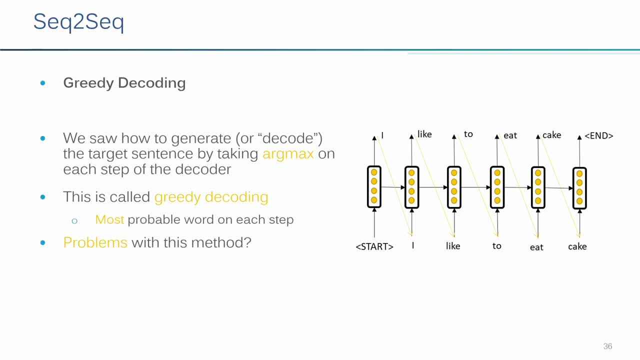 Let's say, If it's not the top one word with the highest probability, We simply discard everything And take that first one And let's go with that. Can you see some problems In going greedy When you're simply predicting the next word? 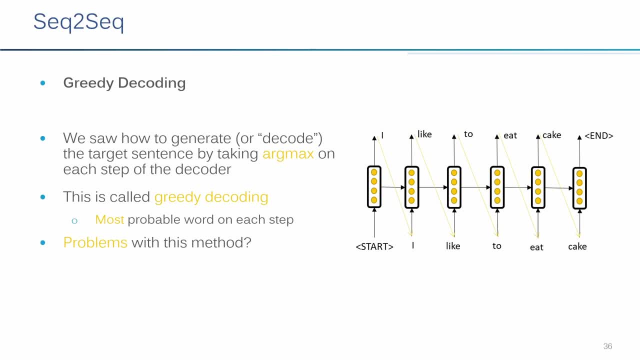 Based on whatever max probability you have, Or I mean Not just with this, With this whole, Let's say, Linear paradigm. Can you see a problem with this? Well, To begin with, There is no guarantee That the word with the highest probability 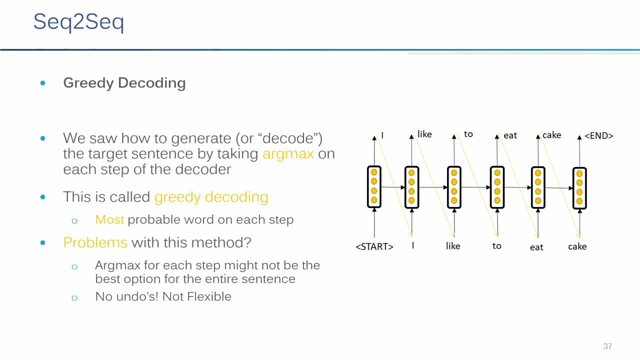 Will provide you the sentence that makes most sense. It can happen, Of course, But it's not necessarily the case, Especially for specific Corpus and context. Also, No undo. So this architecture here Is not that flexible In a way that. 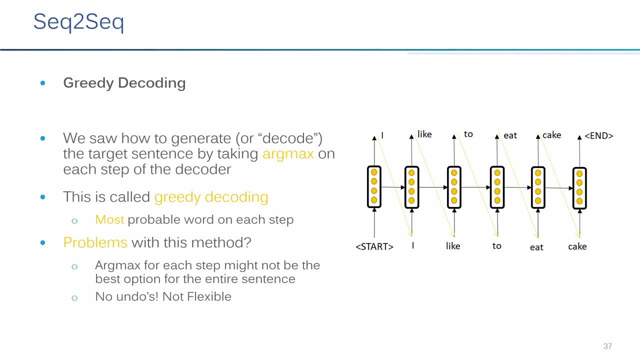 You cannot choose To go back After you generate the next word. So Once you generate, Let's say Here From the start It's I, And then from I, You, You predicted Like, And so on. 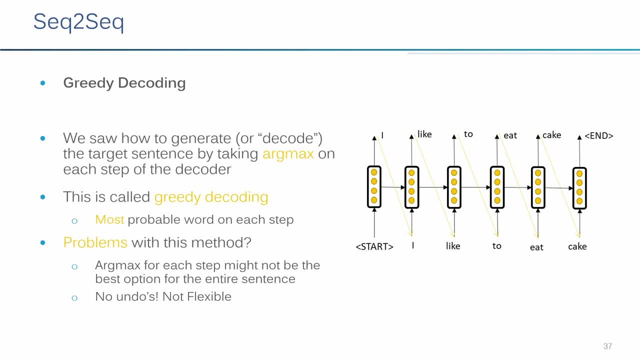 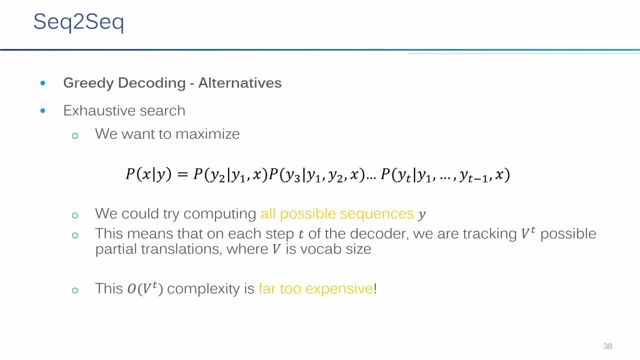 You cannot go back Because in the end was I like to eat computers. So, yeah, Too bad, That's what you get now, So it's a bit hard To control for that, All right, So An alternative For this. 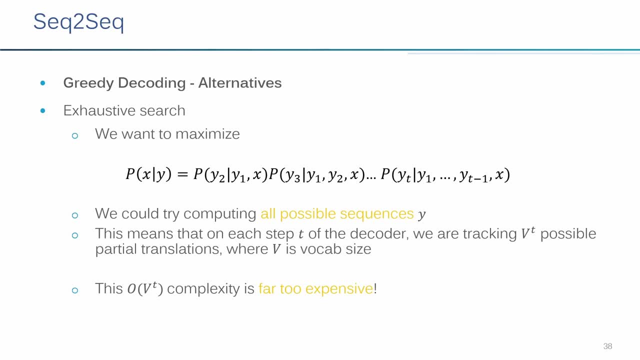 We can do Exhaustive search In a way That we maximize The probability For the entire sequence Given At every new word. We simply Exhaustive look For the entire sequence, Considering The entire vocabulary. Needless to say, 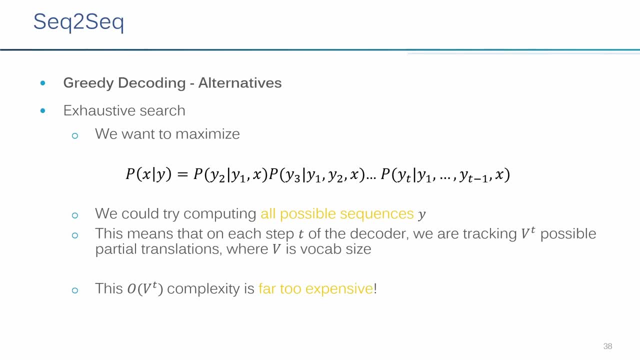 This is not very efficient, Simply because On Each step, We have Simply Too many possibilities. We pretty much have The entire vocabulary, And This is Actually. It doesn't work for us. It's simply Too many possibilities. 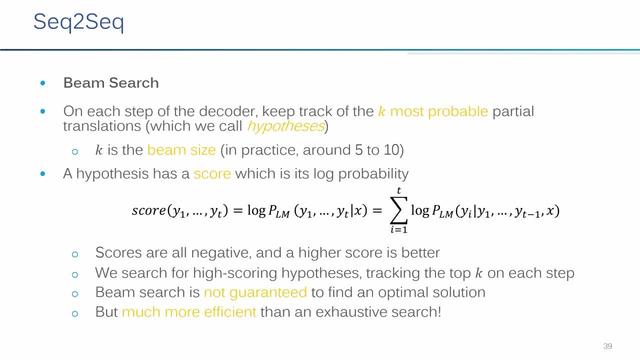 All right, But Hold on. There is a way to Take care of this. One Way of doing this Is using Bing search, And What is Essentially Is a fancy name To say We're going to start. 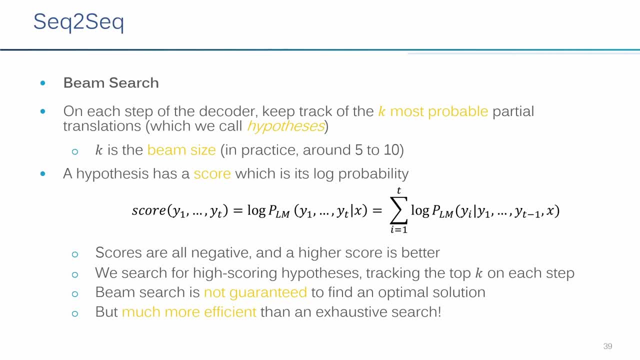 A couple of Possible Sentences: The one with the highest scores. Given The score, How many Sentences We Will Initialize Or We're going to do The entire sequence Is up to us. This is a free parameter. 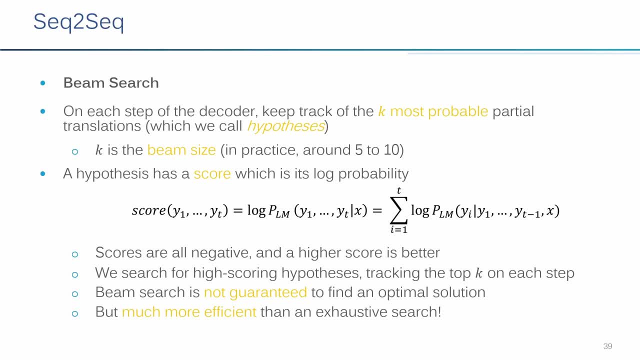 So You can control One, Two, Three, Four, Five, Ten. It depends on How much Computing Power You have, Of course. In practice, This number Is around Five, So We're going to 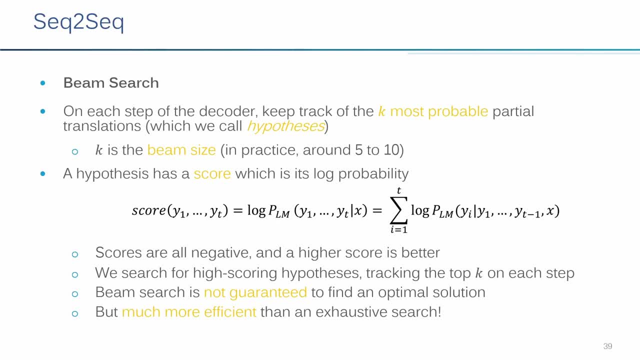 Keep Only Those With The highest Scores. Is This guarantee For us The best sentence Or the best Result? Not By A long Shot, But It Is Better Than Doing. 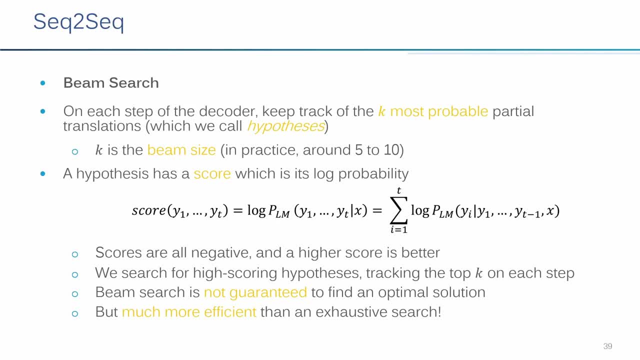 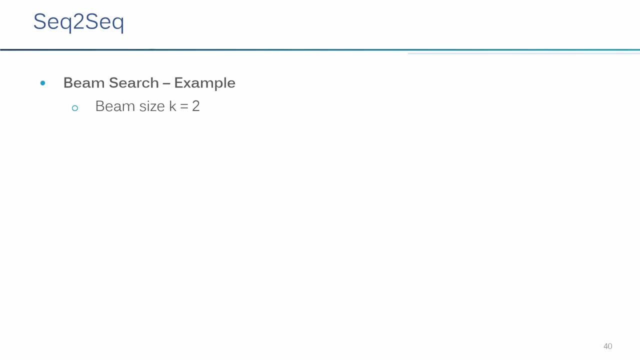 Greeting And Also I cannot Stress. It's Really Interesting, But We'll Get There. So How Being Search Work And, By The Way, This Is Also. 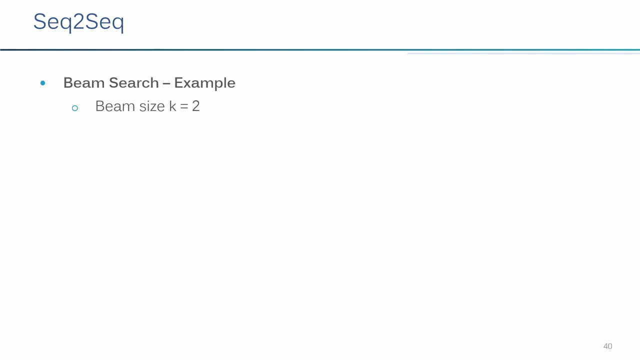 Using Chat Dialogue Systems. Text Summarization Is Not Exclusive To Work, So We Have Our Start Sequence Right Here. By The Way, Are You Seeing? 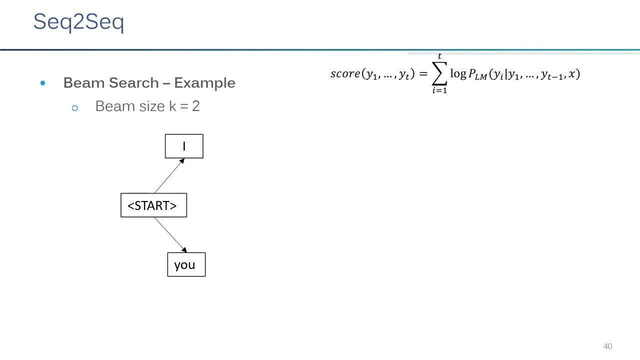 This Shadow. Okay, There's A Fly Here. Okay, Sorry For That. So In The In The, The Highest Score After We Do This On Each. 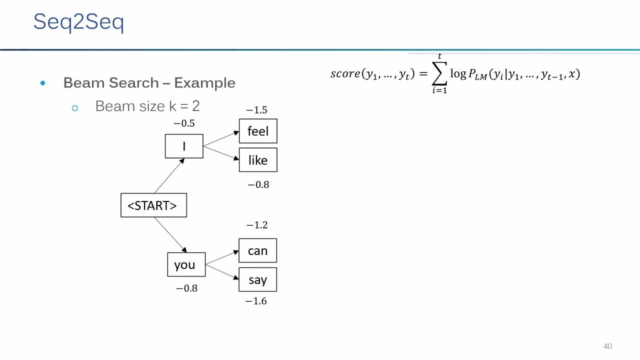 Of This News Steps. We Also Expand The With A Big Size Of Two. So From I Like Two. So In This Case, Right Here We. 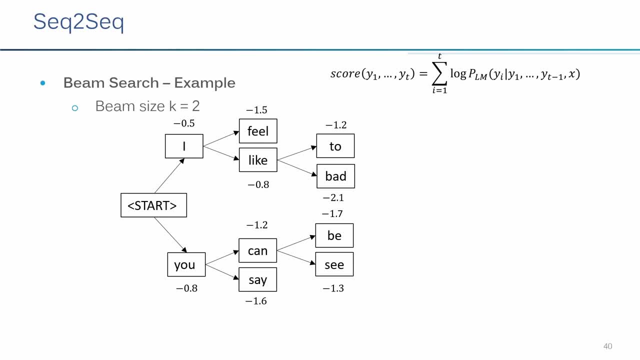 Continue From. I Like Two, So We Continue On Zero Point Eight, And Then Here We Continue With One Point Minus Until We Finish Our 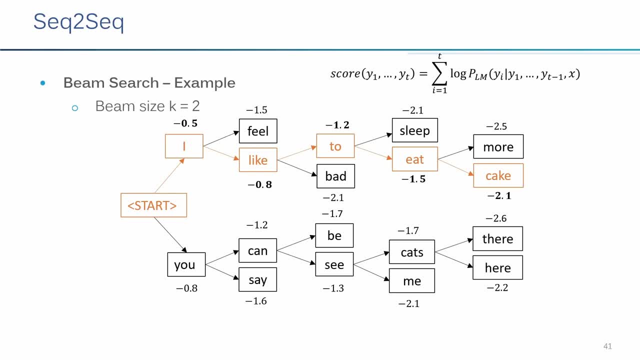 Sequence. Well, I Think I Put This In The Next Slide, But We Continue The Sequence Or The Case Sequence Until We Finish, And How We. 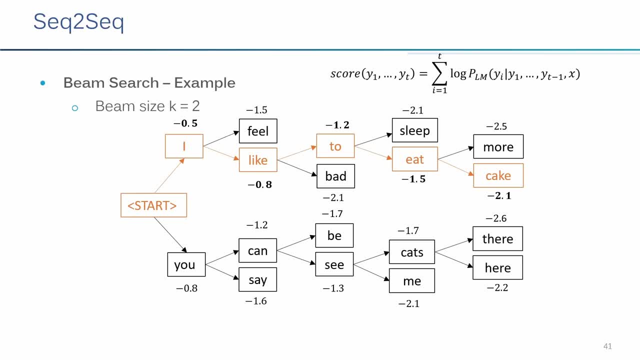 Continue With One Point, One, One, Two, Three, Four, Five, Four, Five, Six, Seven, Eight, Nine, Ten, Twelve, Thirteen, Fifteen, Thirteen, Fifteen, Twelve, Thirteen. 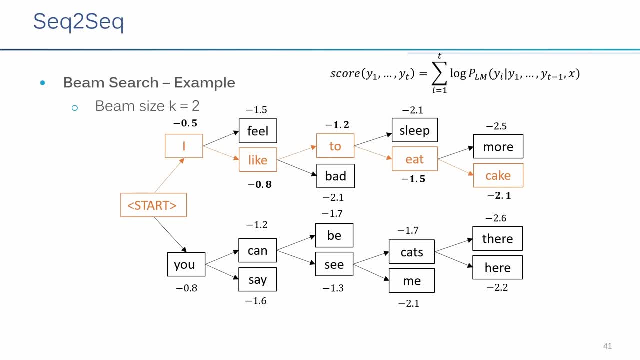 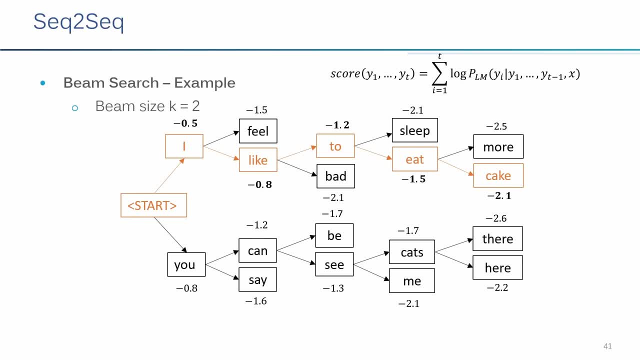 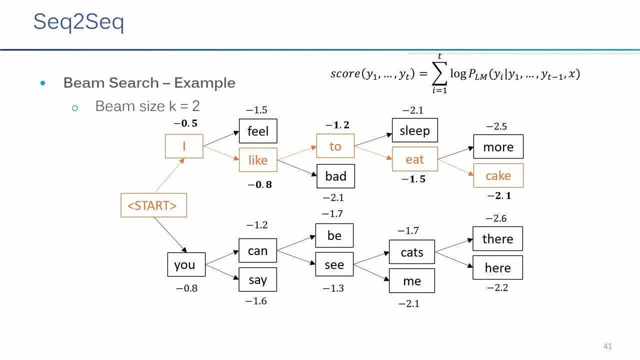 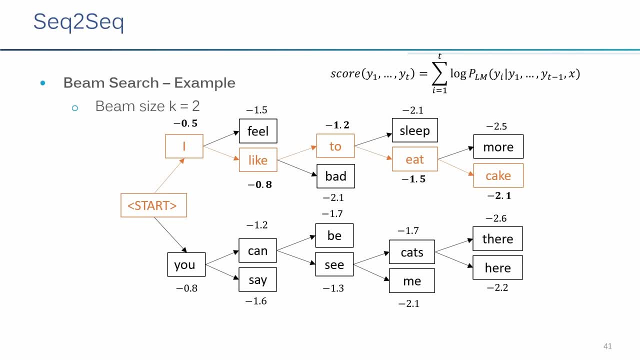 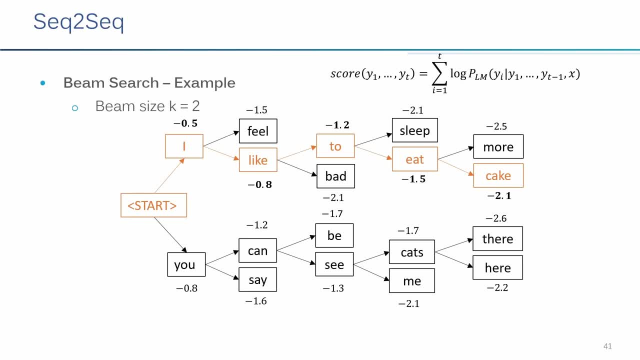 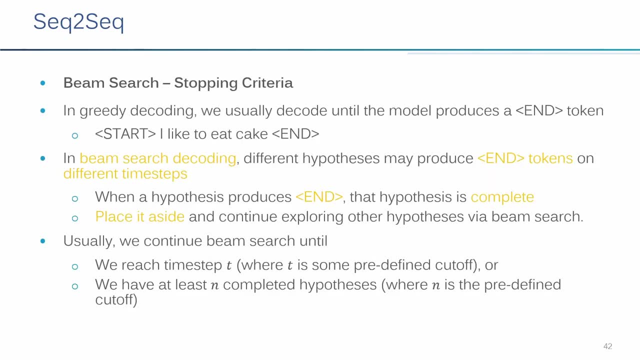 I can provide this for the reading. I'll provide this on the lectures about transforms, I guess, but be that as it may. so in when we stop developing our sequence ingredient coding, we usually decode until the model produces the end token. so, as we saw, we have a star token, the sentence and the. 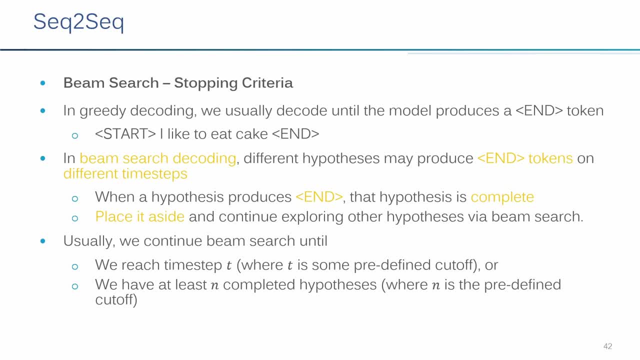 end token and in being searched the coding different hypothesis, they may produce this end token depending on the sequence that you have. so either you go further- a longer sequence- or shorter sequence. you can have your end token there at whatever point. when this happens, simply you put the sentence that was completed side and you continue the other hypothesis, and there's ways. 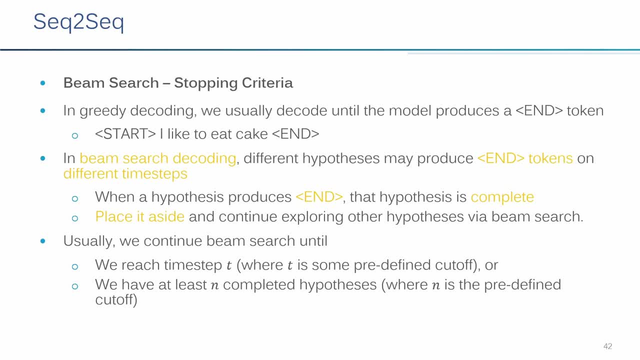 to, let's say, to build on top of this, you can start with a specific number of sequence, and if one of them already gets the end token, you simply start a new one that was, let's say, the top three or four. that was previously not developed. there's improvements. 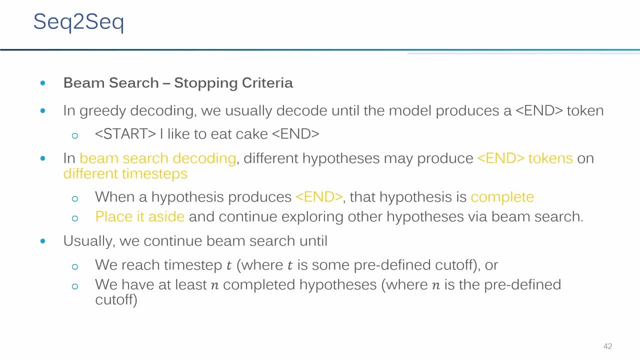 and improvements on this architecture, right. but usually what happened is you do this for specific timestamps, so you have a cutoff. I don't know after 10, 20 or whatever number steps you develop, after that you cut. whatever you sequence that you have, or if you have at least a specific number of complete hypothesis. let's say: 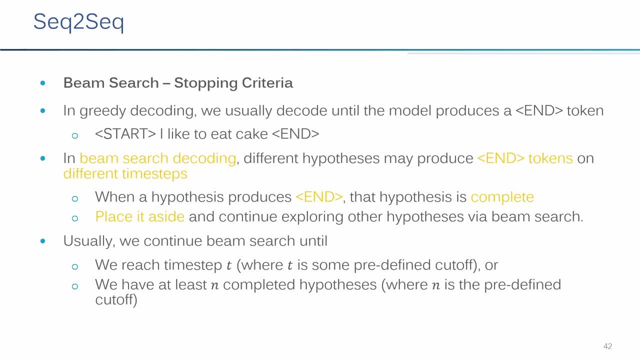 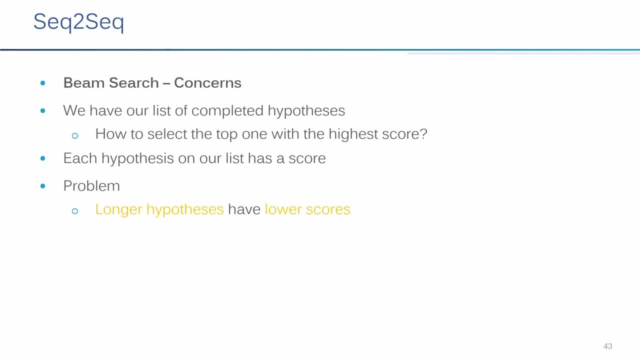 you keep developing them until you reach the end of two or three and that's it. all the others you drop, okay, uh, some concerns. uh, when we were developing the sequence on being searched, you probably saw that we want to maximize the score that we had there. the thing is, the longer your 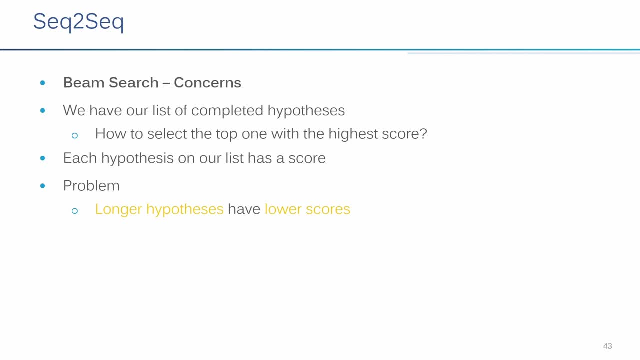 score gets, the lower your score gets, simply because your account for all the probabilities in all the states. so how you cope with that? you simply normalize that, uh, in a way that you don't have to penalize longer sequence because of the score if you take into account their length. otherwise, 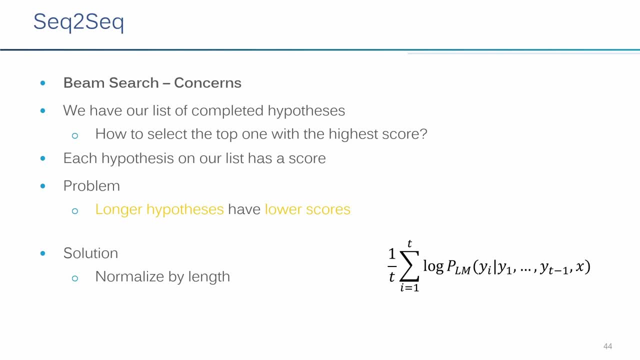 all the, let's say uh, all the, the short sentence or the short sequence, they will have a higher score and you will always have short sequence being developed. yep, usually, uh, when we're trying to decode this part, you have a source sentence, so in this case, you. 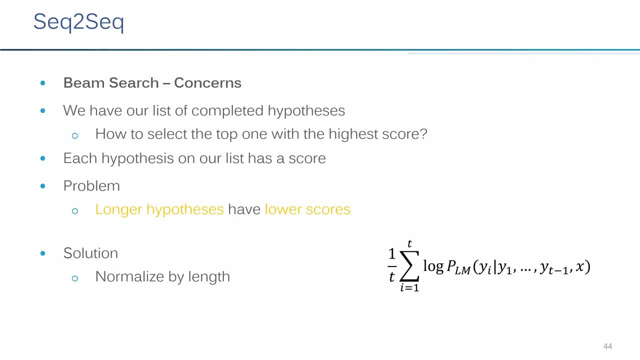 have a training set that, uh, you know exactly when that sentence is. until it's going to be developed. you have the end token. training time. on test time, probably you have to develop. there's a specific number of steps, or until you act, until you reach a specific threshold on the score function. but if you 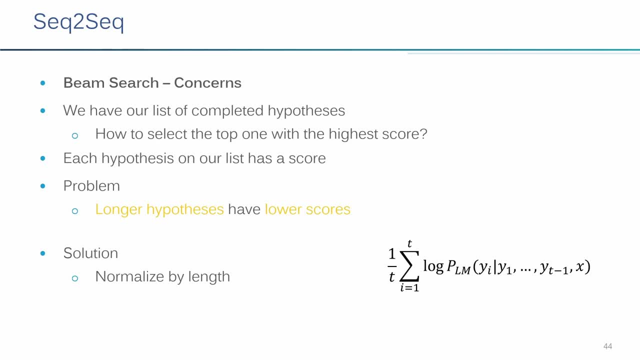 don't have any stopping criteria. this will develop endlessly, of course. uh, all of them. they have some cut off. at some point you have to stop it, but that's pretty much how it is okay. uh, this is a good example how these models: if you continue those sentence endlessly, you see these models. 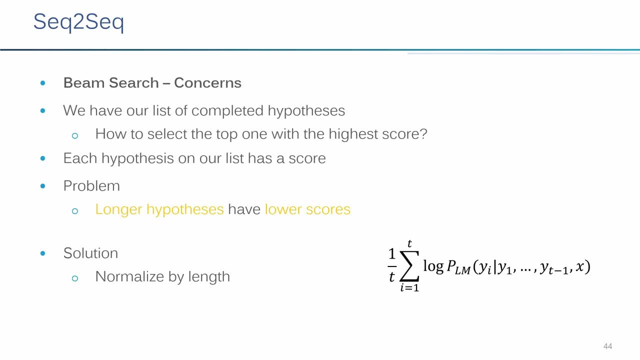 usually hallucinating, like in the beginning, when you have short sentence, say hey, that's, it makes a lot of sense. and then after a while it starts providing some gibberish. and it doesn't make sense because the longer the sequence- specifically talking about vanilla- sequence to sequence- the longer your sequence is, you are relying way more that in the very end in 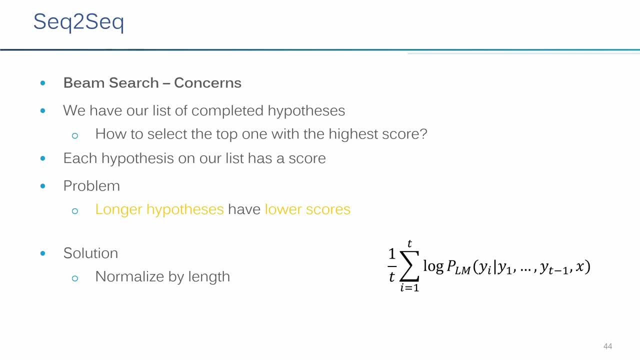 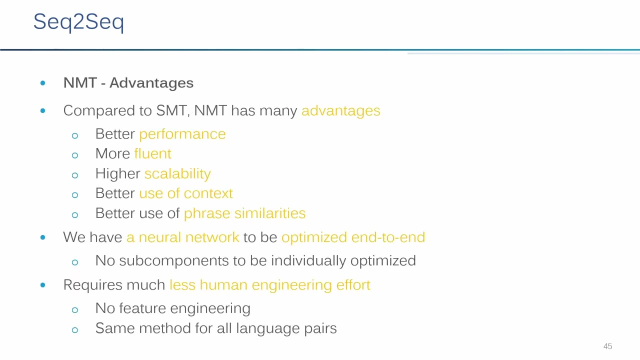 your encoder, you have that sentence as long as it gets. it will be represented in the last date, so there is no guarantee that every single step before it can be used to produce a same sentence towards the end. but it's not trivial to do this, it's a bit annoying. okay, some advantages with neural machine translation compared. 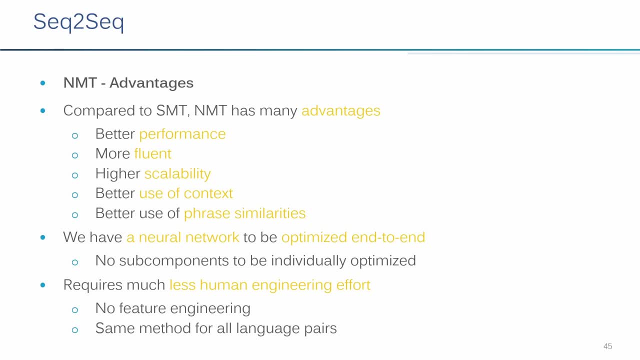 to statistical one. we do have a lot of advantages. first of all, we have better performance. the output that we have is more fluent. needless to say, you can scale a lot, simply because now you don't need to develop, let's say, specific rules for every pair language that you have. if you have enough data that you can align. 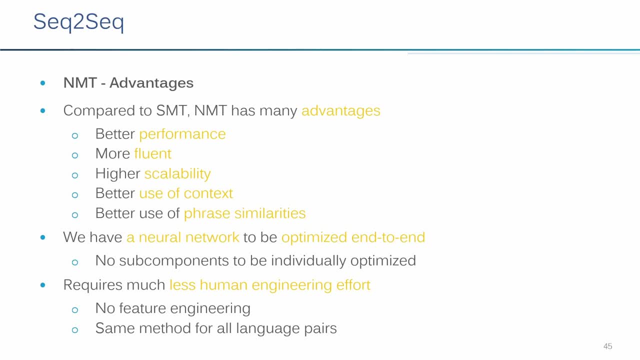 between input and output. you can explore that and scale as many language as you have data, all right. better use of context: that is debatable, but in theory you're making a smart user for context because you encode the entire input sequence as in context for everything that you were developing before, when 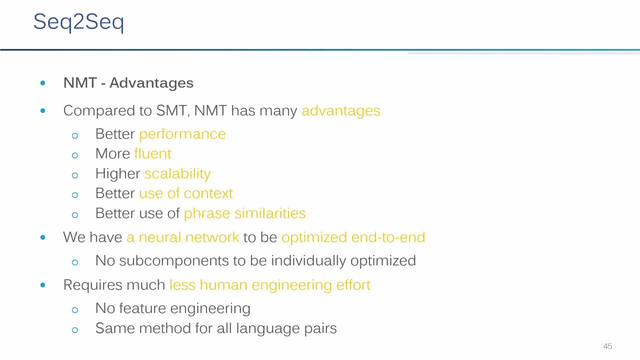 you were decoding, but if that's best one. that's debatable, we'll talk about this in a minute. better use of phrase, similarities seen because you have this aligned pair. you don't know exactly how each word will be aligned back and forth, but at least on the sentence level you know that one input is related with that. 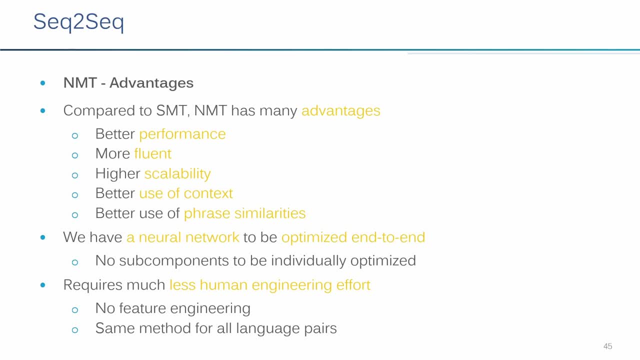 output regardless. we have a neural network to be optimized end-to-end, so there is no individual sub components that we have to take care. I don't know there's specific dish, although you can include this in your example. you can include external knowledge through lexical databases, dictionaries, wiki data and so on, but in this version, vanilla one, you don't have. 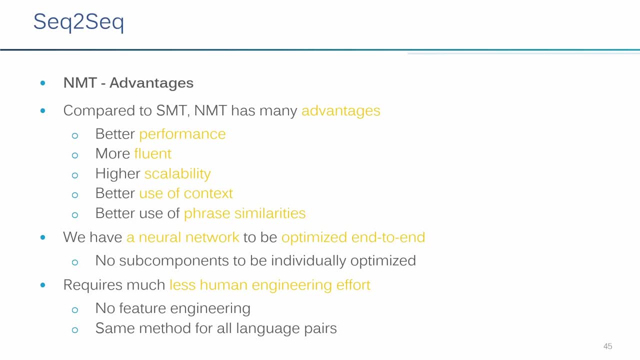 to worry about this. individual components also. needless to say, it require way less human engineering effort, and this is one of the breakthroughs. like you, don't have to take care now with every single detail that we had before with statistical machine translation, and in fact, this is most. 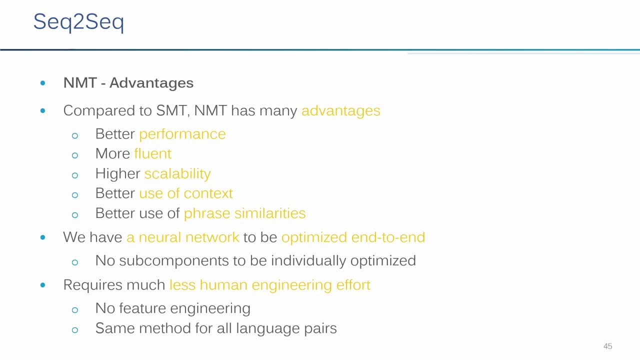 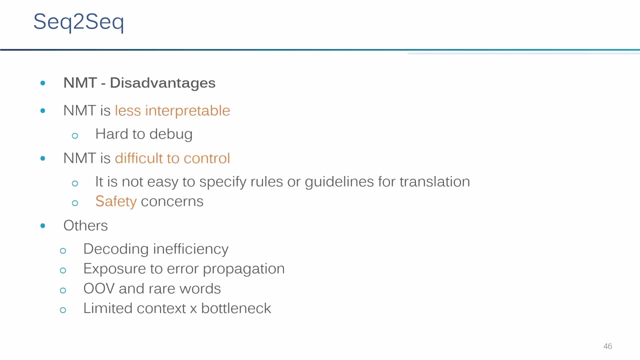 true, for I would say, most architectures that we see here, in the beginning you would see that neural architectures, they wouldn't perform that well, but they allow you to scale and this is a really a game changer from now on. but don't think this is just flowers. there are huge problems with every, every single architecture. I 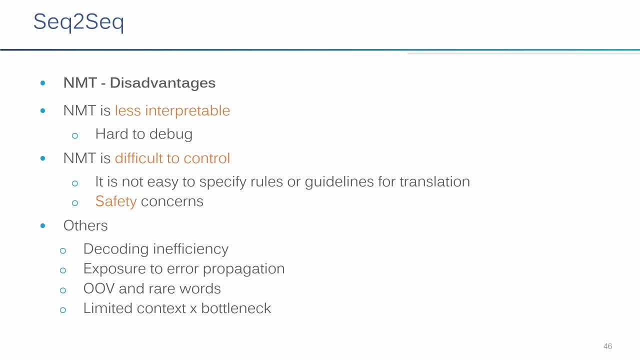 would try to provide. okay, it's good because of that and it's also is bad because of that. in case we miss, let me know and I can include that for sure. but some disadvantage with neural machine translation, is it? it is less interpretable simply because we don't know exactly, for example, what those 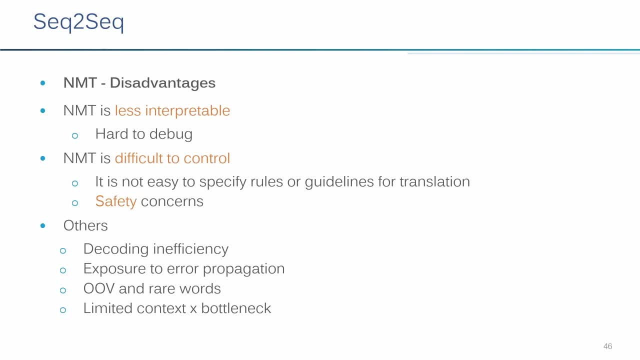 weights. they mean there's no way for you to pinpoint that. yes, this Matrix, and with this weight distribution here, is taking care of whatever nuance that we have in between those two sentences and also is difficult to control in a way that you cannot easily specify rules or guidelines or how. 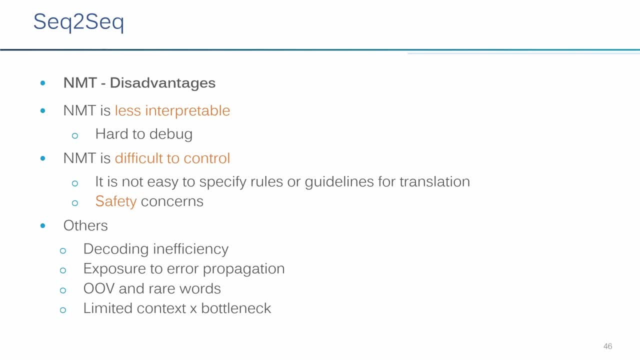 you're translating, how far you're translating what you have to include, what not to include? indians, cultural aspects, you cannot do this. also, safety concerns. I mean there is, uh, it's not easy for you to prevent a model simply to output something. let's say it's a touchy subject. 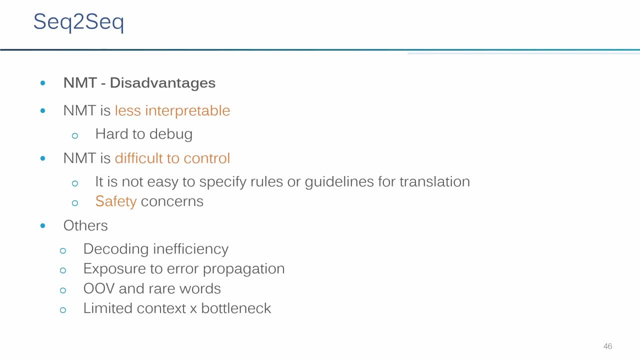 For example- and this actually is still a problem- for up-to-date Ultra-aggressive models that produce any text- what happened in practice is, Instead of taking care on the inner components, of taking probabilities of words- Let's say that might represent some stereotypes or something They do a most of post processing after they generate a sequence- if that sequence, for whatever reason, should not be used, 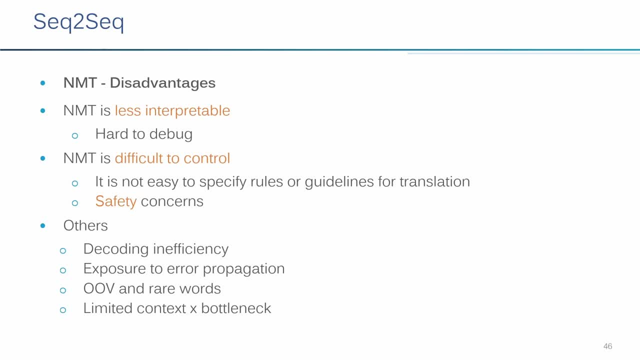 They cut that or they eliminate or they provide a message. I don't know if you ever play with the very first versions of this large language models. They would output some really nasty things. of Course, this is related with related with the data They were ingesting. of course, 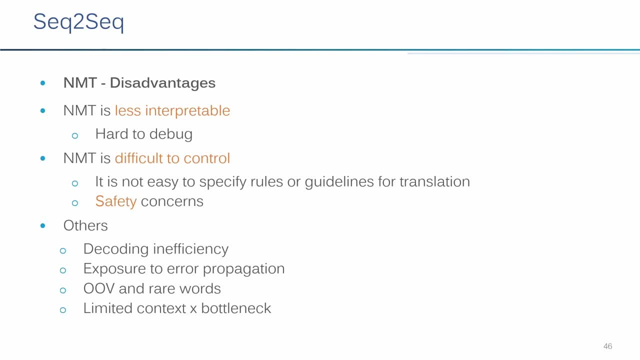 But now either those models, they're kept, or simply you have some comments as disclaimer, say: hey, the output might Might contain whatever words and so on. but we'll see more About this when we talk about text generation in the very last class, when you talk about ethics and bias. 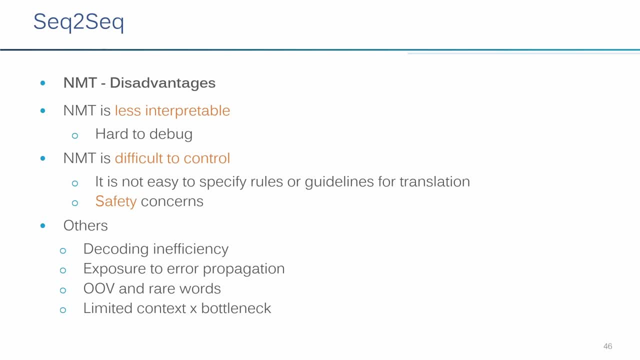 In this lecture right. Also, there are other problems. The decoding part is a bit inefficient. if You have some error or whatever because of the training data that you have and the prediction is not good, You will propagate that out of out of Words, out of the vocabulary. 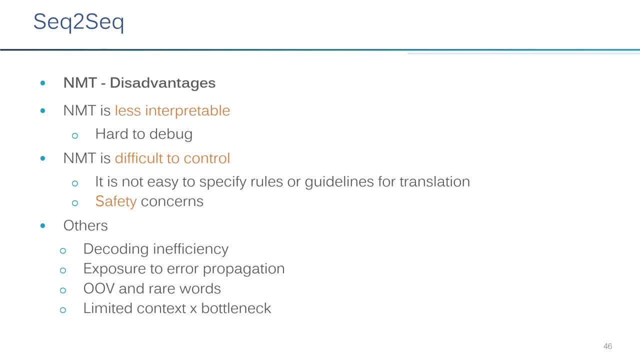 And rare words are also a problem, because if you don't have enough data to represent Specific words, it's going to be really hard to predict them. And of course, we have a limited context and the bottleneck, which we'll talk in a minute right. 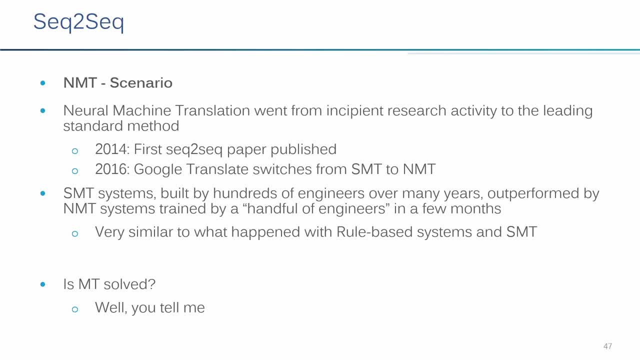 Just to give you an idea. So new machine translation went from a very incipient research activity To the leading standard method. So, if you remember, the very first paper when we talked about this was 2014. the very first paper was published and then 2016, Google switched from statistical machine translator 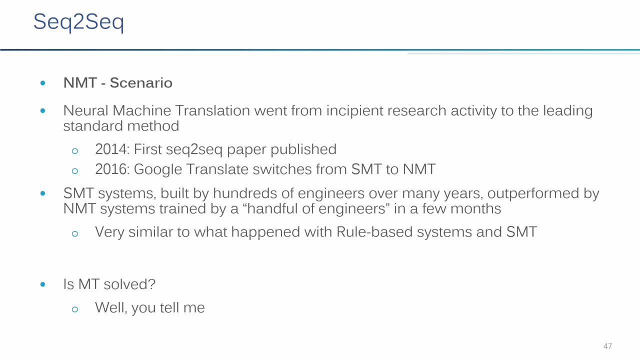 statistical machine translation to neural machine translation. And if you take that into account, this sentence right here is a little bit drastic in my opinion, because it says: statistically statistical machine translation systems built by hundreds of engineers over many years, outperformed by neural machine systems trained by a 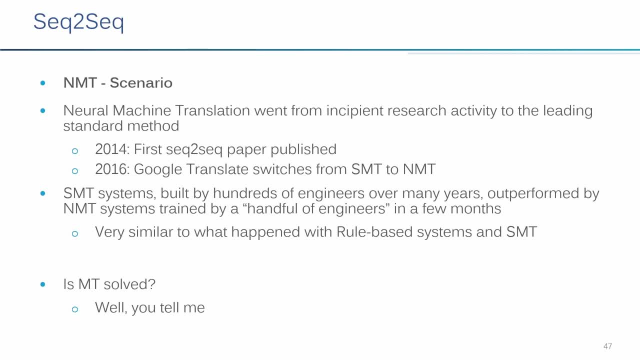 handful of engineers in a few months. It was not a handful of engineers. There's a lot of people working on this. It's definitely an understatement, But for sure it was less people than statistical machine translation. And if you might think, oh yeah, like these people how they didn't. 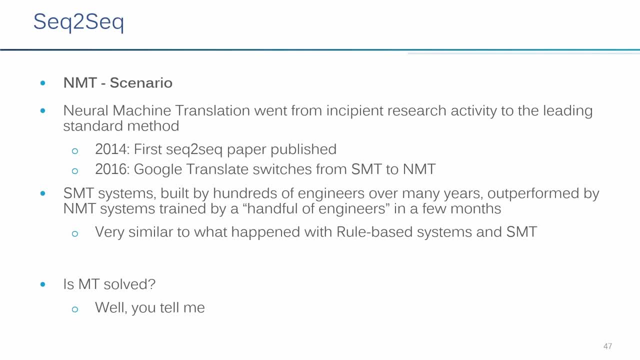 see that coming. this actually happened also before. That's not the first time, And this is happening right now again. So remember the rule-based systems. They suffered the same paradigm shift in which they thought those rules would account for every possible scenario, And then statistical machine translation came and said: ha, if you have enough data. 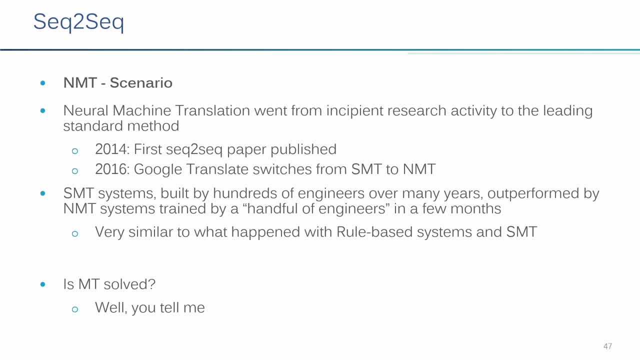 and if you have these features right here, you have discovered- And yeah, the rule-based systems. they pretty much died. Of course, there are still work being done with rule-based systems, But now they're more part of an ensemble, of a complex system. They don't hold by themselves. 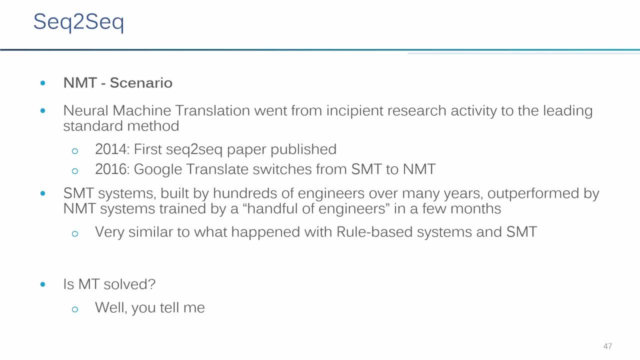 that well anymore And how this is happening today. if you take a look by these large language models, it's pretty much happening the same thing, right? You don't see like vanilla sequence to sequence being used in this kind of architecture anymore. But you might think, OK, now that we have 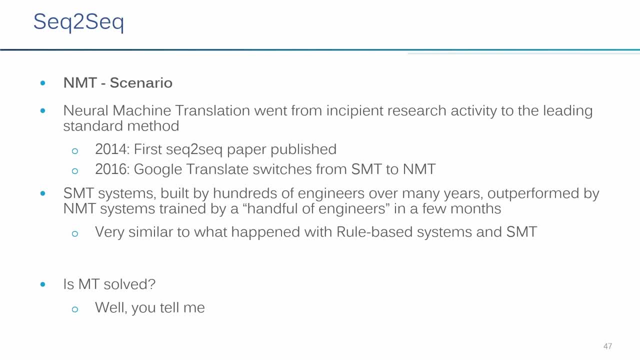 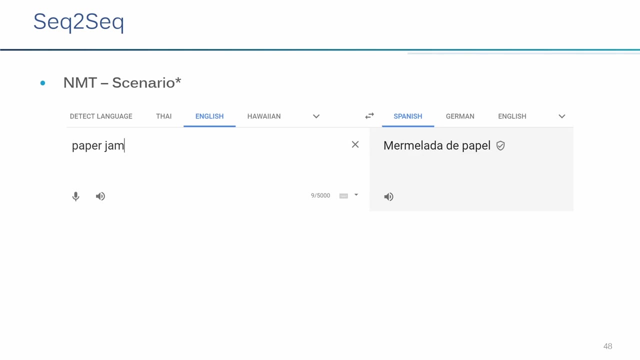 a context. we have encoder decoder. I can calculate how faithful my decoder is. consider my context, And I think is machine translation solved? Well, not exactly, And I wish I could reproduce all of this In 2019 and 20,. I was still able to reproduce a bunch of them, but not anymore. 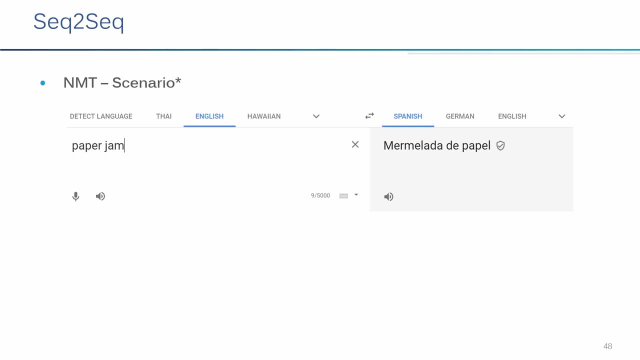 So before in the early days, from near machine translation, if you're using Google- and this actually happened- if you say paper jam, it would be translated to Spanish as marmelada de papel, Which it's pretty much. you want to translate this here and this is what you're getting. 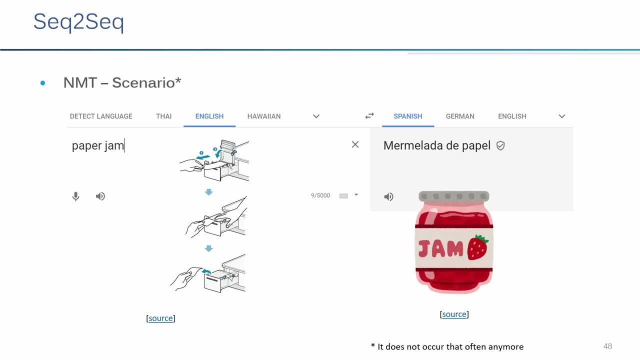 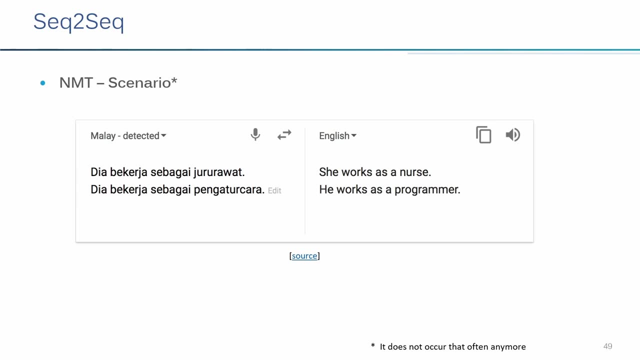 from Spanish And this actually happened. It was really fun to play with that in the beginning. Also, we would embed some biases and stereotypes in machine translation. We talk about this again later on, But depending, let's say, in Malay. I don't talk Malay, but I want to believe. 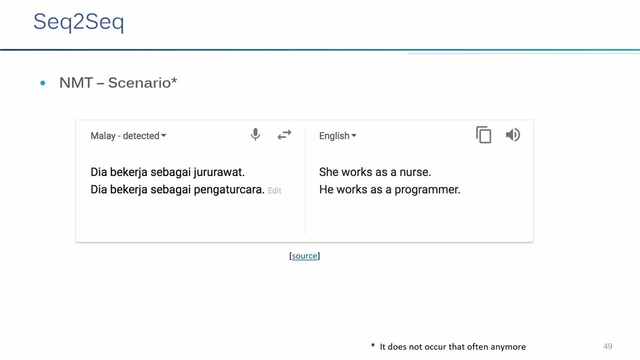 that's the pronoun, how they use it. Depending on the profession or the noun that we use to categorize a specific pronoun, you would have that different. So, for example, if you say this word here is a nurse and this here is a programmer, they would be translated. 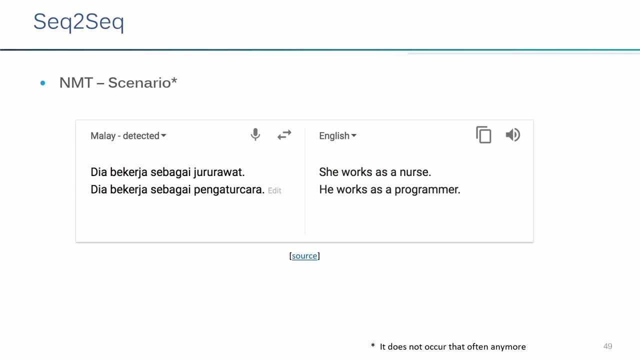 differently. So if you have nurse it would be translated to she, and if you have programmer it would be translated to he. So that was a huge problem in the beginning. But again, this here. it doesn't happen that much anymore. The same thing for Finnish: If you have words. 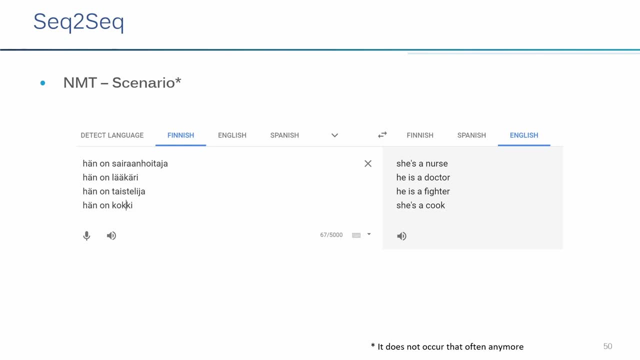 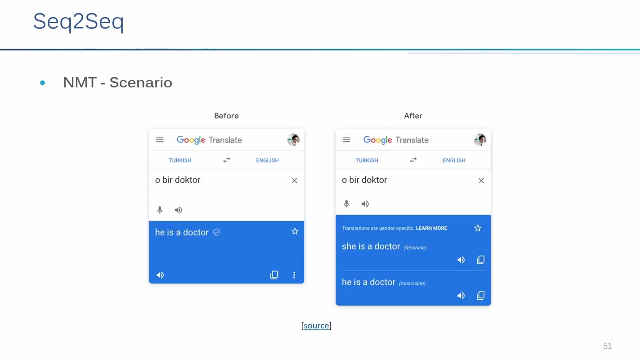 such as nurse and cook, you would have the pronoun translated to she and if you have doctor, fighter, king, leader and all this kind of stuff, it would be he associated. What happened now, at least for most of the, let's say, the examples that we looked on. 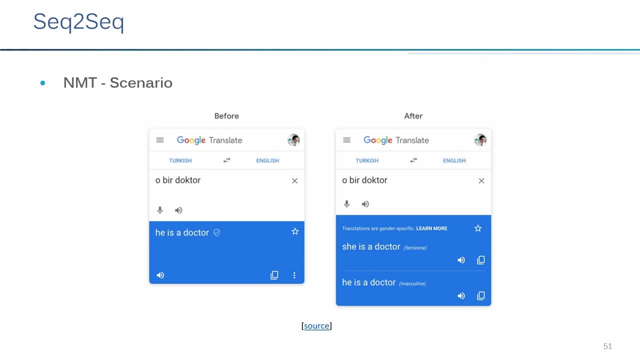 if you have something, if you have a translation that's gender, grammatically gender specific, they would offer to you to say, hey, this language right here that you're trying to translate is gender specific. so you have these two options that they have coded there and with reinforcement learning. 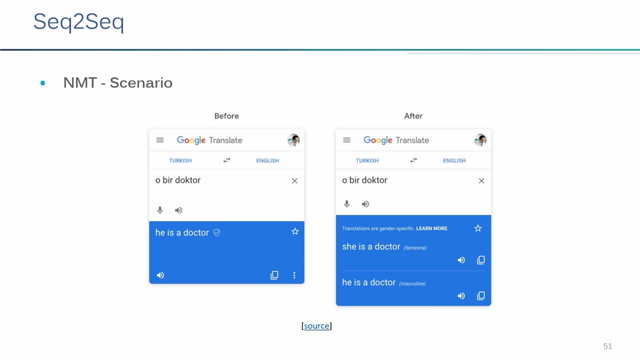 you can help the model get better and better, But then they leave this up to you to choose which kind of translation you want. Maybe also you saw that in a different form, in a way that you provide the sentence, the input sentence, and the output. it provides two. 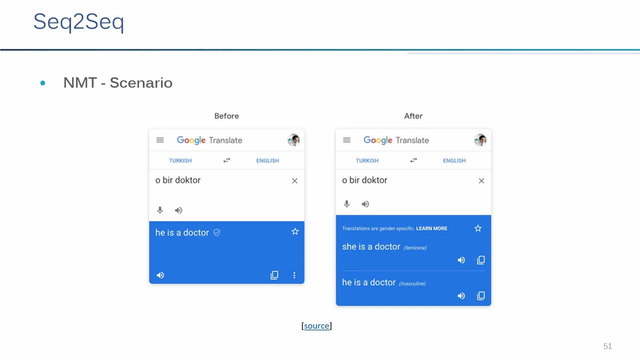 three or even four translations and say, hey, pick a translation that's gender specific and you can give criança. you can say you want to translate that it's the same for both, but yours has a differentскиp. It's the sample version you're looking for And 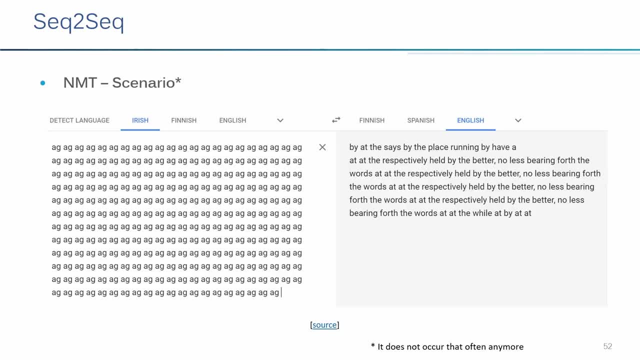 for it to work, you have to give it a set of articles that does similar to the script. you have me, So I think this tool that's really aboutves your ability to make the translation as it can. Thanks for watching, And I don't know we're going to continue the conversation, but I'd also like to share. 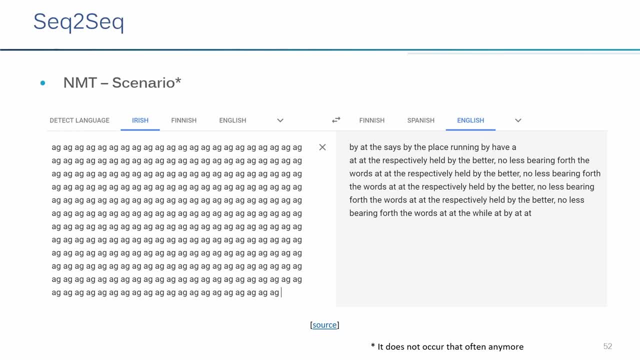 a short note about time and also think about keep things short. Also, it's really cool to see that I am going to create a lot of rest sic statements, And I'll come back to that a little bit later because, somewhat of my experience, it's more forward. 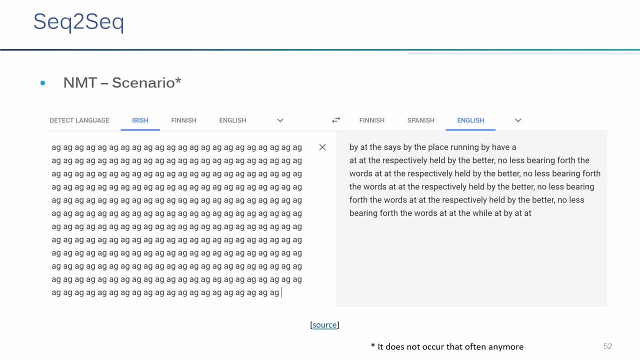 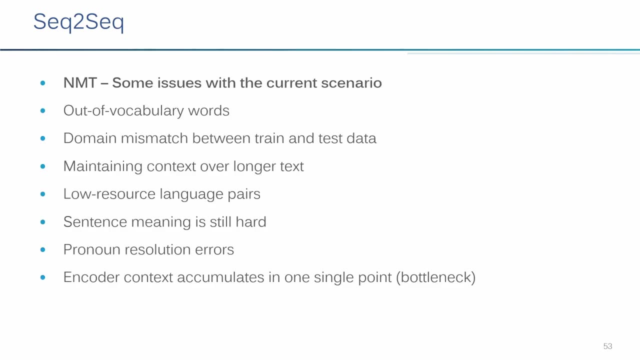 wording provide whatever text with the highest probability they had in this case were text from Bible, Bible and religious texts. this doesn't happen that often anymore, at least not for the examples that I play with, but in any case. so some issues still with the current scenario we have out of vocabulary words domain. 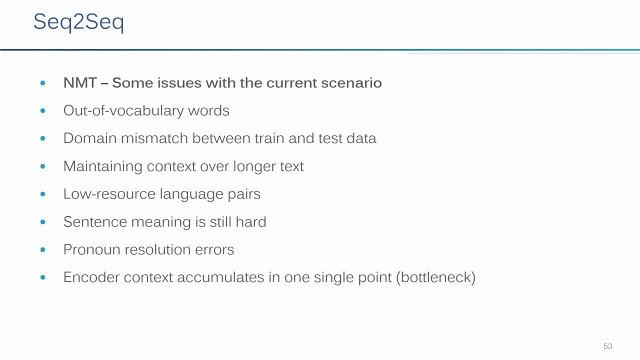 is matched between train and test data, because, while on the train, you have everything in line when you get to test, is not that trivial, because you can provide a, let's say, a word or sentence that you're trying to translate and you have no information about- I don't know- a specific word that you use, so you won't. 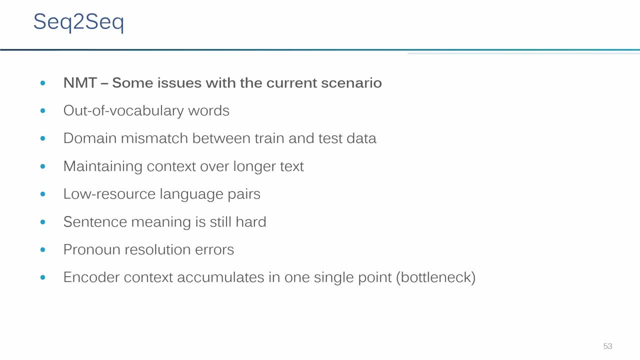 be able to produce a one-to-one translation in this direction. maintaining context over longer attacks is simply complicated because of the bottleneck problem that we have here at the bottom. you have to be able to do a lot of things in the same time, so you have to. 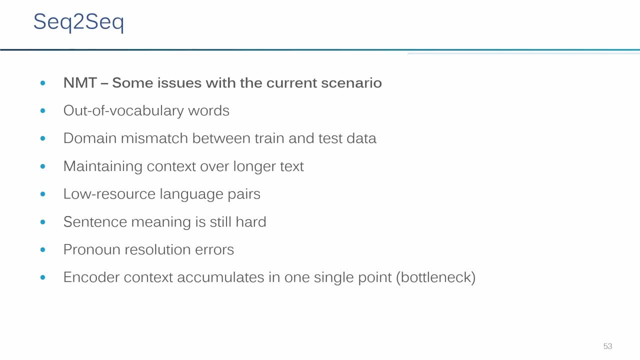 be able to do a lot of things in the same time. so you have to low resource language pairs. they are still a problem, simply because you don't have enough content to train these models sequence to sequence and then later, when we talk about attention, all these models, they require a lot of texts. 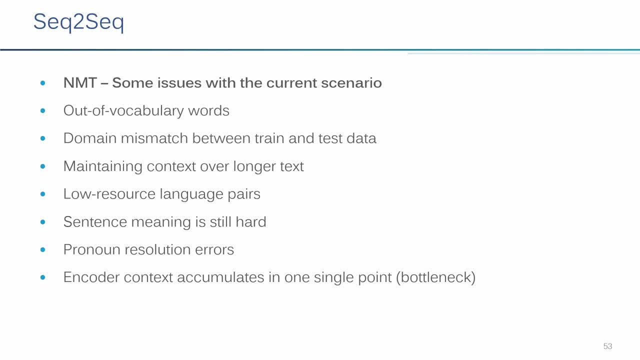 simply they have to optimize those weights a lot. so if you don't have enough examples, the random values that initialize all this weight matrix, they won't produce a good output. sentence meaning it might be hard and the pronoun meaning it might be hard and the pronoun 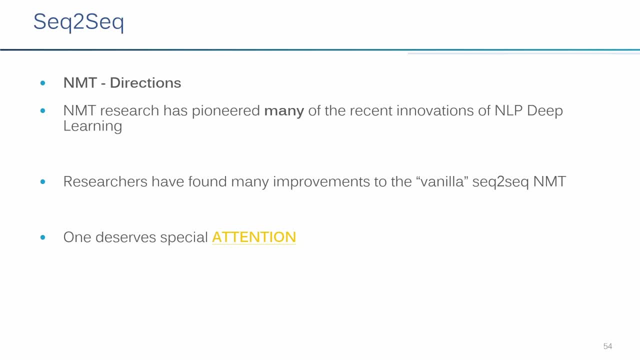 meaning it might be hard, and the pronoun resolutions, as we just saw. so as we saw, a new machine translation research has resolutions, as we just saw. so as we saw, a new machine translation research has resolutions, as we just saw. so as we saw, a new machine translation research has pioneered many of the recent innovations and NLP. 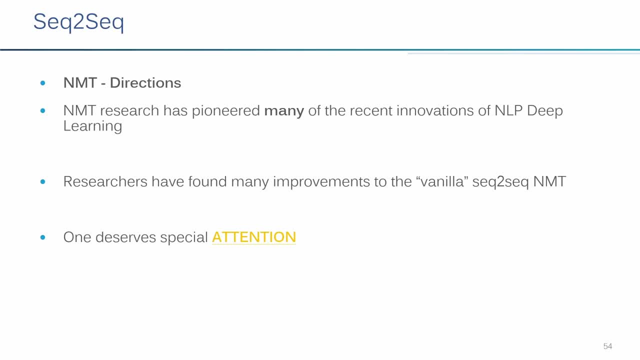 pioneered many of the recent innovations and NLP pioneered many of the recent innovations and NLP deep learning. but again this deep learning. but again this deep learning. but again this vanilla sequence to sequence. people don't use. vanilla, sequence to sequence, people don't use. vanilla, sequence to sequence, people don't use anymore. they're different alternatives. 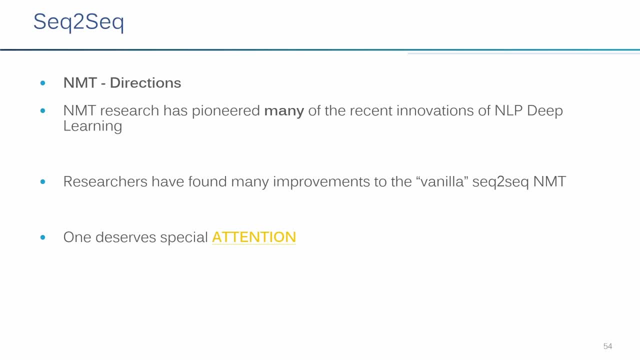 anymore. they're different alternatives. anymore they're different alternatives to, and different architectures there are to, and different architectures there are to, and different architectures there are built on top of that, but one of them built on top of that, but one of them built on top of that, but one of them deserves special attention. this is why. 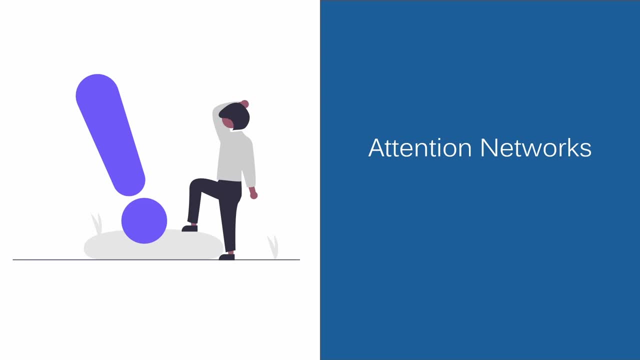 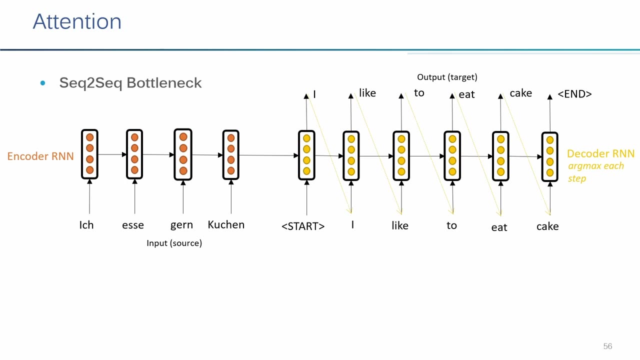 deserves special attention. this is why deserves special attention. this is why we'll talk about that attention networks. we'll talk about that attention networks, we'll talk about that attention networks. so what is attention networks? again we. so what is attention networks? again we. so what is attention networks? again, we have our sequence to sequence model. 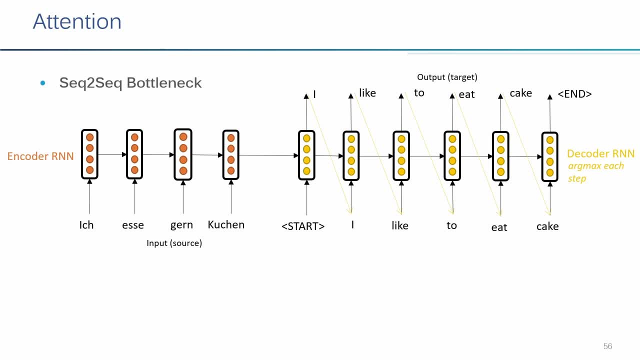 have our sequence to sequence model. have our sequence to sequence model right here, and before we jump into right here and before we jump into right here and before we jump into attention closely from attention. we're attention, closely from attention. we're attention, closely from attention. we're gonna get to self-attention next two. 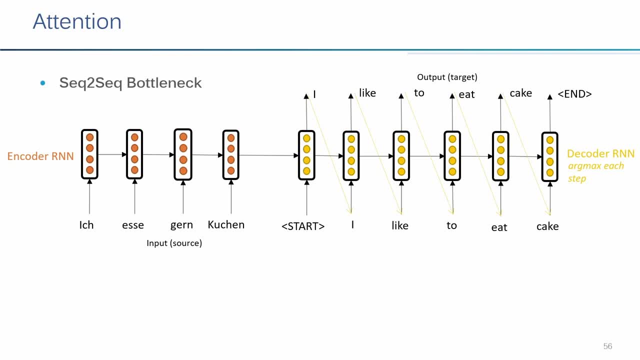 gonna get to self-attention next two. gonna get to self-attention next two: classes don't get frightening, or like if classes don't get frightening, or like if classes don't get frightening. or like if you say, oh, here we use a self-attention, you say, oh, here we use a self-attention. 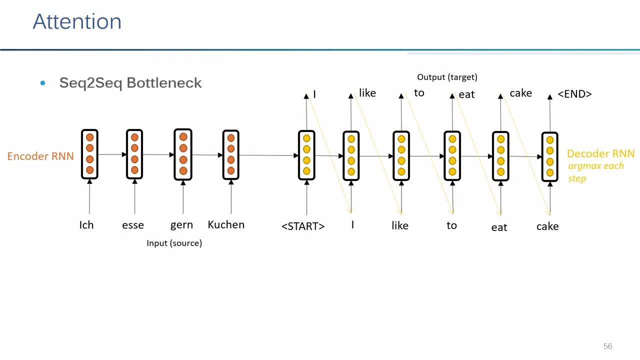 you say: oh, here we use a self-attention. it's not that trivial, like it's a bit. it's not that trivial, like it's a bit. it's not that trivial, like it's a bit different from normal attention and different from normal attention and different from normal attention and self-attention. but in order to grasp that, 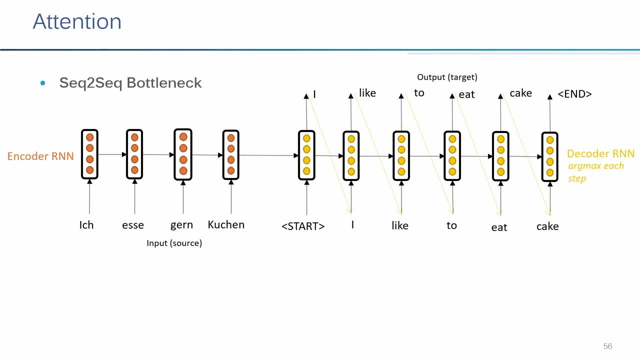 self-attention, but in order to grasp that self-attention, but in order to grasp that, on the Transformers lecture, we should. on the Transformers lecture, we should. on the Transformers lecture, we should take a look into this, but in any case, so, take a look into this, but in any case, so. 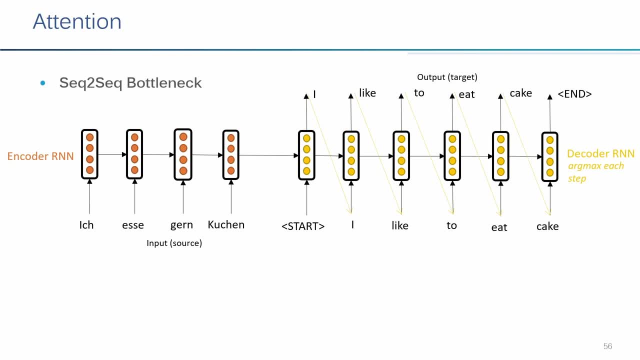 take a look into this, but in any case, so we have our sequence to sequence, we have our sequence to sequence, we have our sequence to sequence. architecture and what we mean by the architecture, and what we mean by the architecture and what we mean by the bottleneck. we already hinted that in a 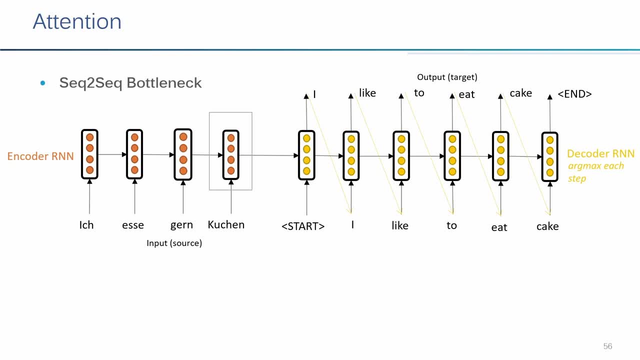 bottleneck. we already hinted that in a bottleneck. we already hinted that in a way that on the very last states that we way that on the very last states that we way that on the very last states that we have our encoder right here we are. have our encoder right, here we are. 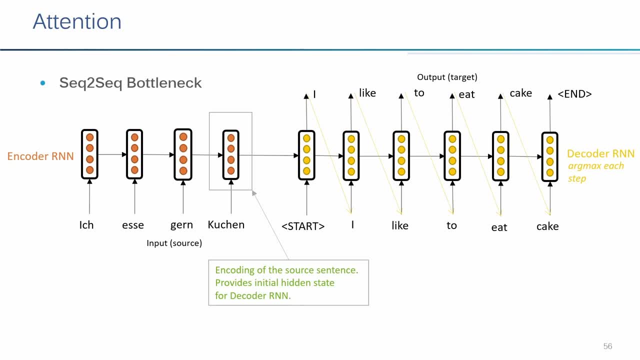 have our encoder right here. we are hoping that this here will provide a hoping that this here will provide a hoping that this here will provide a faithful initial hidden state for all our faithful initial hidden state, for all our faithful initial hidden state for all our decoder part, in a way that this here 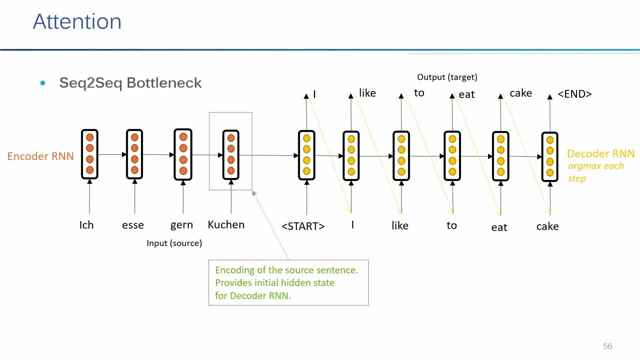 decoder part in a way that this here decoder part, in a way that this here will take account for whatever number of, will take account for whatever number of, will take account for whatever number of steps that we had before and needless to steps that we had before and needless to. 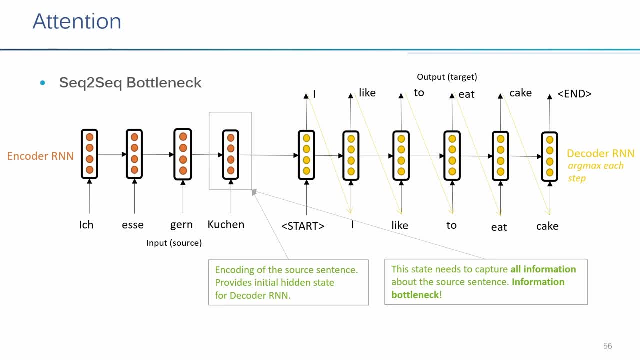 steps that we had before and, needless to say, this is a problem because this say this is a problem because this say this is a problem because this state right here, this last state in our state, right here, this last state in our state, right here, this last state in our encoder and it needs to capture all the 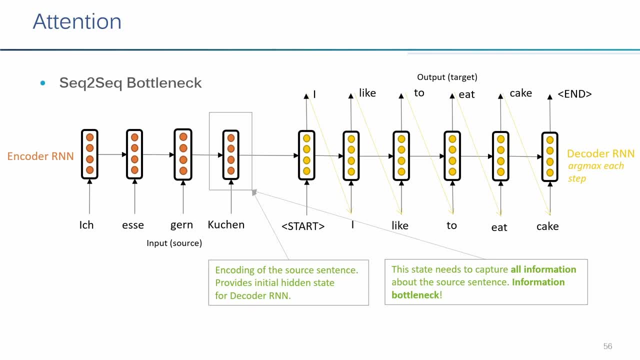 encoder and it needs to capture all the encoder and it needs to capture all the information about the source sentence, information about the source sentence, information about the source sentence, and this here is a bottleneck, simply, and this here is a bottleneck, simply, and this here is a bottleneck simply because 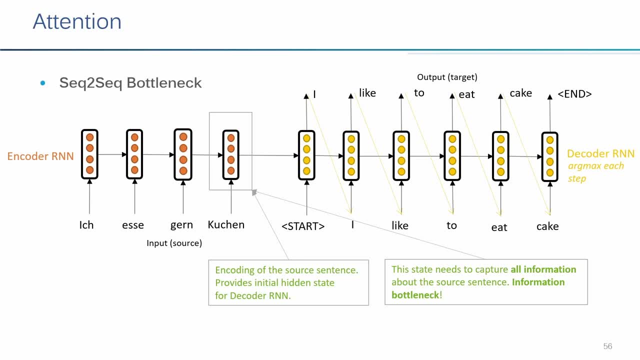 because, because there is no guarantee that this, there is no guarantee that this, there is no guarantee that this- mid-state right here, it will contain mid-state right here. it will contain mid-state right here. it will contain everything that we need to represent, everything that we need to represent. 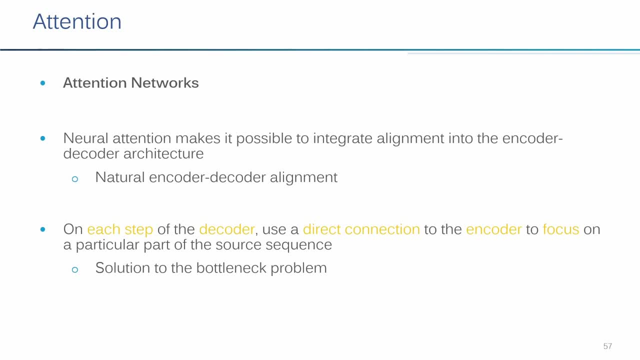 everything that we need to represent our next sentence, our next sentence, our next sentence, so so, so, by using uh neural attention, we'll make it. by using uh neural attention, we'll make it. by using uh neural attention, we'll make it possible to possible, to possible, to integrate the actual alignment that we 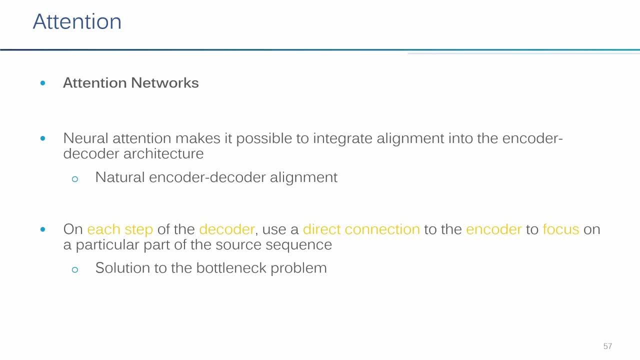 integrate the actual alignment that we integrate the actual alignment that we have, not just by sentence and sentence, have not just by sentence and sentence, have not just by sentence and sentence, but at a token level before we were, but at a token level before we were, but at a token level before we were aligning. 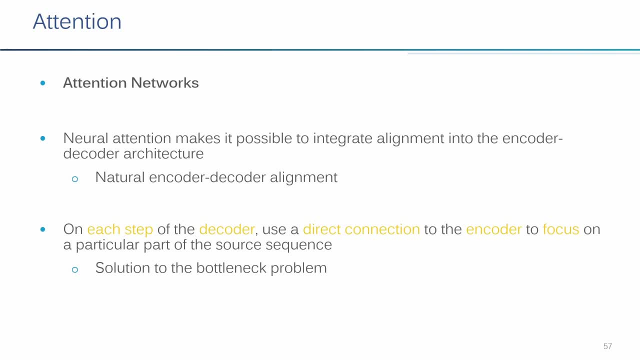 aligning: aligning: uh manually with statistical machine, uh manually with statistical machine, uh manually with statistical machine. translation words by words. translation words by words. translation words by words. then we move to a sequence to sequence, then we move to a sequence to sequence, then we move to a sequence to sequence, in a way that i know that this sentence 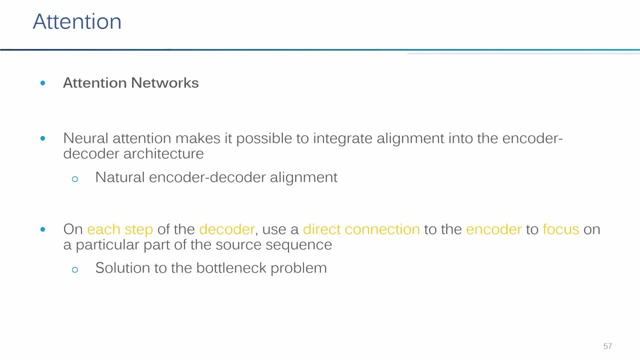 in a way that i know that this sentence, in a way that i know that this sentence here relates with this other sentence, a here relates with this other sentence. a here relates with this other sentence. a and b, but now we can do this at a token- and b, but now we can do this at a token. 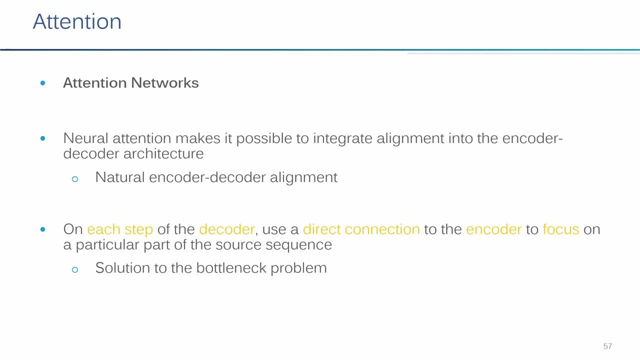 and b, but now we can do this at a token, level, level, level. uh so this, uh this technique. uh so this, uh this technique. uh so this, uh this technique. attention is a natural encoder decoder. attention is a natural encoder decoder. attention is a natural encoder decoder, aligned. 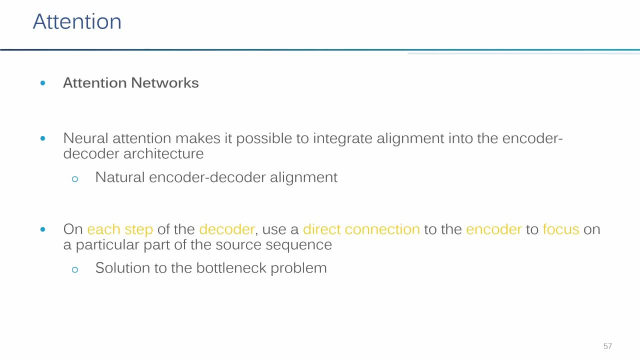 aligned, aligned, and on each step of the decoder we're, and on each step of the decoder we're, and on each step of the decoder, we're going to use a direct, going to use a direct, going to use a direct, direct connection to the encoder, to focus. 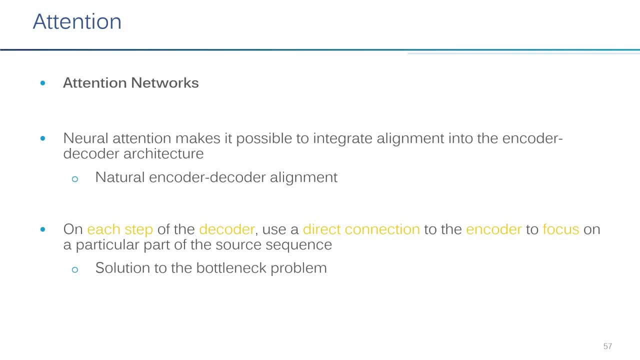 direct connection to the encoder to focus. direct connection to the encoder to focus on a particular part of our, on a particular part of our, on a particular part of our. source sequence in a way that every time source sequence, in a way that every time source sequence, in a way that every time i'm 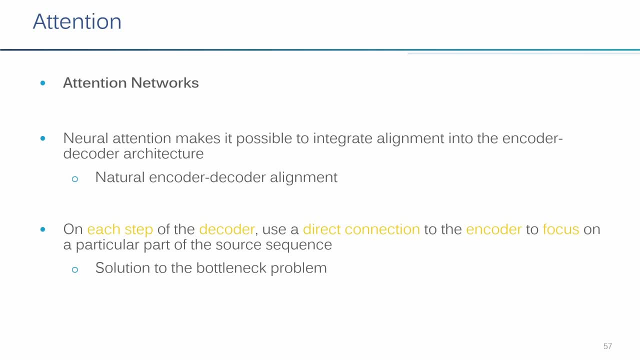 i'm. i'm ultra aggressively predicting every word, ultra aggressively predicting every word, ultra aggressively predicting every word that i have, that i have, that i have. i'll have a sneak peek on my encoder and i'll have a sneak peek on my encoder and i'll have a sneak peek on my encoder and say: okay. 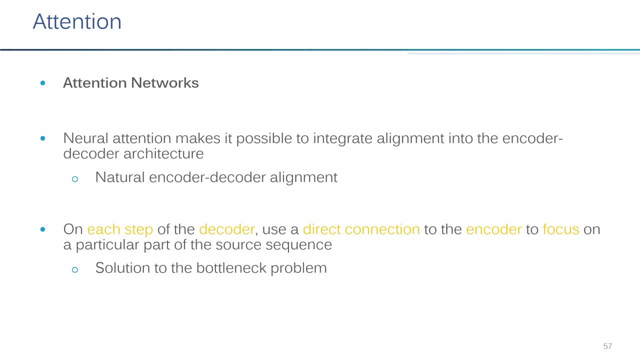 say okay, say okay. from all these words that i have in my, from all these words that i have in my, from all these words that i have in my context, context, context which makes more sense and or which is which makes more sense and or which is which makes more sense and or which is more related. 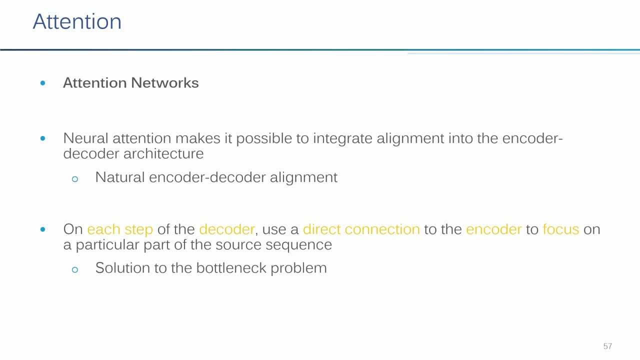 more related, more related with my decoder, and i'll do this for with my decoder and i'll do this for with my decoder and i'll do this for every step in my decoder with these, every step in my decoder with these, every step in my decoder with these direct connections. 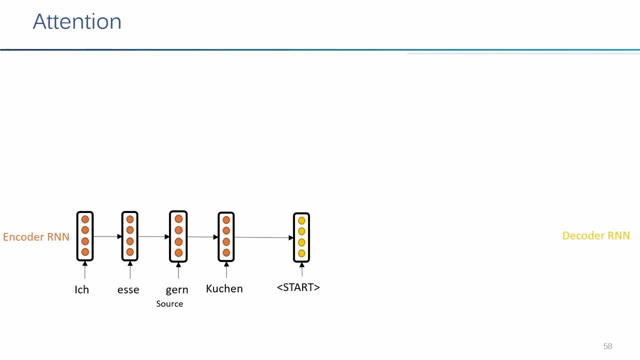 direct connections. direct connections, right, and how this right and how this right and how this looks like. so the idea is: oops, looks like, so the idea is oops, looks like. so the idea is oops. we're gonna have our encoder as before. we're gonna have our encoder as before. 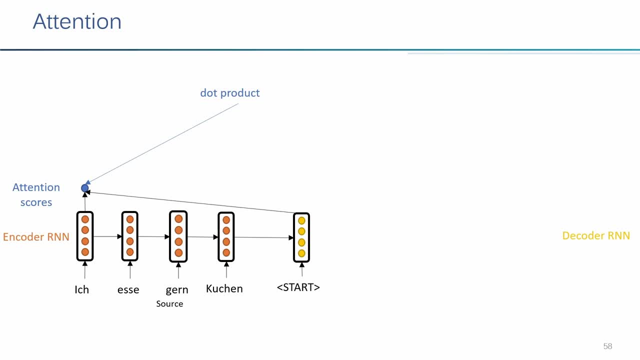 we're gonna have our encoder, as before, but but, but, when we start our our decoder right, when we start our our decoder right, when we start our our decoder right here, here, here, uh, we're gonna use the hidden state. uh, we're gonna use the hidden state. 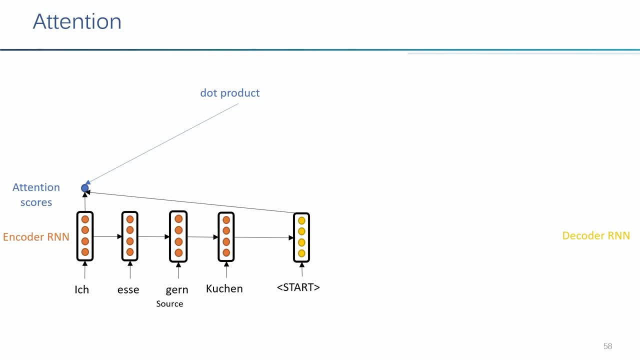 uh, we're gonna use the hidden state from our decoder and our encoder and from our decoder and our encoder, and from our decoder and our encoder and we're going to produce what we call an. we're going to produce what we call an. we're going to produce what we call an attention score by doing the dot product. 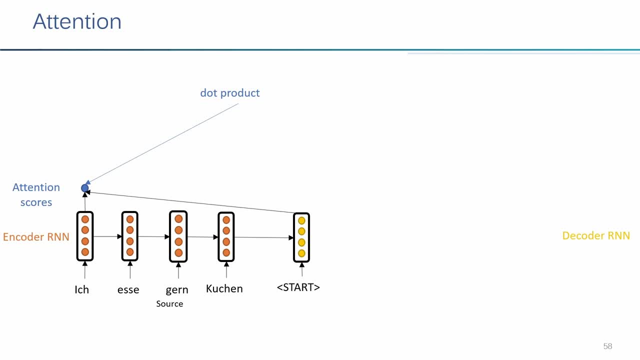 attention score by doing the dot product attention score by doing the dot product between. in this case, since this is the between, in this case, since this is the between, in this case, since this is the first uh, first uh, first uh, on the first state from our decoder and. 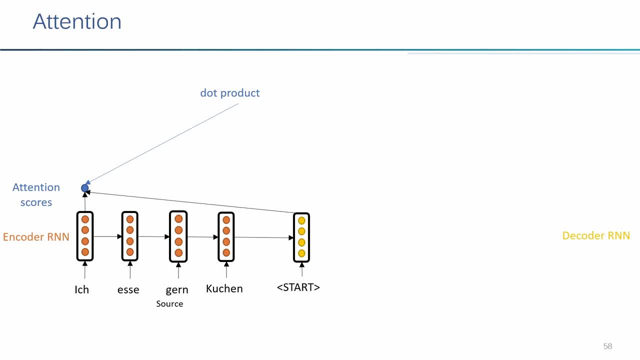 on the first state from our decoder and on the first state from our decoder, and we do this for all the steps in our. we do this for all the steps in our, we do this for all the steps in our encoder in a way that will produce, encoder in a way that will produce. 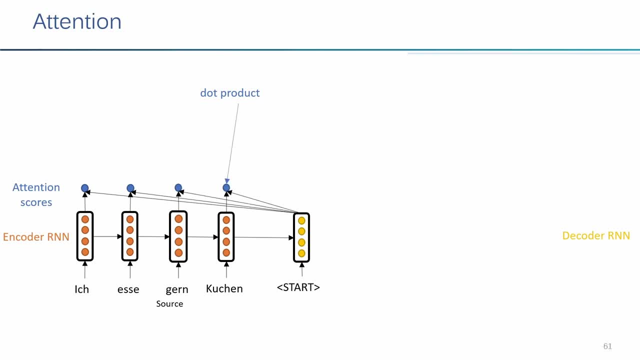 encoder in a way that will produce this attention scores for every single, this attention scores for every single, this attention scores for every single step that we have in our step, that we have in our step, that we have in our encoder, and i hope that i will be able to. 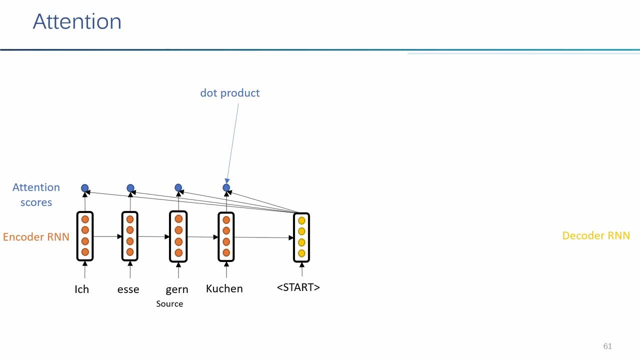 encoder and i hope that i will be able to encoder and i hope that i will be able to associate this step for the next, associate this step for the next, associate this step for the next prediction with the one that makes most, prediction with the one that makes most. 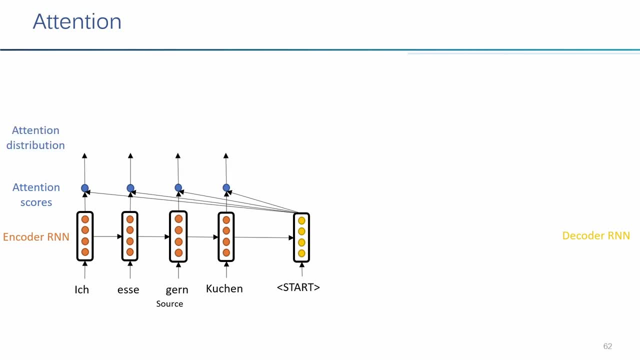 prediction with the one that makes most sense in my sense, in my sense, in my. my encoder part, all right. my encoder part all right, my encoder part all right, uh, uh, uh, so, so, so, and the idea is after we do the dot, and the idea is after we do the dot. 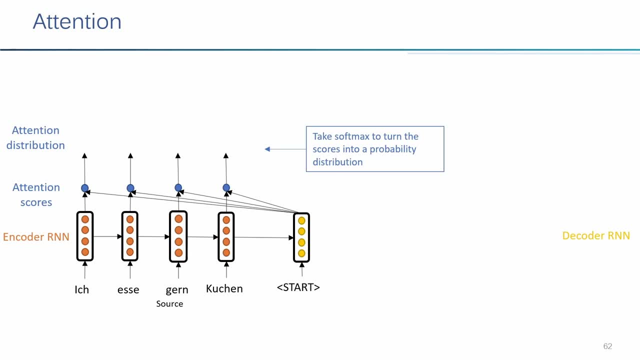 and the idea is, after we do the dot product between the hidden states and product between the hidden states and product between the hidden states and our encoder, and the first step in our our encoder and the first step in our our encoder and the first step in our decoder, we'll take the soft max to take. 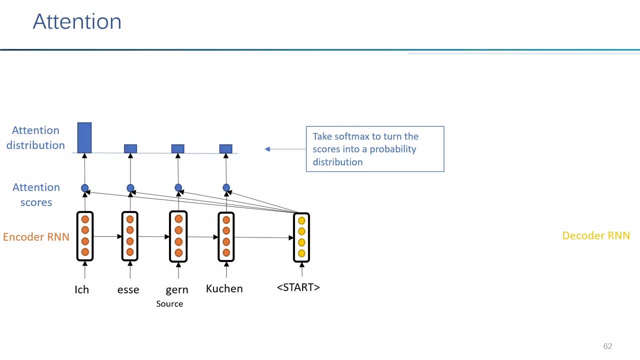 decoder, we'll take the soft max to take decoder, we'll take the soft max to take. uh to transform all this attention. uh, to transform all this attention, uh, to transform all this attention scores into an attention distribution, scores into an attention distribution, scores into an attention distribution. and. 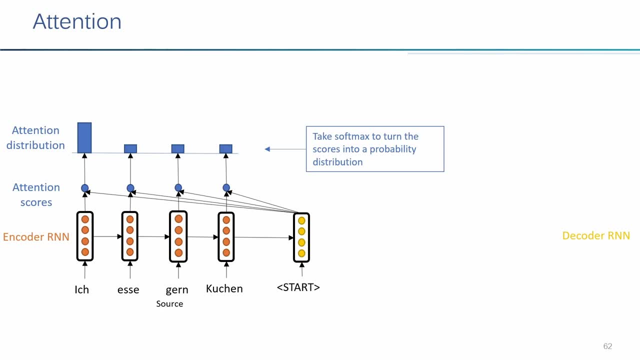 and and by doing this all this year, they have, by doing this all this year, they have, by doing this all this year, they have to sum up to one, and i know that, and we to sum up to one, and i know that, and we to sum up to one, and i know that, and we know that, uh, the the hidden state with 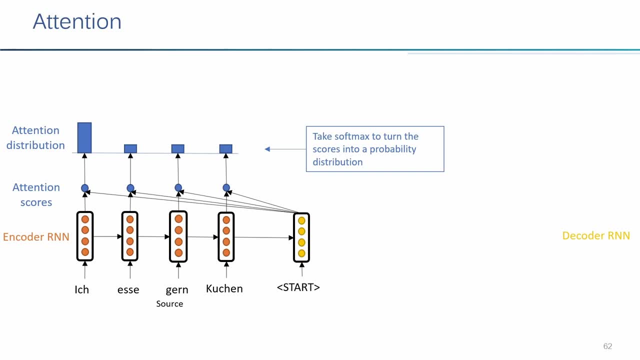 know that, uh, the the hidden state with. know that, uh, the the hidden state with respect to our encoder, with the highest respect to our encoder, with the highest respect to our encoder, with the highest score. score score will also be maximized in this soft max will also be maximized in this soft max. 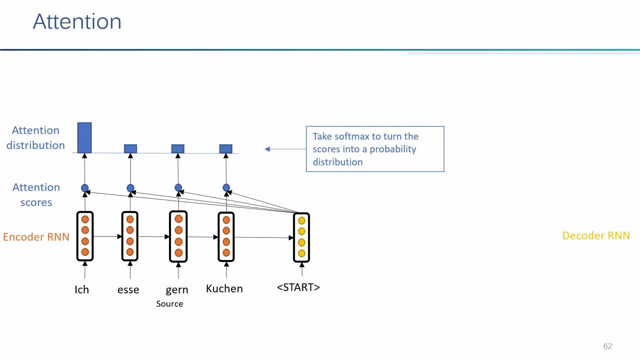 will also be maximized in this soft max right here, so most likely right here, so most likely right here, so most likely. this very first word right here in this, this very first word right here in this, this very first word right here in this case, is case is. 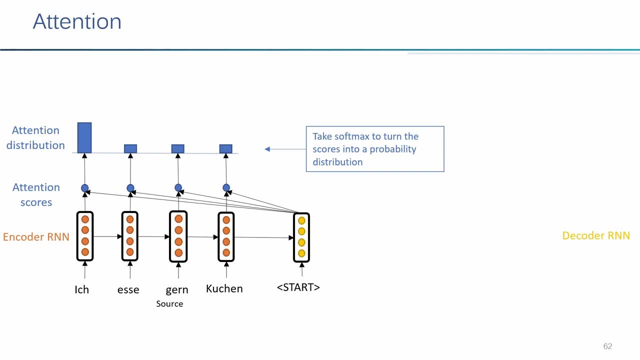 case is, will be related with the very first state, will be related with the very first state, will be related with the very first state in our decoder, and as uh in our decoder, and as uh in our decoder, and as uh, oh yeah, oh yeah, on this step, the decoder time step. 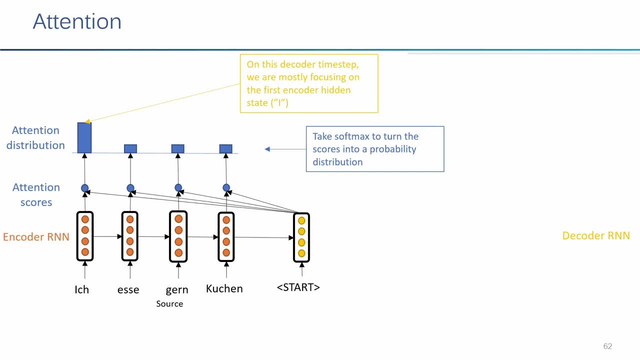 on this step, the decoder time step. on this step, the decoder time step, we're most focusing on the encoder in. we're most focusing on the encoder in. we're most focusing on the encoder in. the state for i in this case is this. the state for i in this case is this. 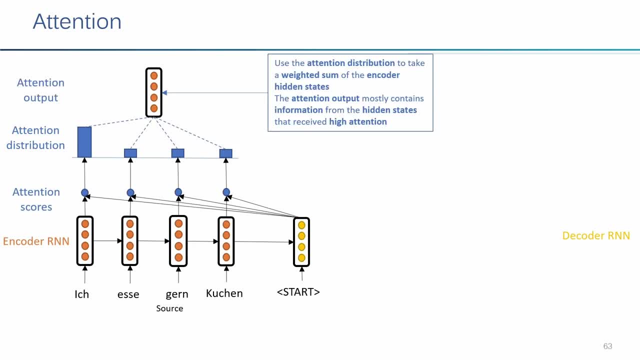 the state for i in this case, is this prediction in our start, prediction in our start, prediction in our start step, and the idea is as we move step, and the idea is as we move step, and the idea is as we move forward, uh, in our decoder forward, uh, in our decoder. 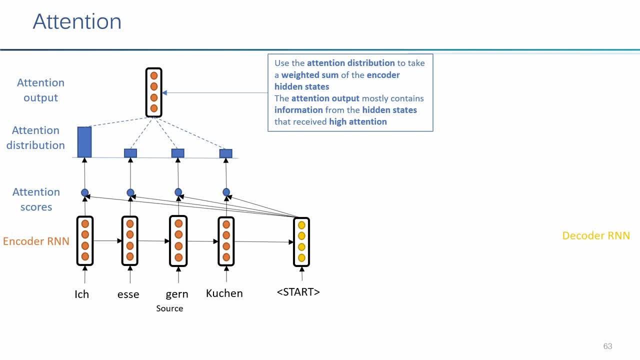 forward. uh, in our decoder for the new steps, we're going to have a for the new steps. we're going to have a for the new steps. we're going to have a different attention distribution in a different attention distribution, in a different attention distribution, in a way that, for every new word that i have, 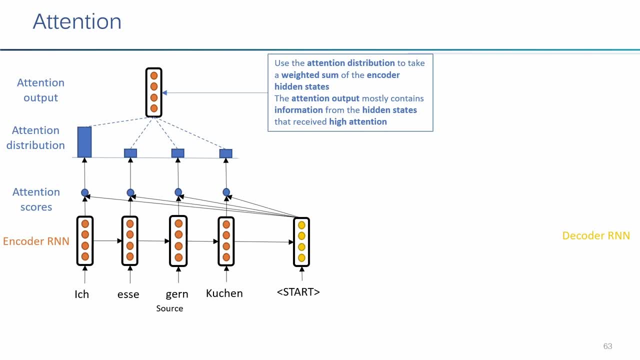 way that for every new word that i have, way that for every new word that i have, this attention distribution change. so this attention distribution change, so this attention distribution change. so we use, we use, we use this attention distribution to take a, this attention distribution to take a. 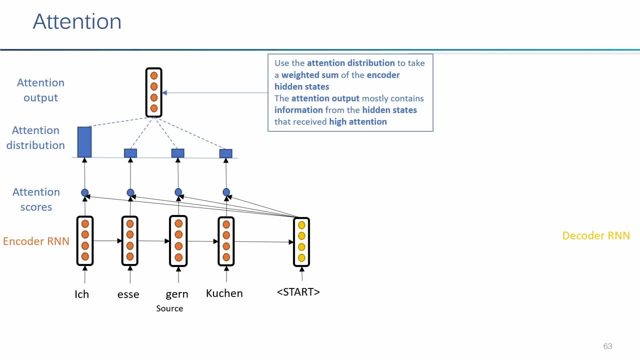 this attention distribution to take a weighted sum of the encoder hidden weighted sum of the encoder hidden weighted sum of the encoder hidden states, states, states, and then our attention output mostly, and then our attention output mostly, and then our attention output mostly contains information from the hidden. contains information from the hidden. 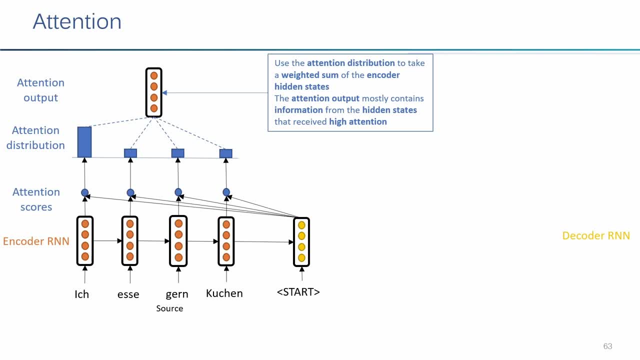 contains information from the hidden states that receive the high states, that receive the high states, that receive the high, the highest attention in this case, right, the highest attention in this case, right, the highest attention in this case, right here. so the idea is here. so the idea is. 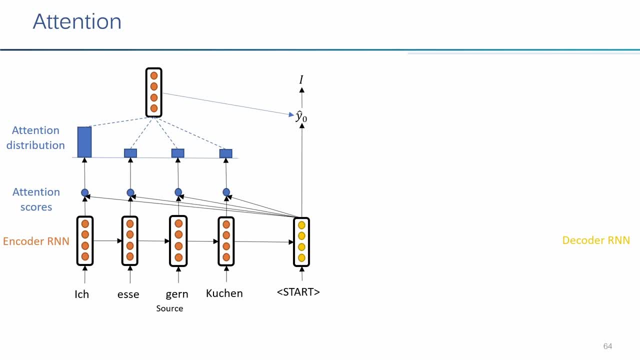 here. so the idea is: after uh, after uh, after uh, we look back and all the steps in our uh. we look back and all the steps in our uh, we look back and all the steps in our uh. encoder: i'll use this attention. encoder: i'll use this attention. 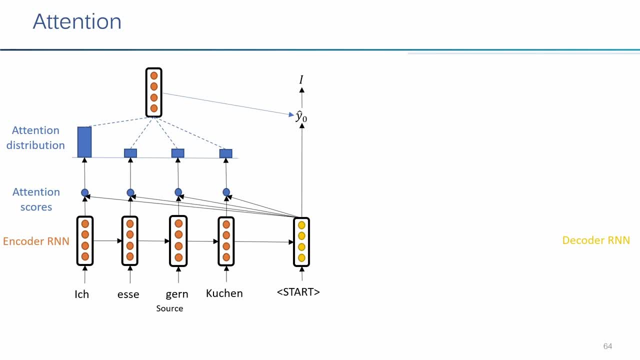 encoder. i'll use this attention distribution right here to help me do a distribution right here to help me do a distribution right here to help me do a better prediction. for which word i'm better prediction for which word i'm better prediction for which word i'm going to predict next. so we concatenate. 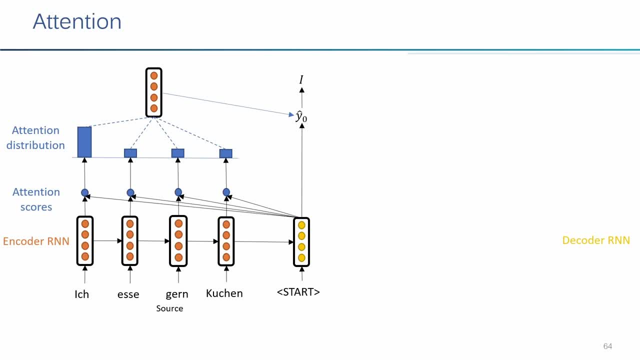 going to predict next, so we concatenate. going to predict next, so we concatenate uh, whatever uh the attention uh output, uh, whatever uh the attention uh output, uh whatever uh the attention uh output that we had in our encoder, that we had in our encoder, that we had in our encoder- considering this decoder right here, and 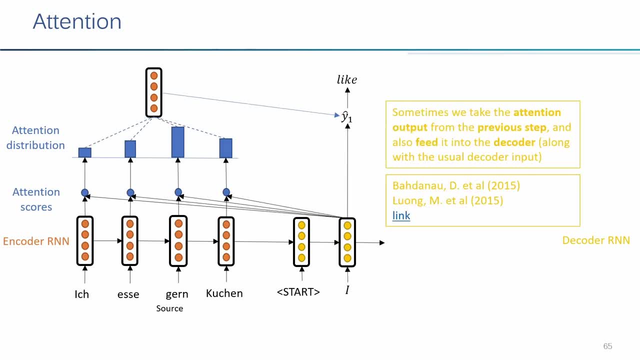 considering this decoder right here and considering this decoder right here, and then we do our prediction. then we do our prediction, then we do our prediction for, uh, the next step. we do pretty much for uh, the next step. we do pretty much for uh, the next step. we do pretty much the same thing, but now we're not taking. 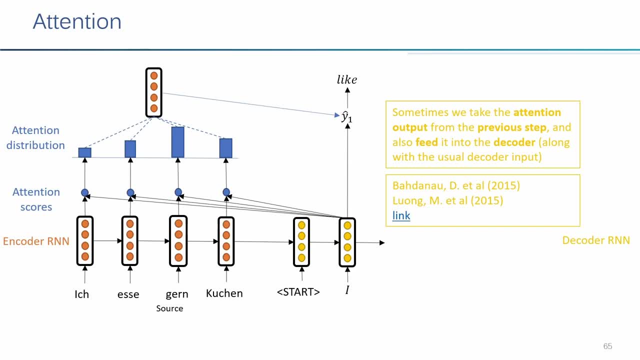 the same thing, but now we're not taking the same thing, but now we're not taking into account more the previous step into account, more the previous step into account, more the previous step. aside from the actual hidden state from aside from the actual hidden state, from aside from the actual hidden state from our decoder. 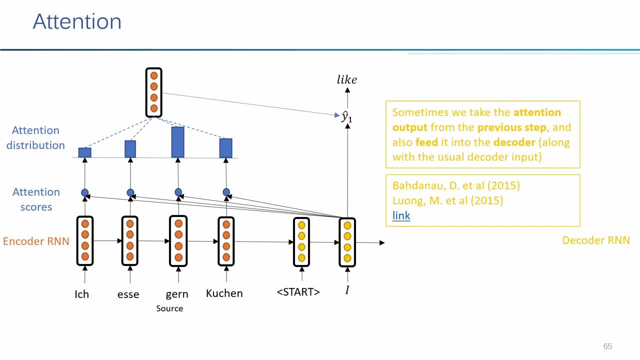 our decoder, our decoder, but we do the dot product again from the. but we do the dot product again from the. but we do the dot product again from the new decoder state with all the steps in new decoder state, with all the steps in new decoder state, with all the steps in our encoder and our attention. 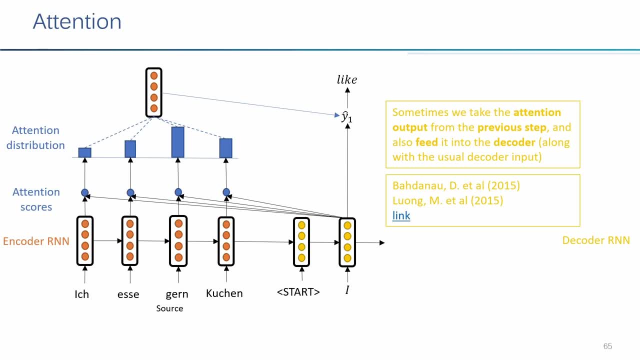 our encoder and our attention. our encoder and our attention. distribution will change. see, because distribution will change. see, because distribution will change. see, because the word related in this second step, the word related in this second step, the word related in this second step right here, most likely will not be the. 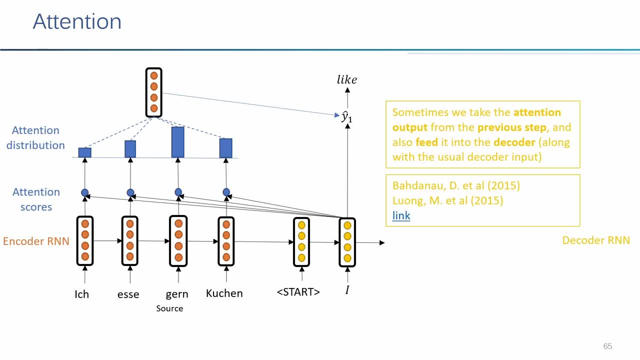 right here, most likely will not be the right here, most likely will not be the first one. first one, first one: uh, as we had in the previous example, the uh as we had in the previous example, the uh as we had in the previous example. the thing is, as we optimize this and since 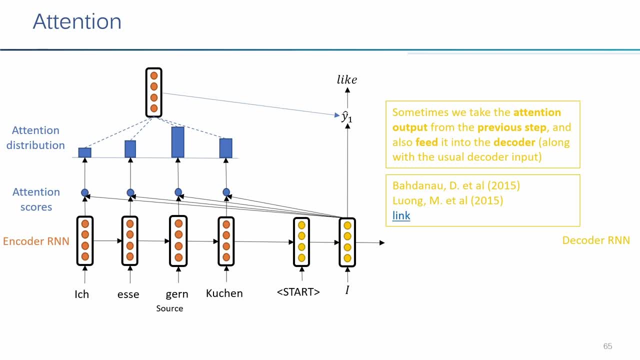 thing is as we optimize this, and since thing is as we optimize this, and since we have the actual, which words we should, we have the actual, which words we should. we have the actual which words we should be predicting here at the training time, be predicting here at the training time. 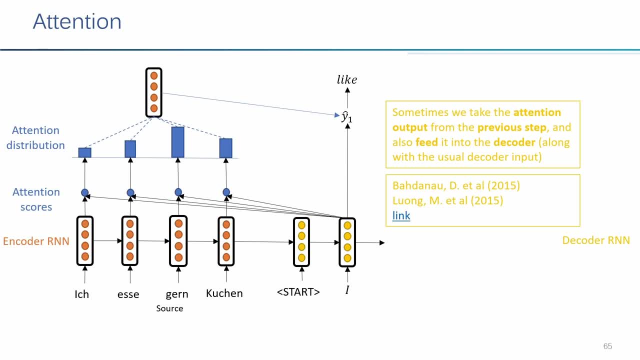 be predicting here at the training time. we're gonna be uh adjusting uh this. we're gonna be uh adjusting uh this. we're gonna be uh adjusting uh this. weights that we are carrying around, all weights that we are carrying around, all weights that we are carrying around, all right. 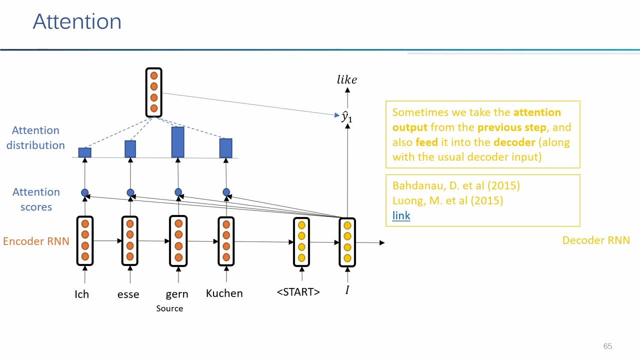 right, right, um, also, um, also, um also. sometimes we take the attention output, sometimes we take the attention output, sometimes we take the attention output from the previous steps. so the previous from the previous steps, so the previous from the previous steps, so the previous step that we just calculated right here. 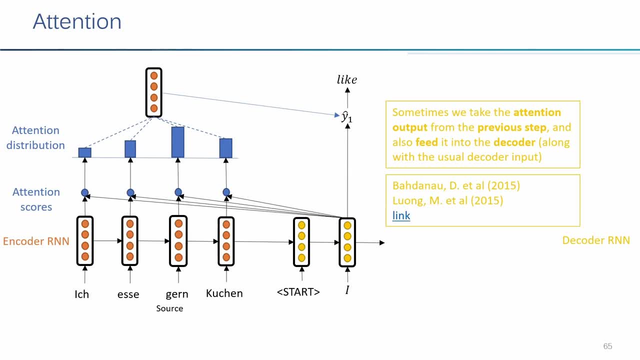 step that we just calculated right here, step that we just calculated right here, and we use this together with the new, and we use this together with the new, and we use this together with the new hidden step to make our prediction so, hidden step to make our prediction so. 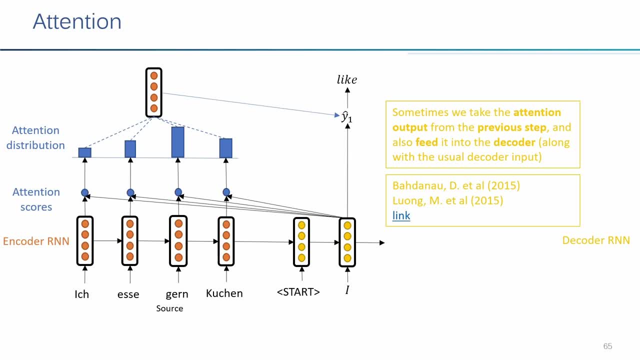 hidden step to make our prediction. so, depending on the architecture that you're depending on the architecture that you're depending on the architecture that you're using, you can either focus on all the using. you can either focus on all the using. you can either focus on all the encoder steps that you had before, or all. 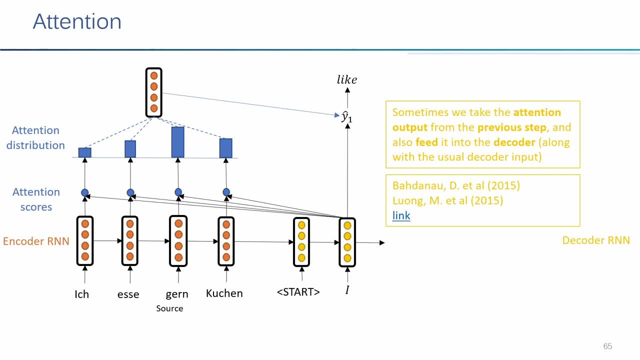 encoder steps that you had before, or all encoder steps that you had before, or all the encoder steps, the encoder steps, the encoder steps, uh, accompanied by the previous uh, uh accompanied by the previous uh, uh accompanied by the previous uh output score that you had. and then we 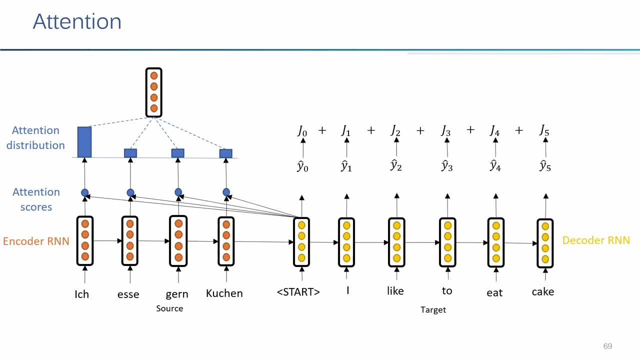 output score that you had, and then we output score that you had, and then we pretty much keep doing this until we pretty much keep doing this, until we pretty much keep doing this, until we reach the end of our seat, reach the end of our seat, reach the end of our seat. our sequence: 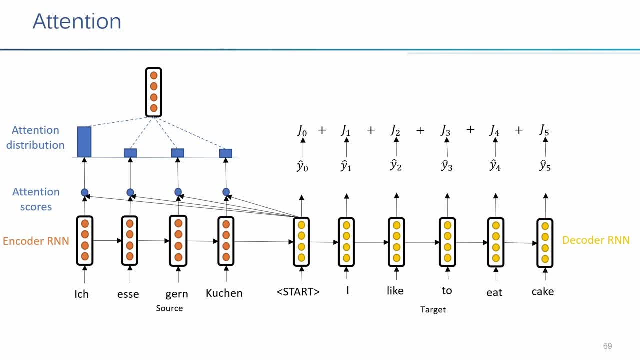 our sequence, our sequence, and the same way as we had before at, and the same way as we had before at, and the same way as we had before at training time. we calculate the loss for training time. we calculate the loss for training time. we calculate the loss for every single prediction. but since we 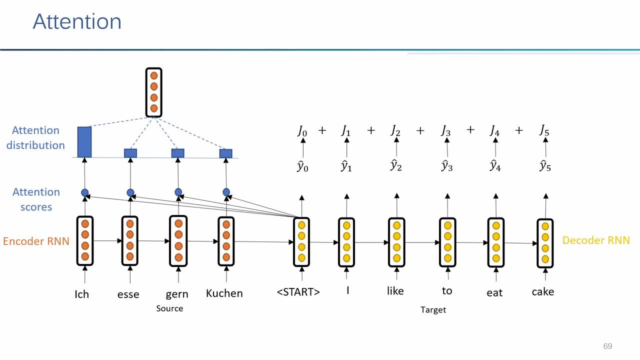 every single prediction. but since we every single prediction. but since we know exactly which word we should be know exactly which word we should be know exactly which word we should be having, here we just use the actual word having. here we just use the actual word having. here we just use the actual word. when we're doing the training and 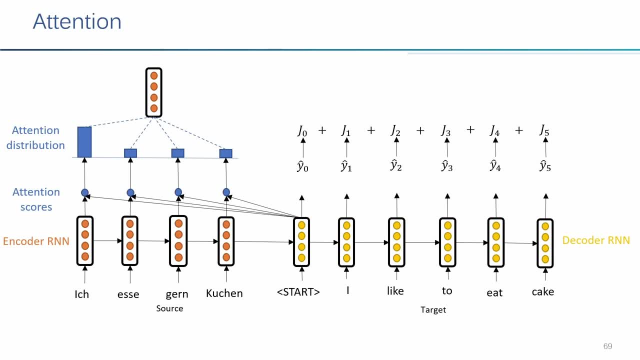 when we're doing the training and when we're doing the training and testing, of course we don't have testing. of course we don't have testing. of course we don't have, uh, the target sentence, uh, the target sentence, uh, the target sentence. okay, okay, okay, different from the other architectures. 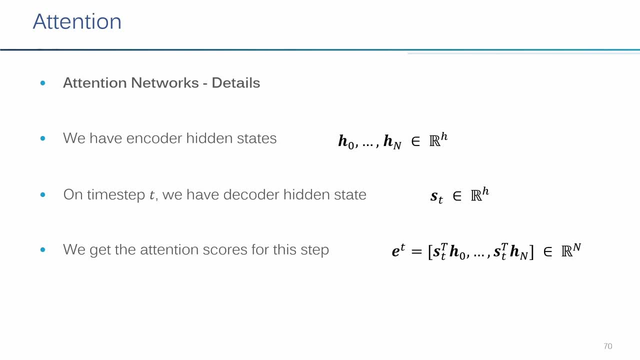 different from the other architectures, different from the other architectures. that we saw. we are not going to do that. we saw we are not going to do that. we saw we are not going to do any jacobians or any partial derivatives, any jacobians or any partial derivatives right now. 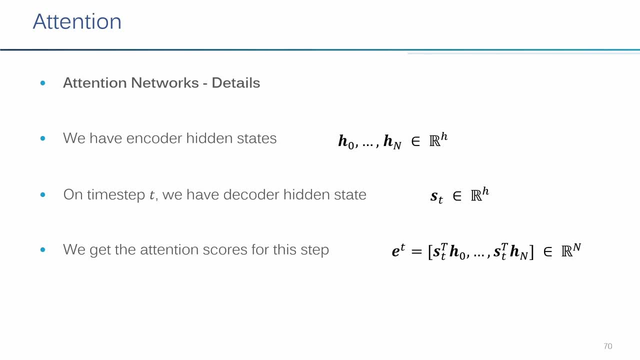 right now. right now, some details to help you remember what. some details to help you remember what. some details to help you remember what are the steps that we are considering. are the steps that we are considering. are the steps that we are considering. we have the encoder hidden states. 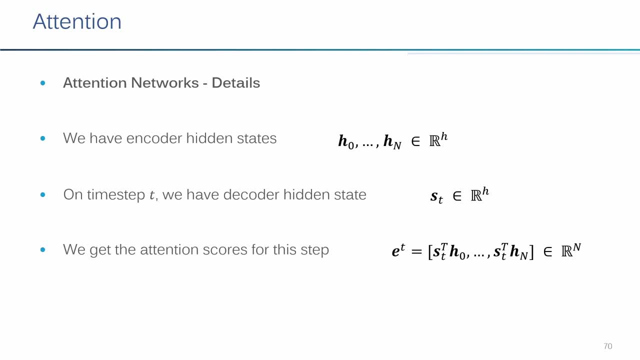 we have the encoder hidden states. we have the encoder hidden states from h0 to hn on on time step t. we have from h0 to hn on on time step t. we have from h0 to hn on on time step t. we have our decoder hidden state, which is our s. 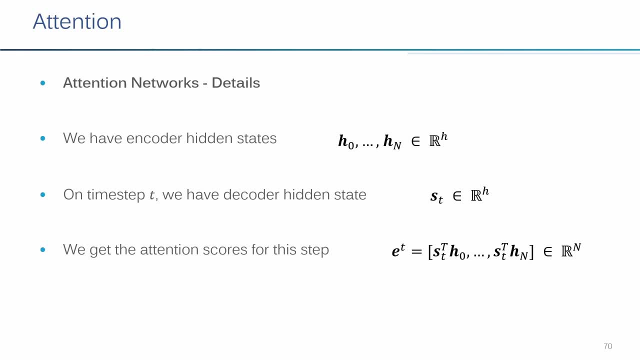 our decoder hidden state, which is our s, our decoder hidden state, which is our s, and then to get the attention score for, and then to get the attention score for, and then to get the attention score for this specific uh, this specific uh, this specific uh, decoder hidden states. we do the dot. 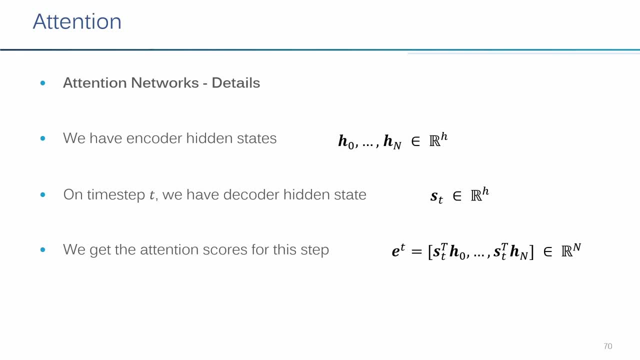 decoder hidden states. we do the dot decoder hidden states. we do the dot product from that product, from that product, from that timestamp in this, in this case t here with timestamp in this, in this case t here with timestamp in this, in this case t here with all the steps that we had before in. 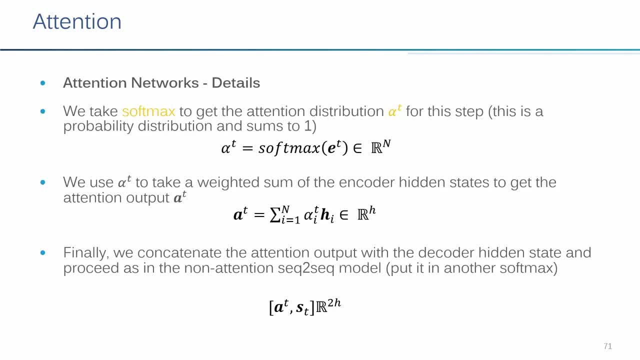 all the steps that we had before in all the steps that we had before in our encoder, our encoder, our encoder. after that we take the soft max to get. after that we take the soft max to get. after that we take the soft max to get the attention distribution. so we take uh. 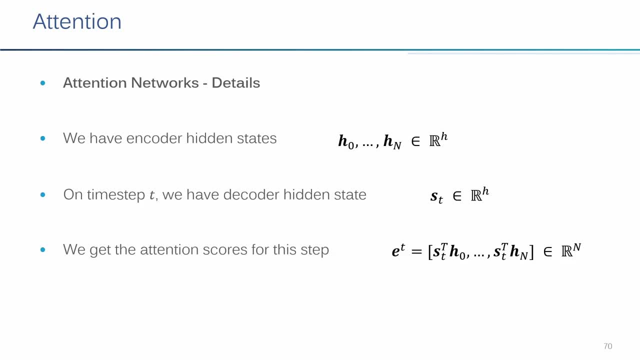 the attention distribution. so we take uh the attention distribution, so we take uh our e that we just calculated right here, our e that we just calculated right here, our e that we just calculated right here with the dot product between decoder and with the dot product between decoder and 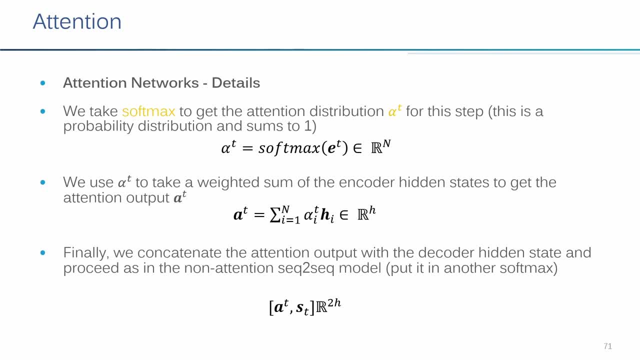 with the dot product between decoder and encoder. we put this in a soft max to get encoder. we put this in a soft max to get encoder. we put this in a soft max to get this, this, this attention distribution, and then we do a attention distribution and then we do a. 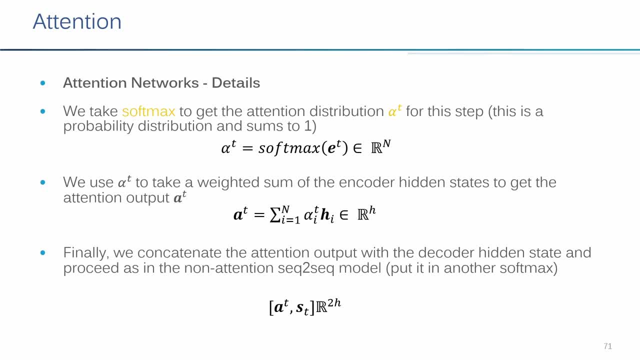 attention distribution. and then we do a weighted, a weighted sum between the weighted, a weighted sum between the weighted, a weighted sum between the encoder hidden states, uh, to get the encoder hidden states. uh, to get the encoder hidden states, uh, to get the attention output that hopefully we will. 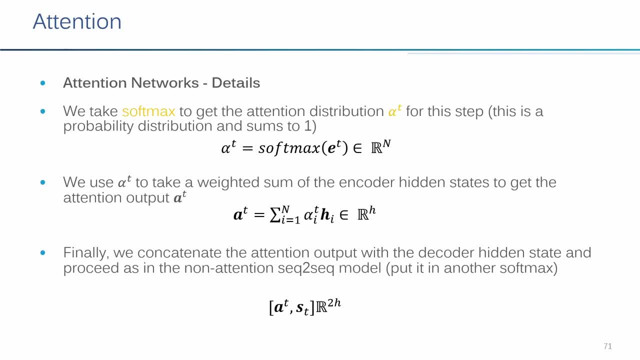 attention output, that hopefully we will attention output, that hopefully we will align our input and our output, align our input and our output, align our input and our output. in the end, we take, uh, that weighted sum. in the end, we take, uh, that weighted sum. in the end, we take, uh, that weighted sum that we calculated right here. 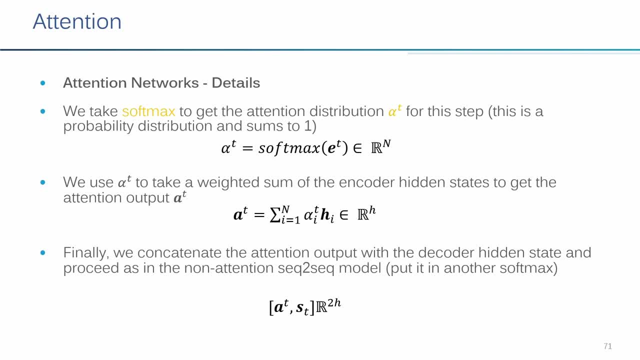 that we calculated right here, that we calculated right here with uh, the prediction that we have in with uh, the prediction that we have in with uh, the prediction that we have in our decoder state and we use our decoder state and we use our decoder state and we use the the. 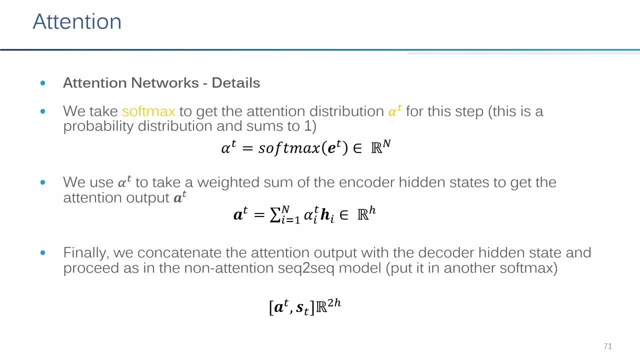 the, the, the, the output scores that we have with decoder output scores. that we have with decoder output scores. that we have with decoder uh prediction, or, in this case, the uh prediction. or, in this case, the uh prediction. or, in this case, the decoder uh hidden state. decoder uh hidden state. 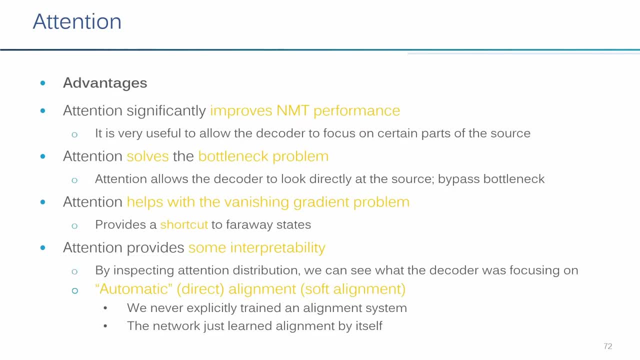 decoder uh hidden state to have our prediction right. to have our prediction right, to have our prediction right. uh, some advantages and i think you know uh some advantages and i think you know uh some advantages and i think you know, i put the disadvantages a bit. i put the disadvantages a bit. 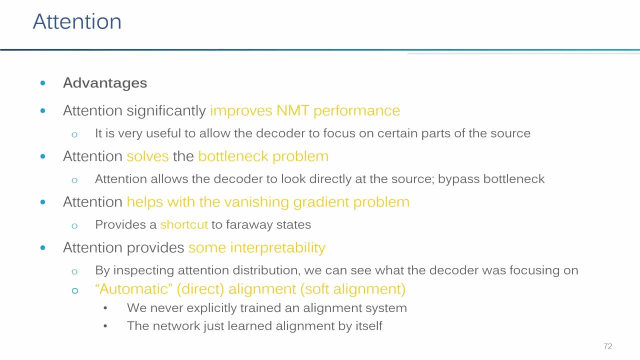 i put the disadvantages a bit, a bit after so. uh, attention a bit after so. uh, attention, a bit after so, uh, attention, significantly improves near machine. significantly improves near machine. significantly improves near machine performance, performance, performance, simply because we allow our decoder to, simply because we allow our decoder to. 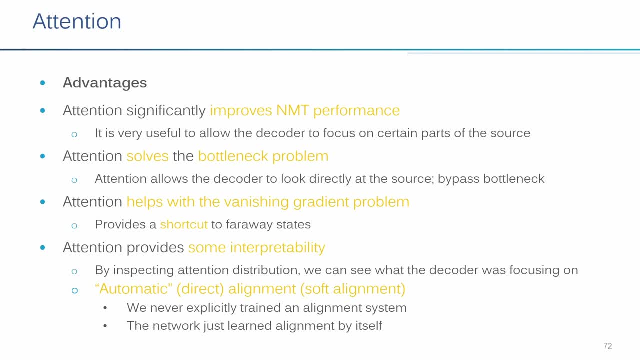 simply because we allow our decoder to attain to specific parts, attain to specific parts, attain to specific parts from our source, from our encoder, and from our source from our encoder, and from our source from our encoder, and this is done kind of automatically, this, this is done kind of automatically. this 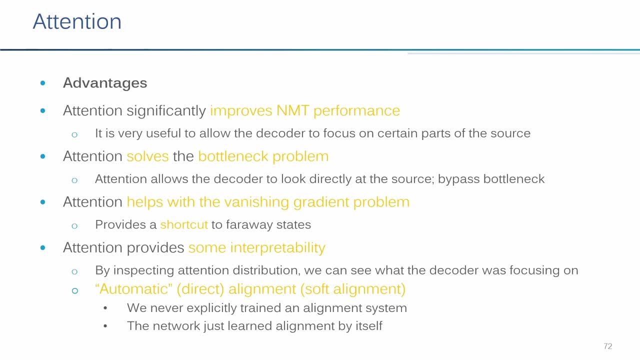 this is done kind of automatically. this solves, solves, solves kind ofish the bottleneck problem in kind ofish the bottleneck problem in kind ofish the bottleneck problem in practice, practice, practice. we have other bottlenecks, so, but let's. we have other bottlenecks, so but let's. 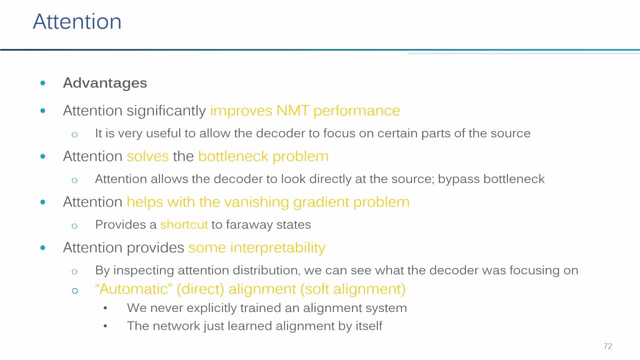 we have other bottlenecks, so but let's believe that, for now, the attention, believe that for now the attention, believe that, for now the attention allows the decoder to look directly at, allows the decoder to look directly at, allows the decoder to look directly at the source, bypassing the last state that 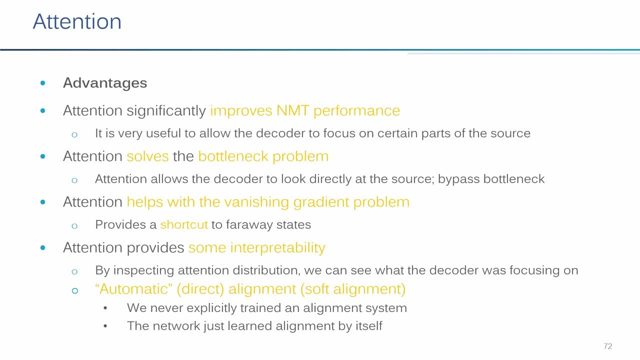 the source, bypassing the last state, that the source, bypassing the last state that i had in my encoder in practice. we'll i had in my encoder in practice. we'll i had in my encoder in practice. we'll see that, see that, see that it doesn't look that far away it. 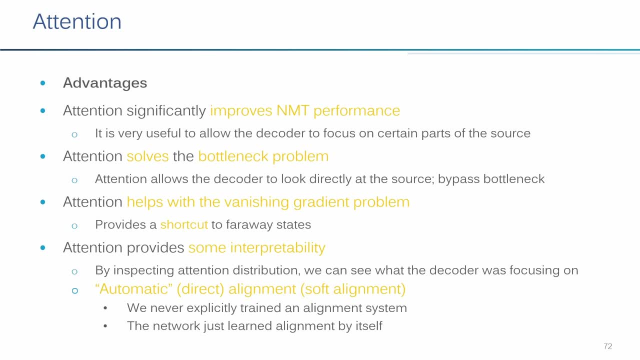 it doesn't look that far away. it it doesn't look that far away, it doesn't. it doesn't take into account the doesn't. it doesn't take into account the doesn't. it doesn't take into account the larger context that good as we wish for. 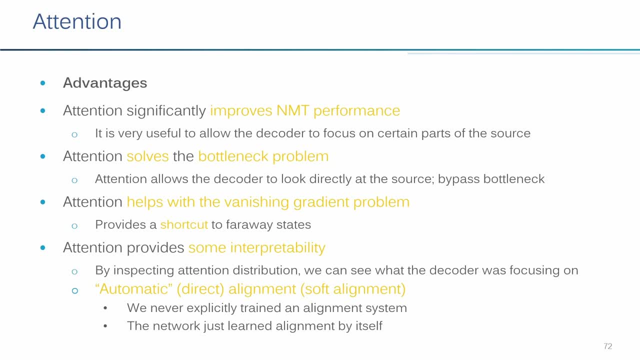 larger context, that good as we wish for larger context, that good as we wish for um, um, um. attention helps with the vanish gradient. attention helps with the vanish gradient problem, simply because now we have problem. simply because now we have problem, simply because now we have a shortcut, shortcut to far away states. so 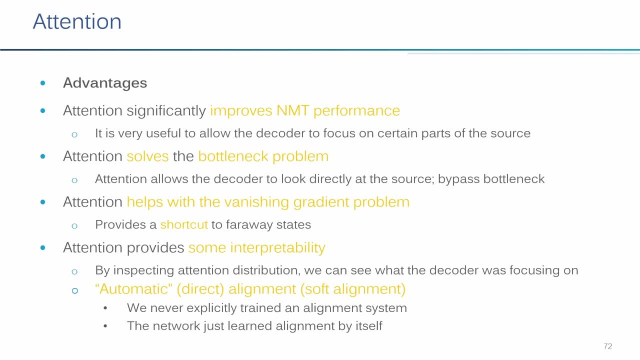 a shortcut shortcut to far away states. so a shortcut shortcut to far away states. so we are connecting every single step in. we are connecting every single step in. we are connecting every single step in our encoder with our decoder directly, our encoder with our decoder directly, our encoder with our decoder directly. attention does. 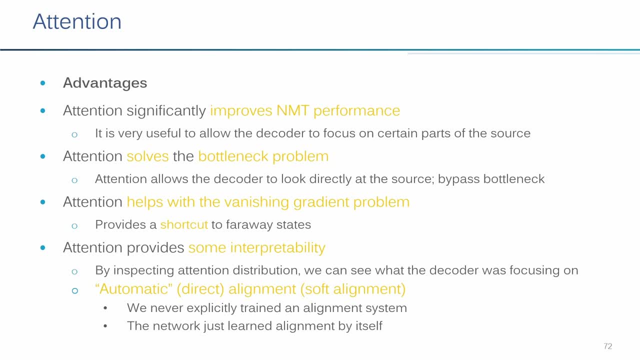 attention. does attention does provide some interpretability, and but provide some interpretability, and but provide some interpretability, and but this here is both an advantage and its. this here is both an advantage and its this here is both an advantage and its advantage. we'll talk later on. 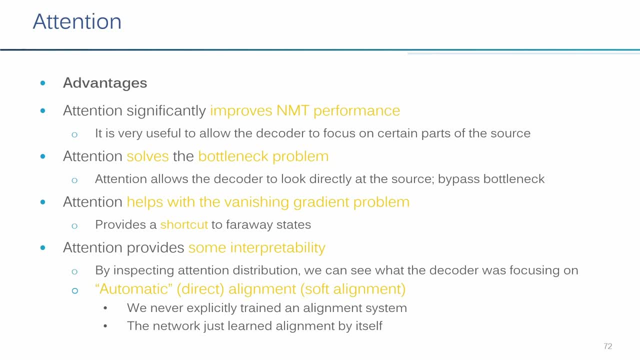 advantage: we'll talk later on. advantage: we'll talk later on. by looking at this, by looking at this, by looking at this output or this distribution scores that output or this distribution scores that output or this distribution scores that we have, you can say okay if whatever we have. you can say okay if whatever. 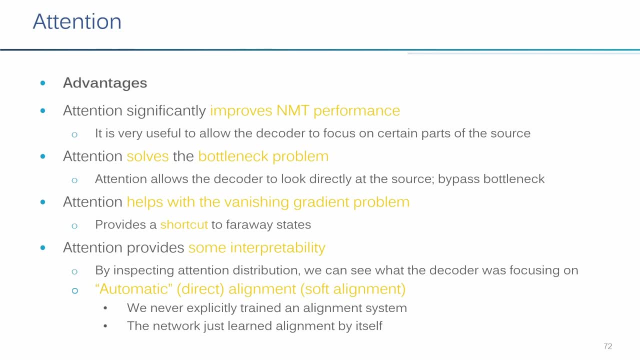 we have. you can say okay, if whatever output that i have has the highest score output that i have has the highest score output that i have has the highest score on this part of my encoder- probably on this part of my encoder. probably on this part of my encoder. probably it's paying more attention to this part. 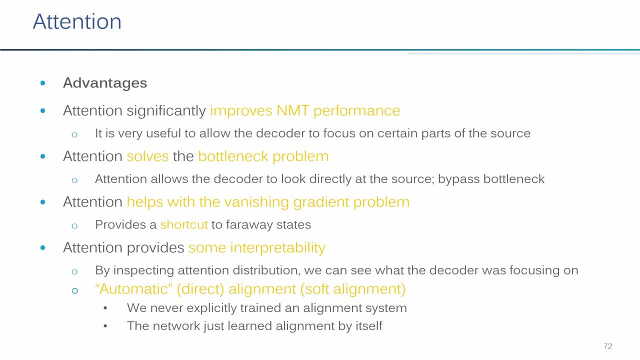 it's paying more attention to this part. it's paying more attention to this part, and you can use this in test time to. and you can use this in test time to. and you can use this in test time to kind of justify why you have a certain 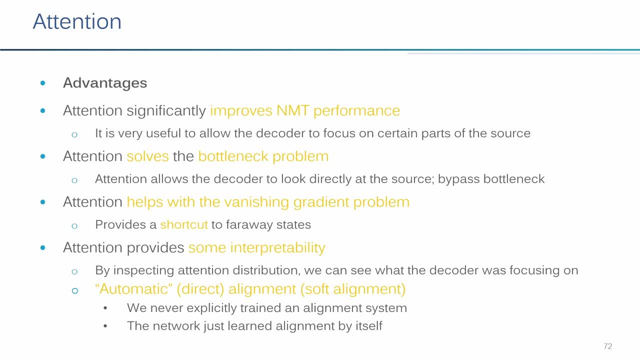 kind of justify why you have a certain, kind of justify why you have a certain, let's say, translation sequence. let's say translation sequence. let's say translation sequence: uh, in practice is not that easy. uh, in practice is not that easy. uh, in practice is not that easy. you don't have to take care anymore by. 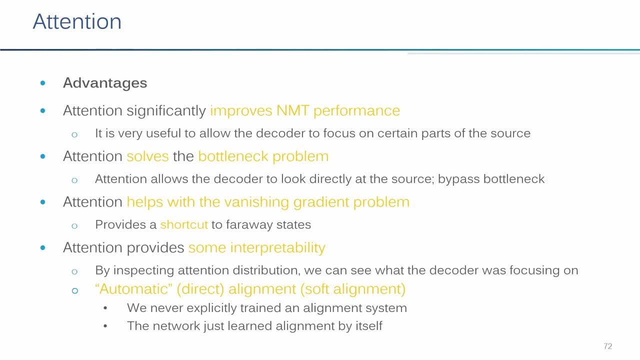 you don't have to take care anymore by. you don't have to take care anymore by. okay. this word has to relate from. okay. this word has to relate from. okay. this word has to relate from. encoder and decoder directly. this is done. encoder and decoder directly: this is done. 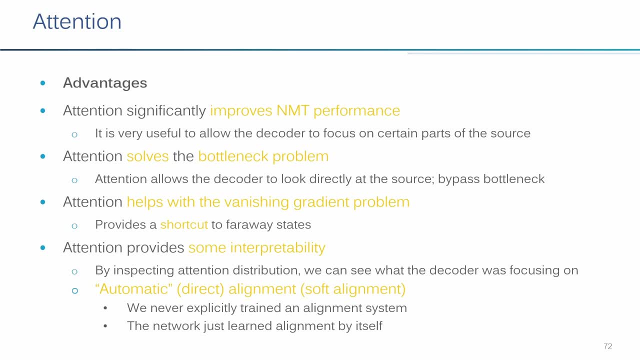 encoder and decoder directly. this is done automatically see because we know automatically see because we know automatically see because we know all the words, from all the words, from all the words, from our input and our output sequence, all our input and our output sequence, all our input and our output sequence. all right. 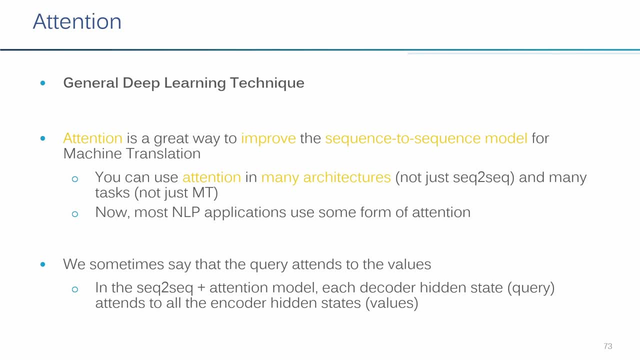 um, um, um, yes, yes, yes. so attention is a great way to improve. so attention is a great way to improve. so attention is a great way to improve. the sequence to sequence model for the sequence to sequence model for the sequence to sequence model for machine translation: machine translation. 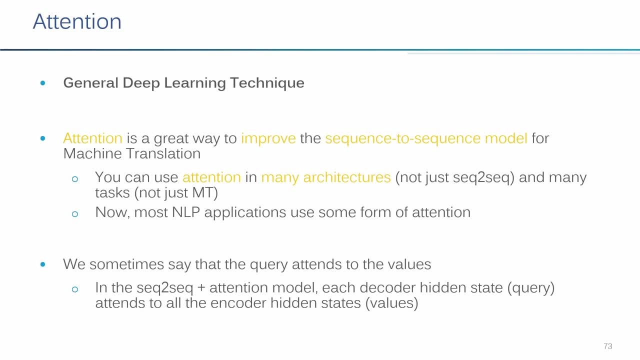 machine translation, and of course you can use this in many, and of course you can use this in many, and of course you can use this in many different architectures, not just different architectures, not just different architectures, not just sequence to sequence, sequence to sequence, sequence to sequence, and not. 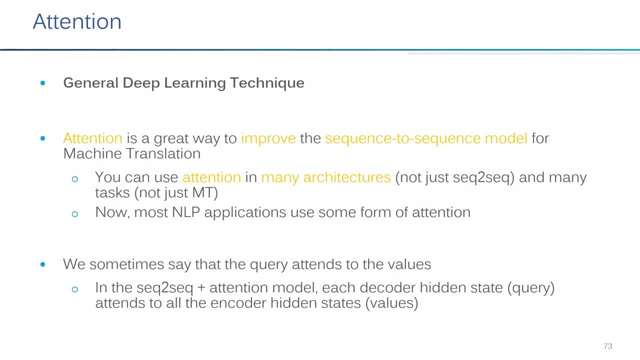 and not, and not just machine translation. we'll see that, just machine translation. we'll see that, just machine translation. we'll see that later on we take this idea of out. later on we take this idea of out. later on we take this idea of out, taking a look from our output and our our. 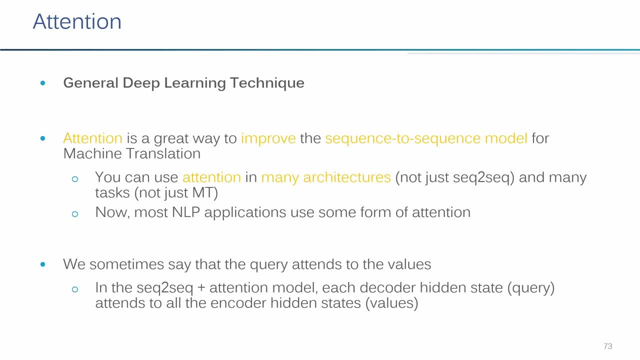 taking a look from our output and our our, taking a look from our output and our, our inputs. and instead of using these two inputs, and instead of using these two inputs, and instead of using these two sentences- we use the same sentence to sentences- we use the same sentence to. 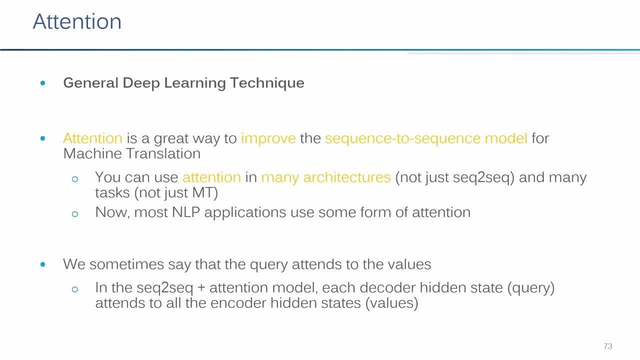 sentences. we use the same sentence to see how the turns between that input. see how the turns between that input. see how the turns between that input. sentence: they pay attention one to sentence. they pay attention one to sentence. they pay attention one to another and this is pretty much self. 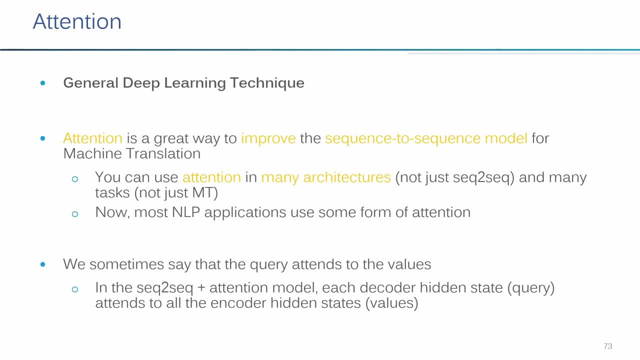 another, and this is pretty much self another, and this is pretty much self. attention, attention, attention, but we'll get there, but we'll get there, but we'll get there also. we sometimes also, we sometimes also. we sometimes say that the query attends to specific, say that the query attends to specific. 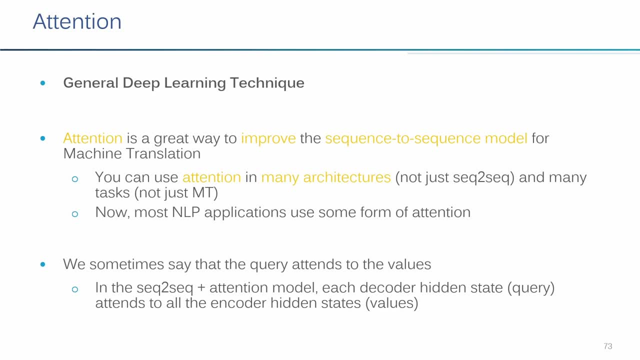 say that the query attends to specific values, and this is the very incipient values and this is the very incipient values and this is the very incipient version when we talk about self version. when we talk about self version, when we talk about self attention that we will see, that we have. 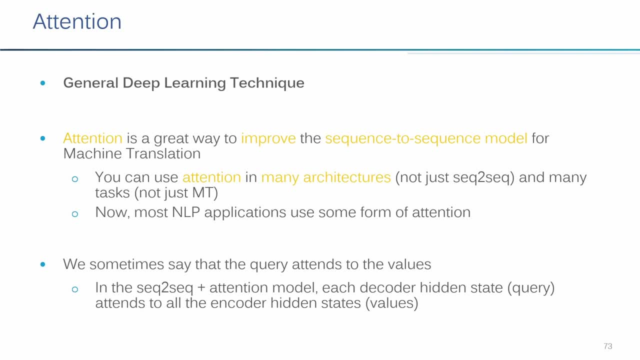 attention. that we will see that we have attention. that we will see that we have query values and keys. think about this: query values and keys. think about this: query values and keys. think about this dynamic between your encoder and decoder, dynamic between your encoder and decoder, dynamic between your encoder and decoder- that you have some sort of a query and 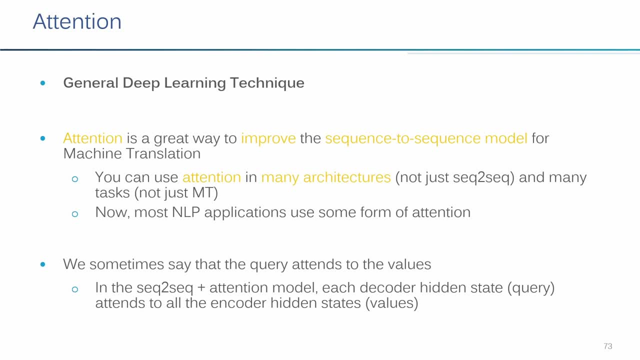 that you have some sort of a query and that you have some sort of a query and that's your decoder and you're looking, that's your decoder, and you're looking, that's your decoder and you're looking back to retrieve specific values and back to retrieve specific values, and 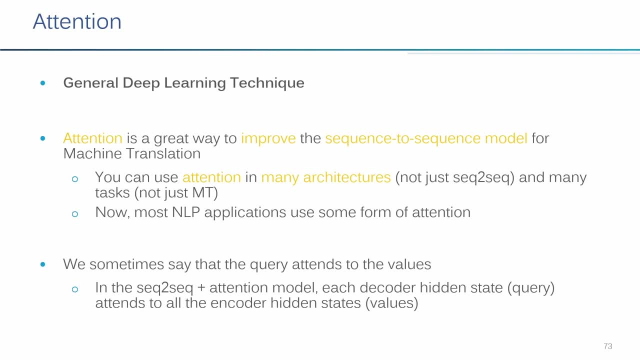 back to retrieve specific values and what are those values, the words that, what are those values, the words that, what are those values, the words that you have in your encoder, so this idea to you have in your encoder, so this idea to you have in your encoder, so this idea to use terms as and weights, of course, as, 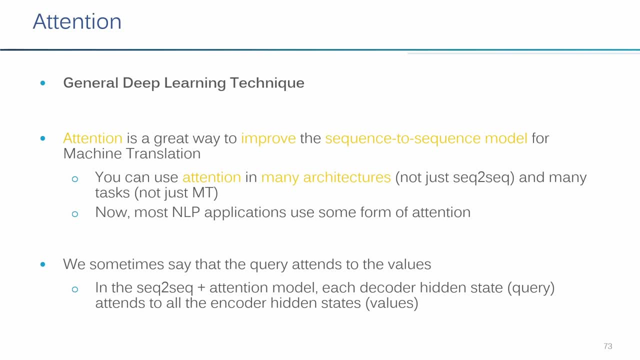 you have in your encoder. so this idea to use terms as and weights, of course, as you have in your encoder. so this idea to use terms as and weights, of course, as query values, and later we'll introduce keys- query values, and later we'll introduce keys- query values and later we'll introduce keys- it starts pretty much with this. 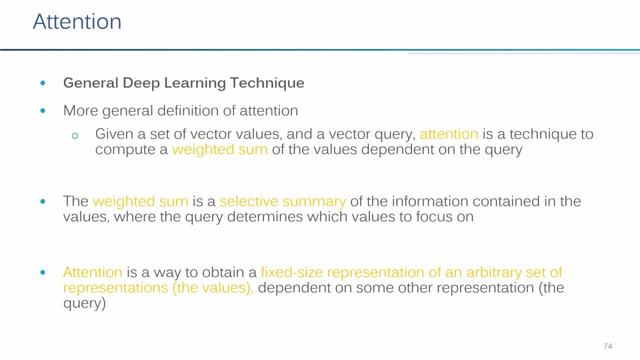 so given just to a more general, so given just to a more general, so given just to a more general definition of attention, given a set of definition of attention, given a set of definition of attention, given a set of vector values, vector values, vector values and a vector query. attention is a. 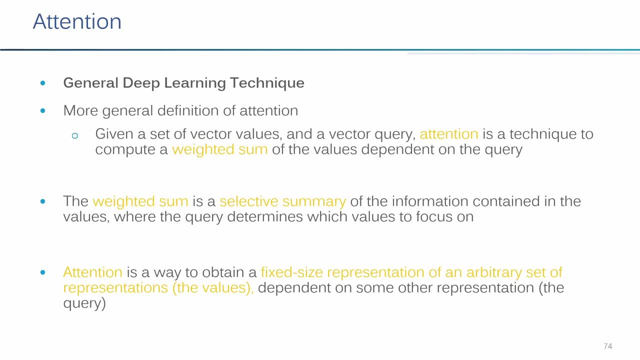 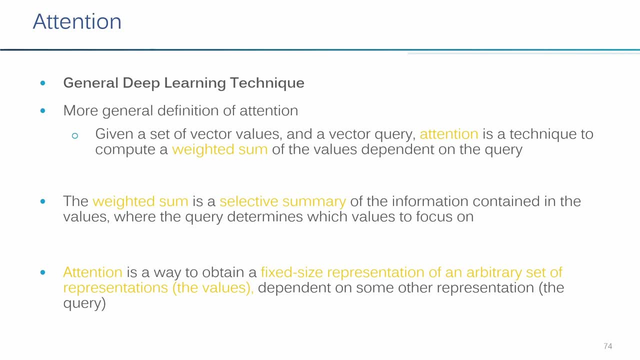 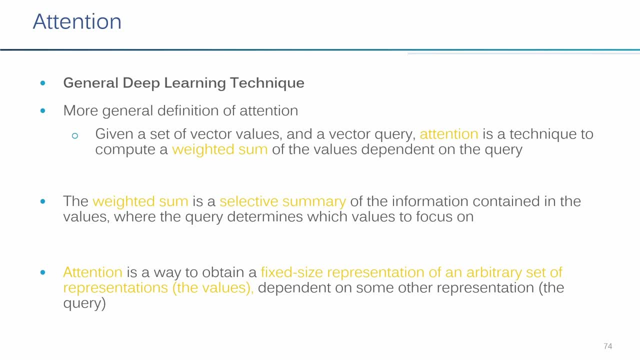 to focus on. so every time i use my word to focus on. so every time i use my word in my decoder as a query, i can probe my in my decoder as a query. i can probe my in my decoder as a query. i can probe my encoder and see, okay, which word i have. 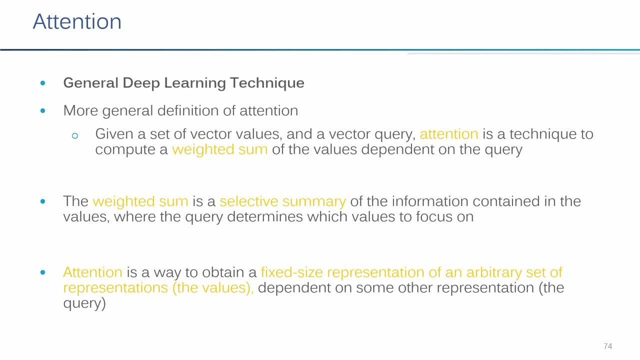 encoder and see, okay, which word i have encoder and see, okay, which word i have to pay attention and which value i want to pay attention and which value i want to pay attention and which value i want to retrieve. to retrieve, to retrieve. uh, this is just the outline we can. 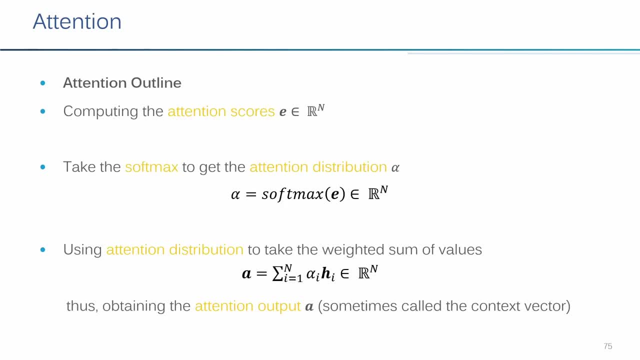 uh, this is just the outline we can, uh, this is just the outline we can actually go to more interesting stuff. actually go to more interesting stuff, actually go to more interesting stuff. this here is already repeated. what we this here is already repeated, what we this here is already repeated, what we just said, it's just to help study on the 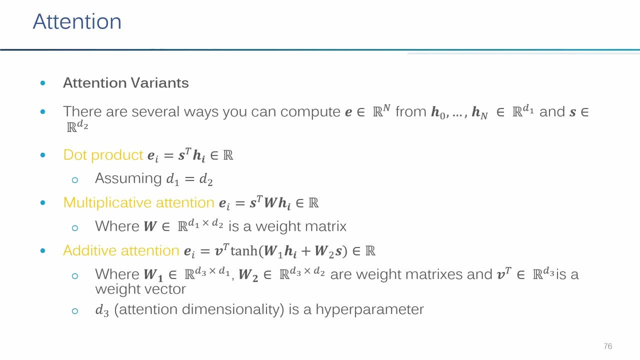 just said it's just to help study on the just said it's just to help study on the summary, summary, summary. so so so, the way we're calculating the similarity, the way we're calculating the similarity, the way we're calculating the similarity between the encoder and decoder, the way 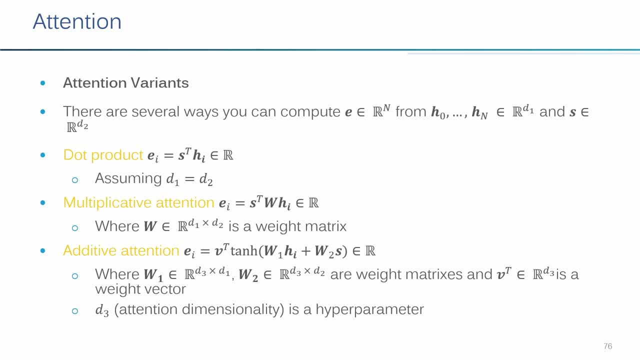 between the encoder and decoder, the way between the encoder and decoder, the way we present with a dot product is not the we present with a dot product is not the we present with a dot product is not the only way of doing this, only way of doing this. 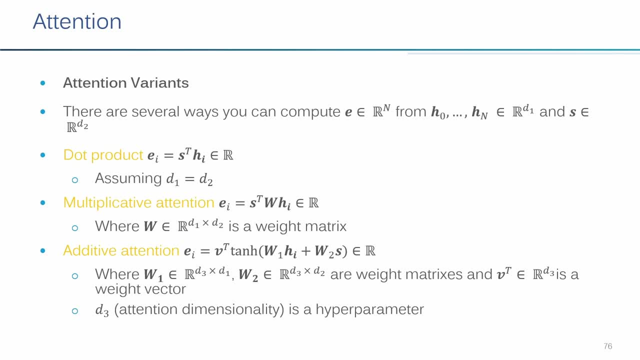 only way of doing this. people have tried to optimize and have people have tried to optimize and have people have tried to optimize- and have a better representation for this dynamic, a better representation for this dynamic. a better representation for this dynamic. the way we just saw is the dot product. 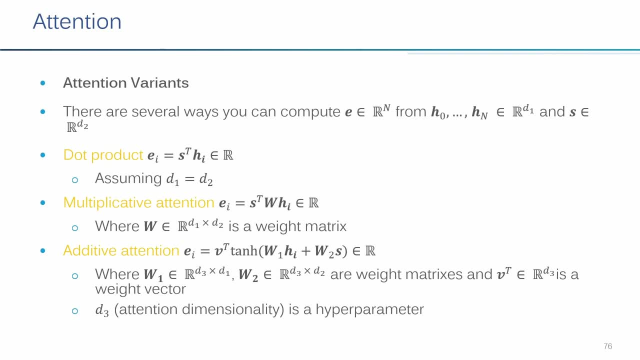 the way we just saw is the dot product. the way we just saw is the dot product in which we multiply our decoder and in which we multiply our decoder and in which we multiply our decoder and encoder. right here, as you can see, the encoder, right here, as you can see, the. 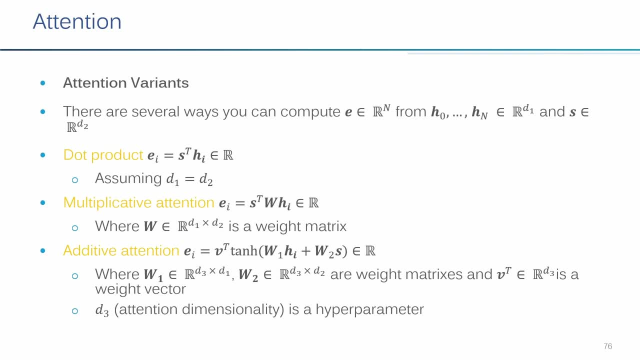 encoder right here, as you can see, the first one, first one, first one. uh, there's also multiplicative attention. uh, there's also multiplicative attention. uh, there's also multiplicative attention in a way that you also do the dot, in a way that you also do the dot. 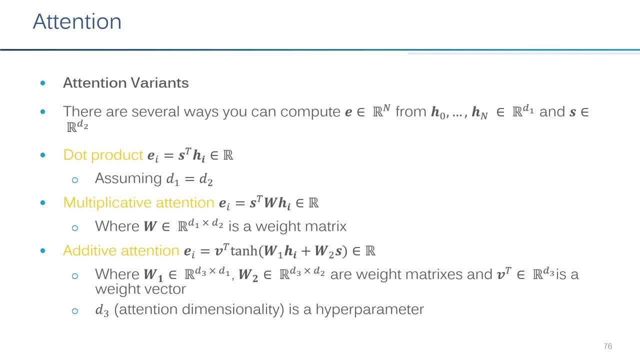 in a way that you also do the dot product between encoder and decoder, but product between encoder and decoder, but product between encoder and decoder, but you introduce a new weight matrix to. you introduce a new weight matrix to, you introduce a new weight matrix to that. that that then, uh, there, there is another approach. 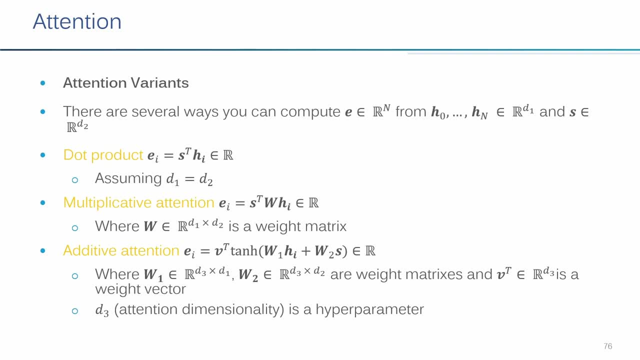 then, uh, there, there is another approach. then, uh, there, there is another approach- i didn't put it here- in which they- i didn't put it here, in which they- i didn't put it here- in which they decompose this weight matrix and decompose this weight matrix and 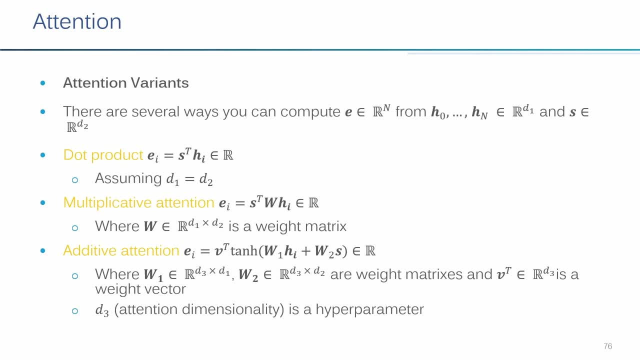 decompose this weight matrix and sub matrix with uh, sub matrix with uh, sub matrix with uh- a smaller dimensionality in a hope to a smaller dimensionality, in a hope to a smaller dimensionality, in a hope to make this here more performatic. because make this here more performatic because 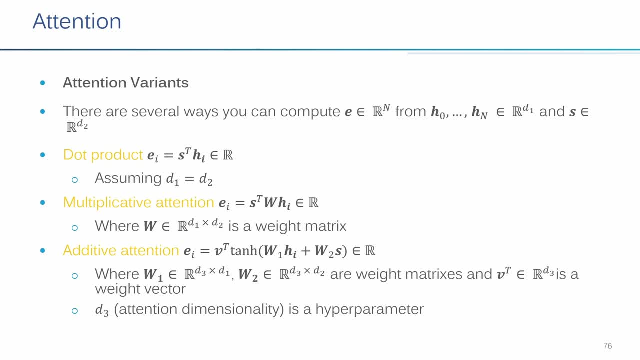 make this here more performatic, because not not all the dimensions, they will not, not all the dimensions, they will not not all the dimensions, they will matter, matter, matter. and this multiplicative attention, uh, then. and this multiplicative attention, uh then. and this multiplicative attention, uh, then. we have also additive attention: uh, in. 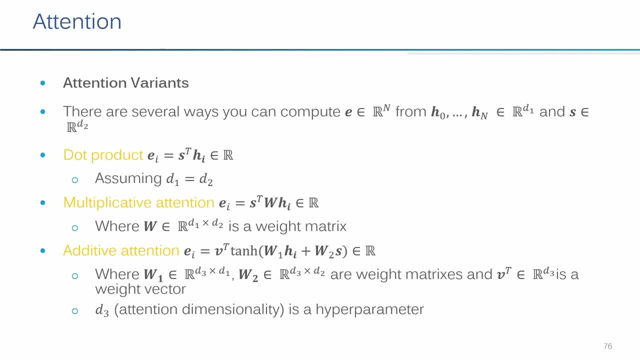 we have also additive attention uh in. we have also additive attention uh in which you multiply, which you multiply, which you multiply for specific weights, your encoder in for specific weights, your encoder in for specific weights, your encoder in your decoder. you put that in a 10 h and 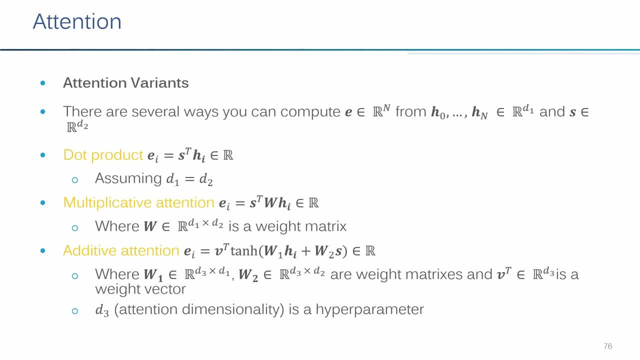 your decoder, you put that in a 10 h, and your decoder, you put that in a 10 h, and then you multiply it by another weight, then you multiply it by another weight, then you multiply it by another weight. vector: vector: vector arbitrarily initialized. then there's other architectures, but 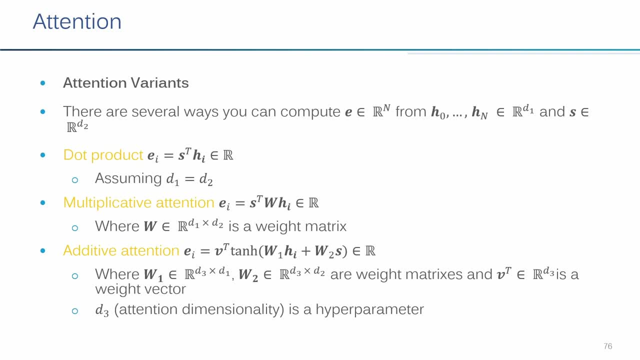 then there's other architectures, but then there's other architectures, but this got more popular in self-attention. this got more popular in self-attention. this got more popular in self-attention in a way that, in a way that, in a way that they discover that there is no need. 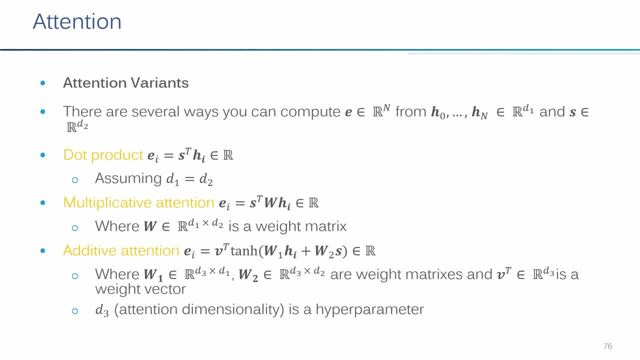 they discover that there is no need. they discover that there is no need, especially if you have larger sequence, especially if you have larger sequence, especially if you have larger sequence, that you have to pay attention, or at that you have to pay attention, or at that you have to pay attention, or at least verify every single word in that. 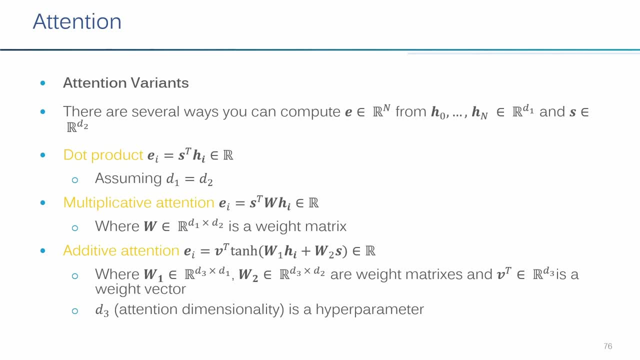 least verify every single word in that least, verify every single word in that context. so they come up with the concept context, so they come up with the concept context. so they come up with the concept of global attention, local attention of global attention, local attention of global attention, local attention, random attention, and so on. 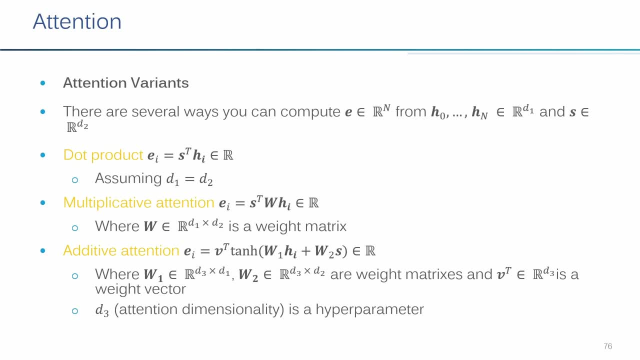 random attention and so on. random attention and so on. uh, but we'll hopefully uh get there. but uh, but we'll hopefully uh get there. but uh, but we'll hopefully uh get there. but think as just improvements, how to think as just improvements, how to think as just improvements, how to relate the encoder and the decoder. that 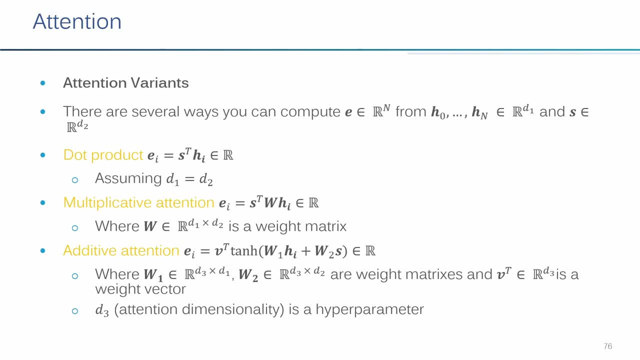 relate the encoder and the decoder. that relate the encoder and the decoder. that you have all right. the, you have all right. the you have all right. the initial idea: it remains the same initial idea. it remains the same initial idea. it remains the same. then uh, then uh. 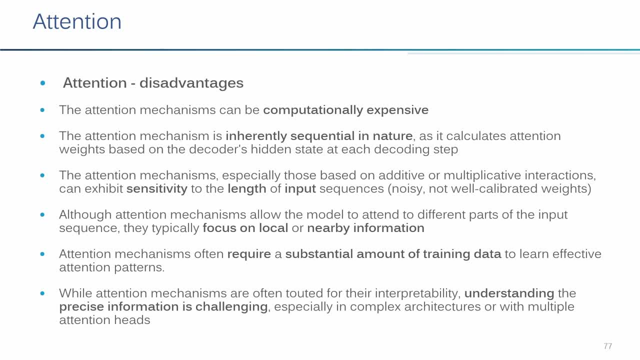 then, uh, you might think yes, you might think yes, you might think yes, we solved the problem between encoder, we solved the problem between encoder, we solved the problem between encoder and decoder and decoder and decoder. but attention technique also has its. but attention technique also has its. but attention technique also has its problems. 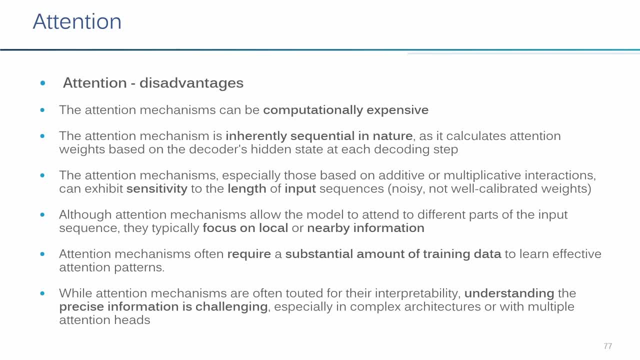 problems, problems first, first, first. it is really expensive to run that. it is really expensive to run that. it is really expensive to run that because you have to make all the, because you have to make all the, because you have to make all the multiplications for every state in your 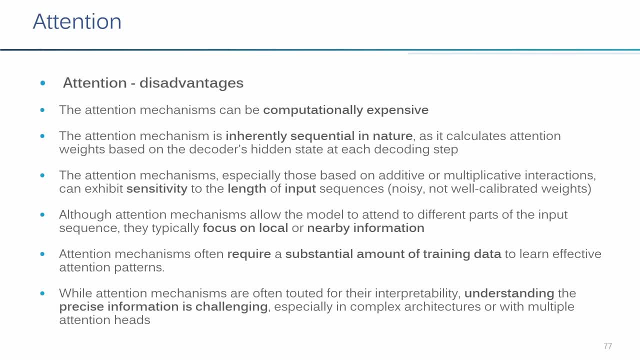 multiplications for every state in your multiplications for every state in your decoder, with all the states that you decoder, with all the states that you decoder, with all the states that you have in your encoder, have in your encoder, have in your encoder this, this, this problem will get worse in self-attention. 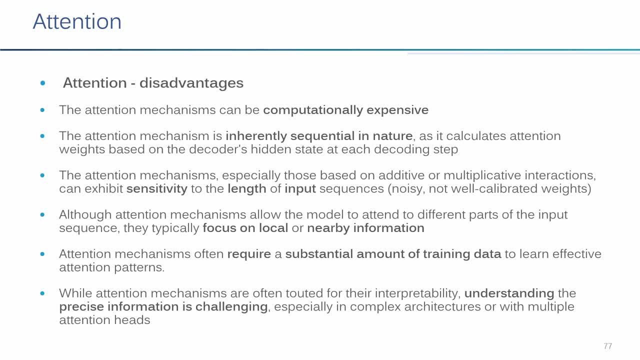 problem will get worse in self-attention problem will get worse in self-attention. the attention mechanism as we see right, the attention mechanism as we see right, the attention mechanism as we see right now is sequential in nature, simply now is sequential in nature. simply now is sequential in nature simply because at the decoder step we have to. 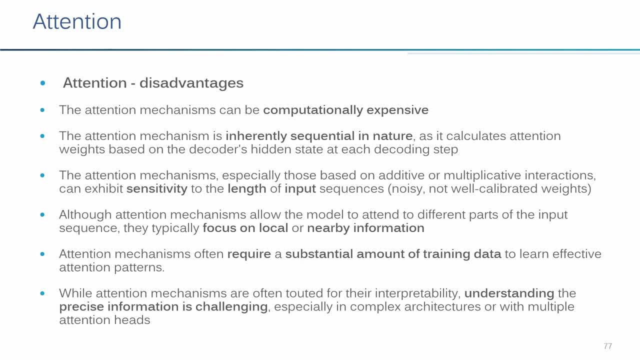 because at the decoder step we have to, because at the decoder step we have to calculate the attention scores for all, calculate the attention scores for all, calculate the attention scores for all those steps over and over again. the attention scores when we are, the attention scores when we are. 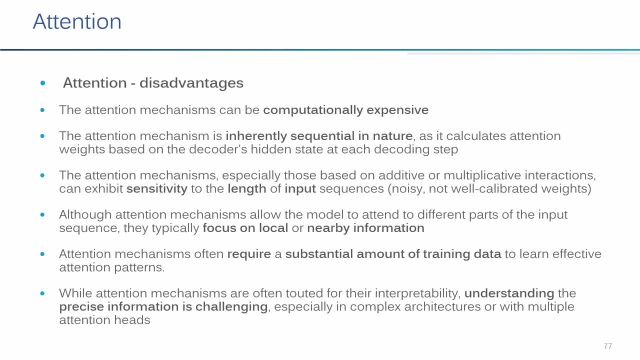 the attention scores when we are multiplying the decoder and the encoder. multiplying the decoder and the encoder, multiplying the decoder and the encoder, especially if you're using additive, and especially if you're using additive, and especially if you're using additive and multiplicative interactions. they are multiplicative interactions. they are 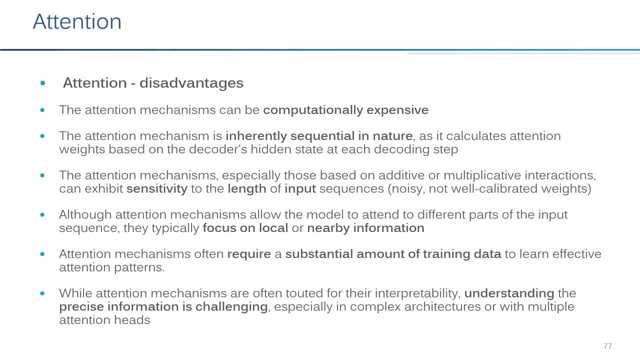 multiplicative interactions. they are sensitive to the length of input. you sensitive to the length of input, you sensitive to the length of input you have. so have, so have. so the larger it is, the harder it gets to, the larger it is, the harder it gets to. the larger it is, the harder it gets to control that, or the less meaningful it. 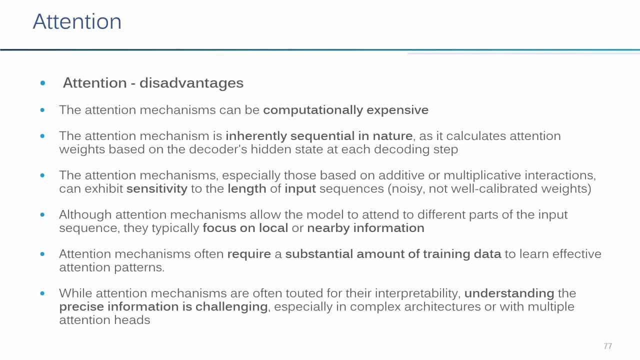 control that or the less meaningful it. control that or the less meaningful it gets at least uh for the weights. gets at least uh for the weights, gets at least uh for the weights. capturing the sequence, capturing the sequence, capturing the sequence also, also also. we saw, we'll see that uh. 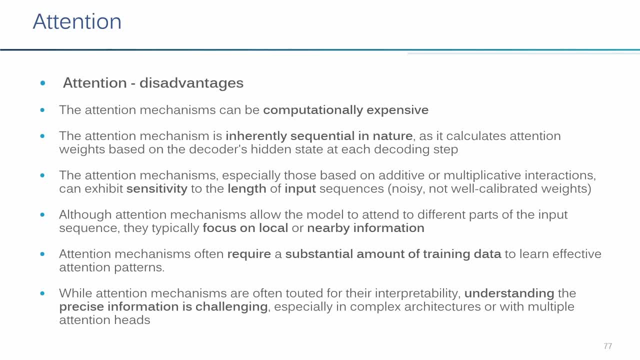 we saw, we'll see that. uh, we saw, we'll see that. uh, although this attention mechanism allows, although this attention mechanism allows, although this attention mechanism allows us to attend to different parts in our us, to attend to different parts in our us, to attend to different parts in our inputs, 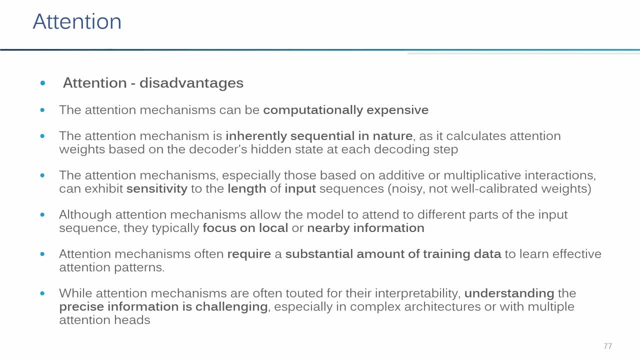 inputs, inputs in practice. we'll see that from the in practice. we'll see that from the in practice we'll see that from the entire sequence, very specific parts are entire sequence. very specific parts are entire sequence. very specific parts are actually relevant for your prediction in actually relevant for your prediction in. 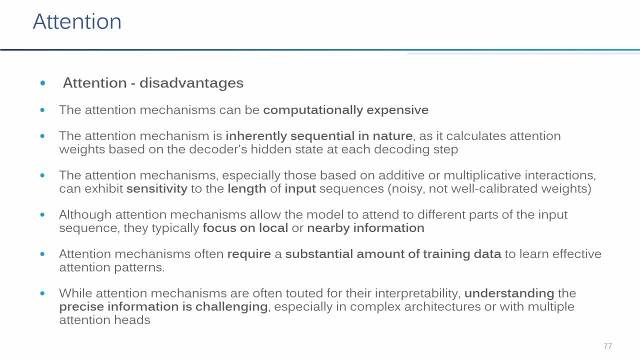 actually relevant for your prediction in the end, which they'll have a really the end, which they'll have a really end, which they'll have a really highest score there, highest score there, highest score there, uh uh, uh. needless to say, and we talk about this, needless to say, and we talk about this, 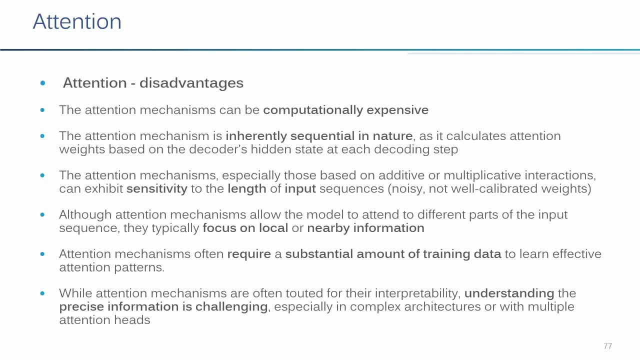 needless to say- and we talk about this already, already, already, we do require a lot of training data, for we do require a lot of training data, for we do require a lot of training data for this technique slash architecture, this technique slash architecture, this technique slash architecture also, and we talk about this on. 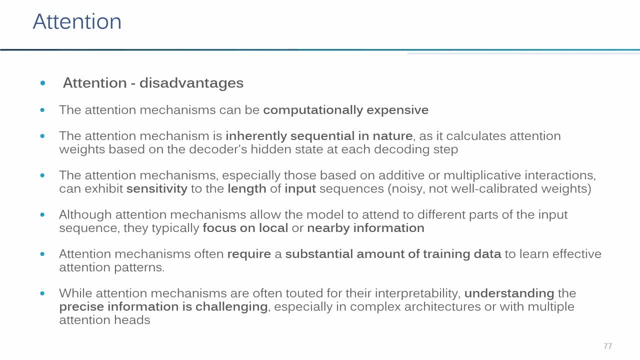 also, and we talk about this on also, and we talk about this on- advantages, although advantages, although advantages, although usually you see attention scores being usually you see attention scores being usually you see attention scores being used as a proxy to understand where, used as a proxy to understand where. 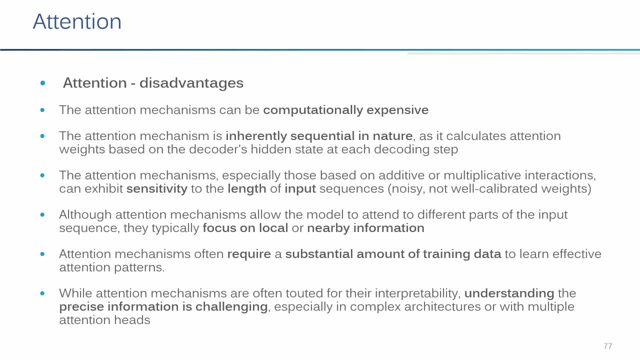 used as a proxy to understand where your model is paying attention. your model is paying attention. your model is paying attention. in practice is not that meaningful. it's in practice is not that meaningful. it's in practice is not that meaningful. it's debatable. yes, you have a distribution of 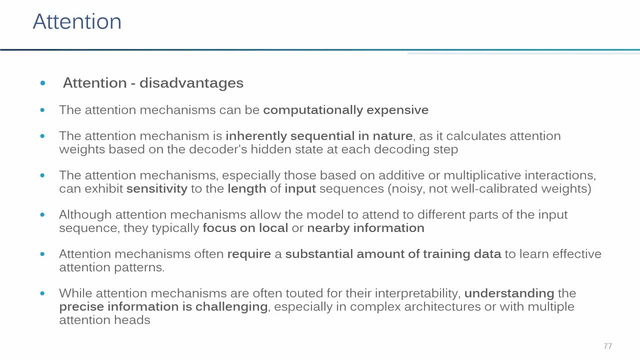 debatable. yes, you have a distribution of debatable. yes, you have a distribution of high scores for whatever parts that you high scores for, whatever parts that you high scores for, whatever parts that you have in your sentence, but what actually have in your sentence, but what actually? 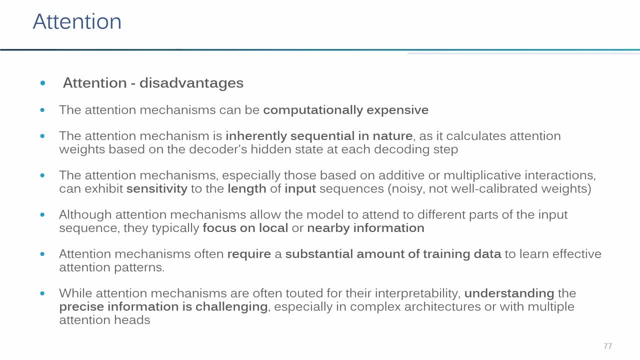 have in your sentence, but what actually that means? that means that means it's debatable in a sense. that is it. it's debatable in a sense. that is it. it's debatable in a sense. that is it really showing to me that this, really showing to me that this? 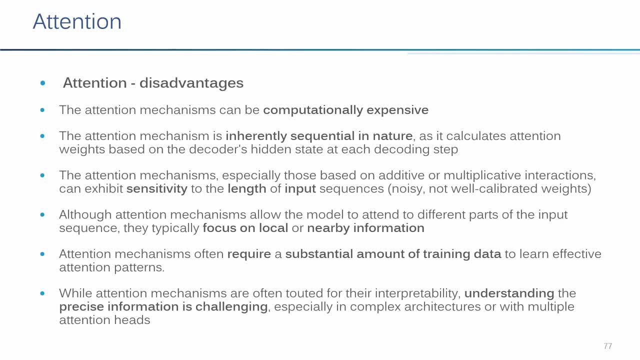 really showing to me that this relationship between two words are simply relationship between two words, are simply relationship between two words, are simply represented because i have a higher represented, because i have a higher represented because i have a higher score between those two parts, score between those two parts. 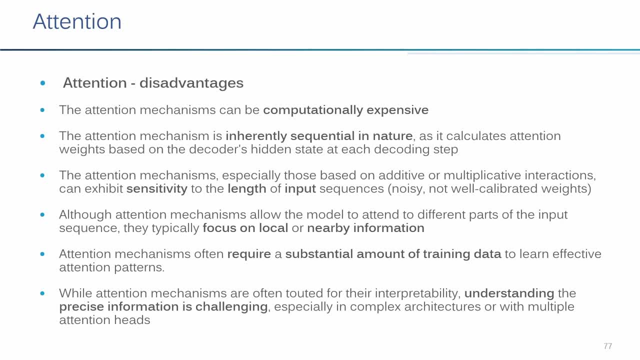 score between those two parts. um, um, um, think as, and i'm really think as, and i'm really think as, and i'm really going far on this comparison. how many of going far on this comparison? how many of going far on this comparison? how many of you already were looking to word clouds? 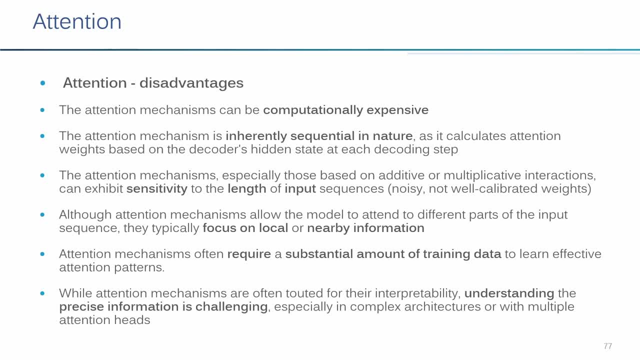 you already were looking to word clouds. you already were looking to word clouds. everyone loves to do word clouds. what do everyone loves to do word clouds? what do everyone loves to do word clouds? what do they mean? they mean, they mean. yeah, you have a blob of words, some words. 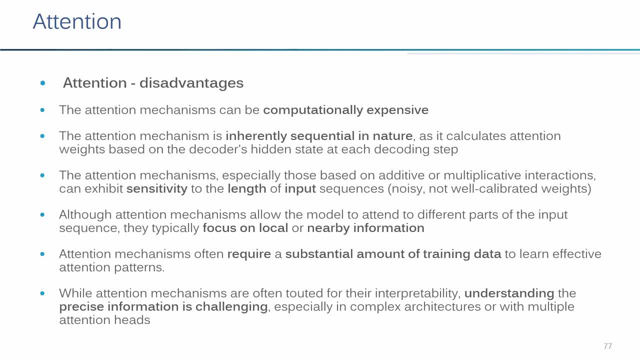 yeah, you have a blob of words. some words, yeah, you have a blob of words. some words are bigger, smaller, but are bigger, smaller, but are bigger, smaller. but yeah, it looks nice in the website. but if, yeah, it looks nice in the website. but if, yeah, it looks nice in the website. but if you want to make your points like 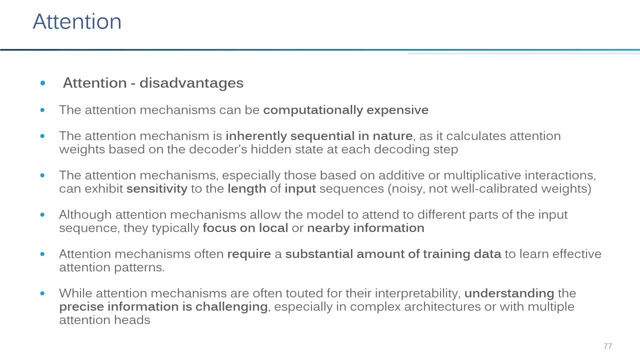 you want to make your points like. you want to make your points like: yeah, it doesn't mean much. yeah, it doesn't mean much. yeah, it doesn't mean much. what usually it's going to happen? is you what usually it's going to happen? is you what usually it's going to happen? is you see papers with fancy heat maps to show? 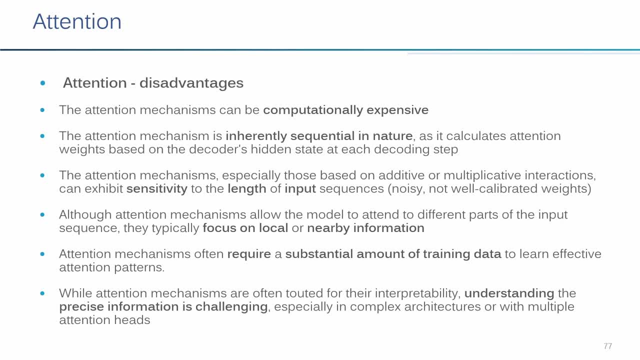 see papers with fancy heat maps to show. see papers with fancy heat maps to show how the attention is changing over the, how the attention is changing over the, how the attention is changing over the layers, layers, layers. yes, it gives you a good hint to okay if. yes, it gives you a good hint to okay if. 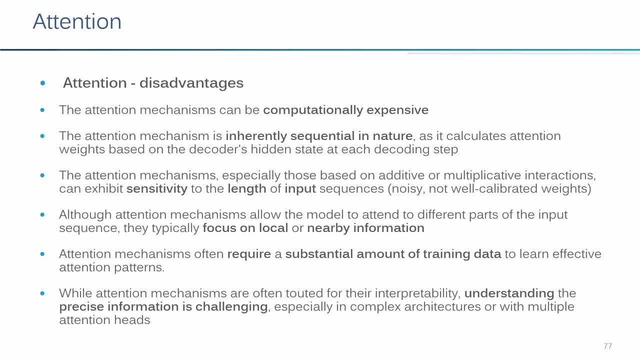 yes, it gives you a good hint to: okay, if the model, the sequence are not pay the model, the sequence are not pay the model, the sequence are not pay attention to specific attention to specific attention to specific sequences, maybe that's not that relevant sequences. maybe that's not that relevant. 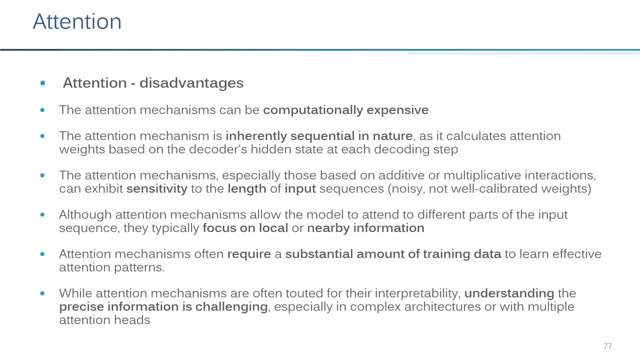 sequences. maybe that's not that relevant. yes, but don't base your entire yes, but don't base your entire yes, but don't base your entire discussion simply because discussion, simply because discussion, simply because you have a fancy heat map to illustrate. you have a fancy heat map to illustrate. 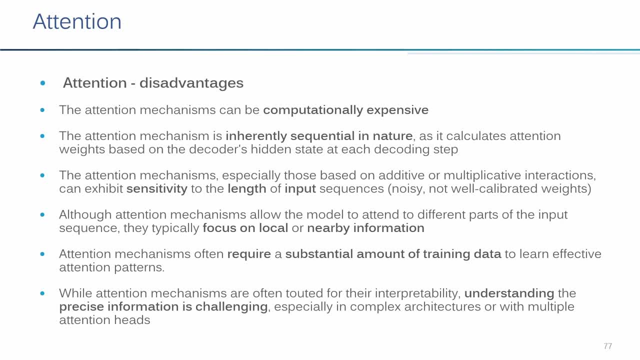 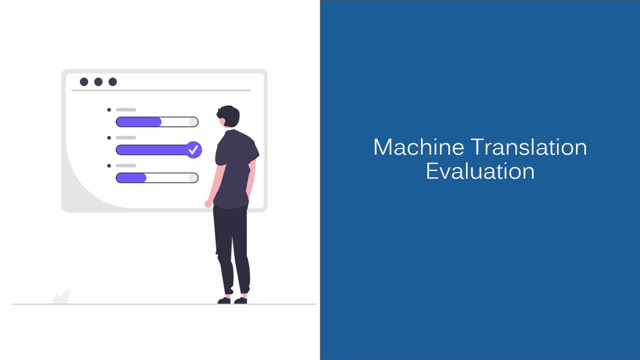 you have a fancy heat map to illustrate: uh, these attentions, uh, these attentions, uh, these attentions, scores okay and scores okay and scores okay. and before we move forward, if you remember the beginning of the, if you remember the beginning of the, if you remember the beginning of the class, we talk about how machine 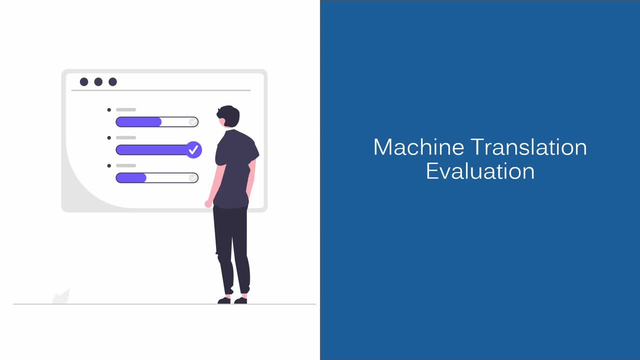 class. we talk about how machine class. we talk about how machine translation translation. translation is problematic, not because it's hard is problematic, not because it's hard is problematic, not because it's hard to capture all the semantic difference. to capture all the semantic difference, to capture all the semantic difference between: 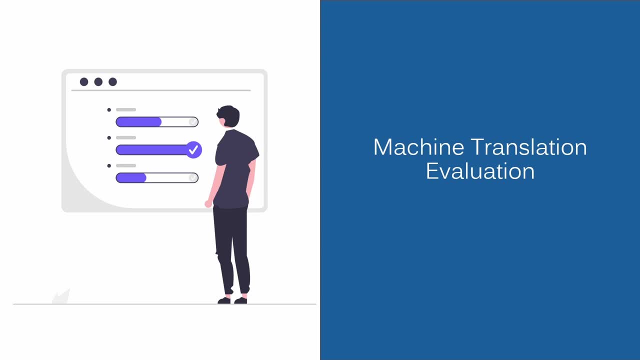 between between input and output or source and target input and output or source and target input and output or source and target sequences, but also about the evaluation sequences, but also about the evaluation sequences, but also about the evaluation, and this is valid for pretty much, and this is valid for pretty much. 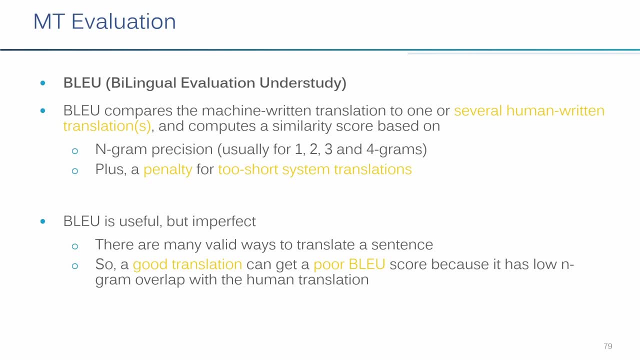 and this is valid for pretty much any task that involves generation of any task that involves generation of any task that involves generation of text. they are based on very specific text, they are based on very specific text, they are based on very specific metrics: metrics, metrics. everyone know that they suck, but they. 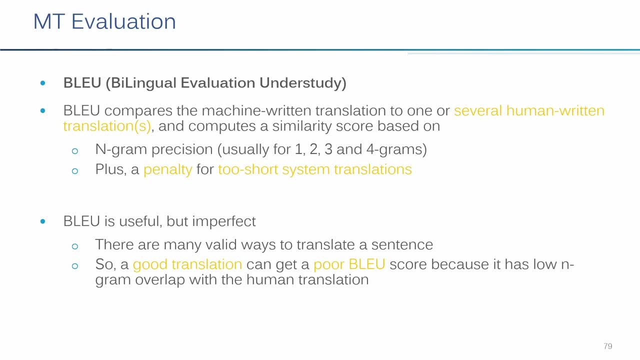 everyone know that they suck, but they- everyone know that they suck, but they still use them, still use them, still use them. there are better metrics nowadays that there are better metrics nowadays that. there are better metrics nowadays that they try to grasp, they try to grasp, they try to grasp. okay, how faithful one translation is. or 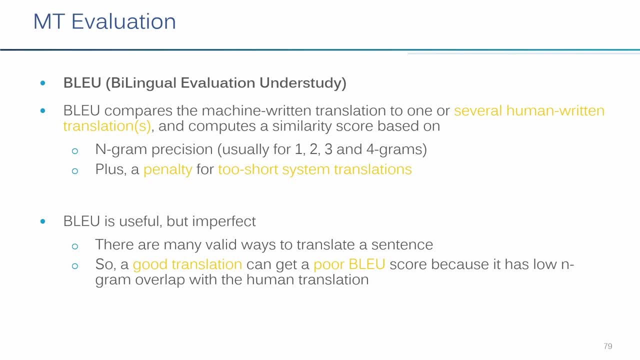 okay how faithful one translation is, or okay how faithful one translation is or how it conveys a specific meaning, but in practice if you have those, but in practice if you have those, but in practice if you have those systems and you don't validate with systems and you don't validate with. 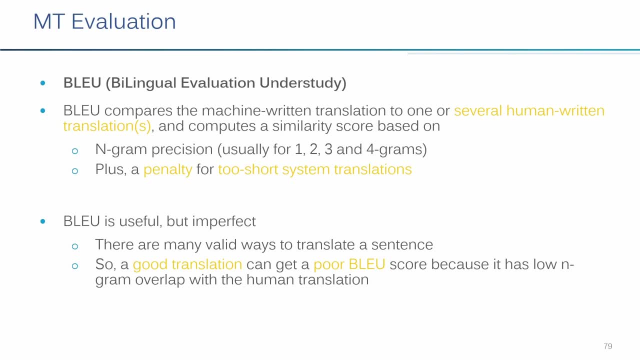 systems and you don't validate with people. it can have the highest score, you people. it can have the highest score, you people. it can have the highest score. you can think of it, can think of it, can think of it, if it's not a good translation people. 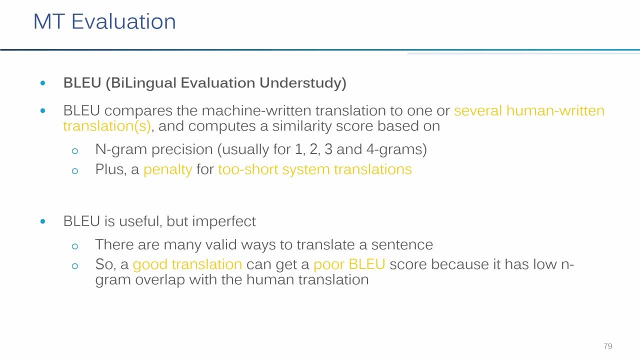 if it's not a good translation, people, if it's not a good translation, people will not use it. it's not reliable as will not use it. it's not reliable as will not use it. it's not reliable. as simple as this. simple as this, simple as this. so, for those thinking about working with 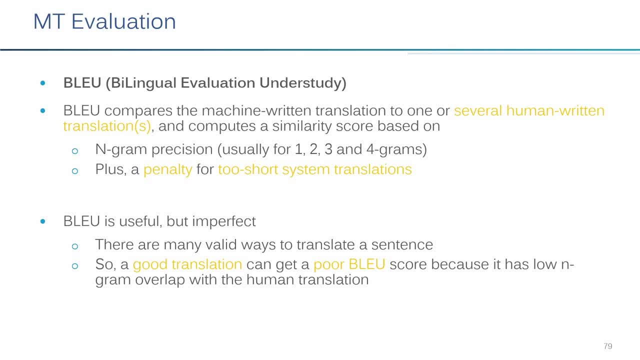 so for those thinking about working with, so, for those thinking about working with, uh, to always have a qualitative analysis. uh, to always have a qualitative analysis. uh, to always have a qualitative analysis in whatever experiment that you have to, in whatever experiment that you have to, in whatever experiment that you have to miss, to at least validate if. 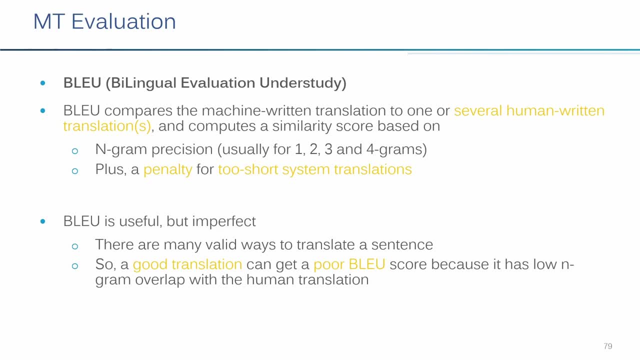 miss to at least validate, if miss to at least validate if, uh, it's indeed working for humans. so, uh, it's indeed working for humans. so, uh, it's indeed working for humans. so, that being said, this huge caveat we have. that being said, this huge caveat we have. 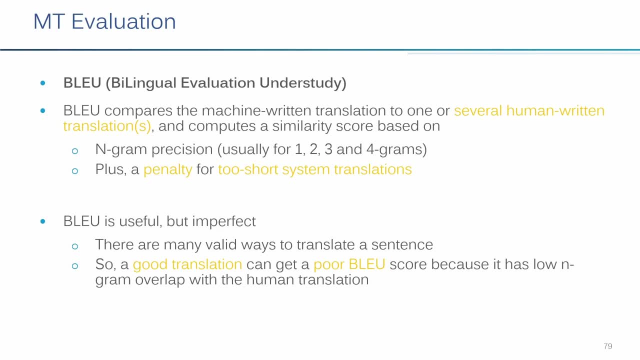 that being said, this huge caveat, we have to take a look on those, to take a look on those, to take a look on those: uh, automatic metrics. simply because, uh, automatic metrics. simply because, uh, automatic metrics. simply because people still compare with them, but keep, people still compare with them, but keep. 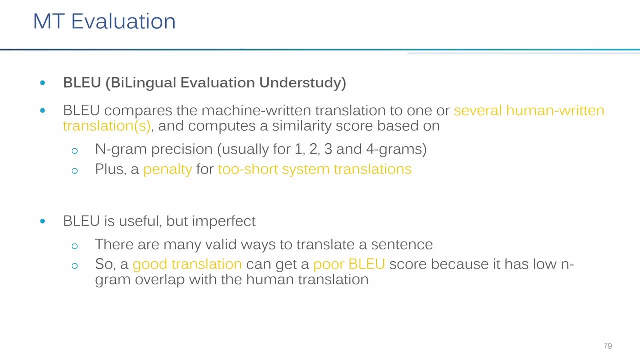 people still compare with them. but keep in mind, that's not the best practice in mind. that's not the best practice in mind. that's not the best practice proxy. so we have blue right here. which proxy. so we have blue right here. which proxy. so we have blue right here, which is pretty much. we're gonna take a look. 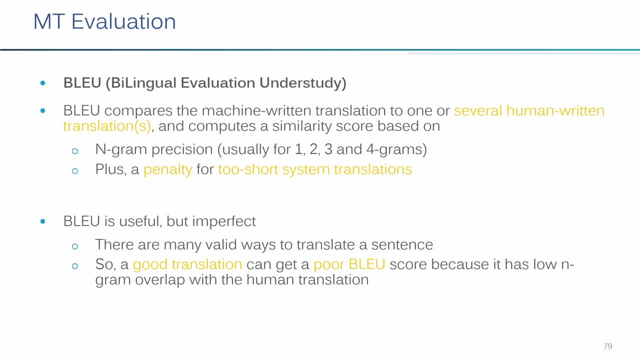 is pretty much we're gonna take a look is pretty much we're gonna take a look, uh, on the translation that we have with uh, on the translation that we have with uh, on the translation that we have with some references and this translation is some references and this translation is. 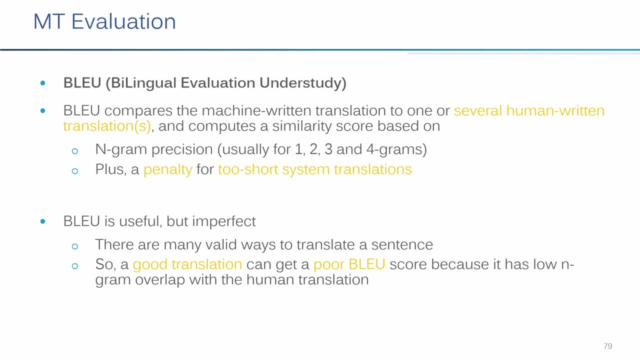 some references, and this translation is usually done by human, which is also usually done by human, which is also usually done by human, which is also debatable, if human is actually the best debatable, if human is actually the best debatable, if human is actually the best gold standard. 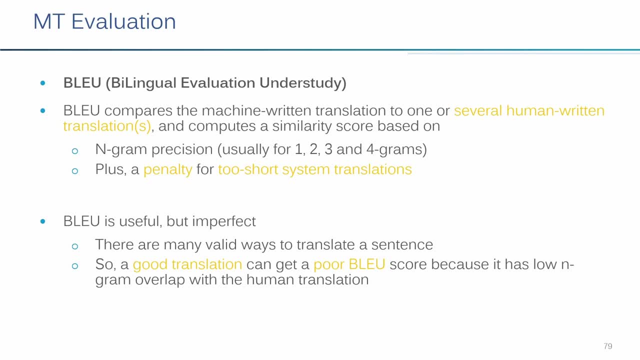 gold standard- gold standard- uh spoiler alert. not always there's uh spoiler alert. not always there's uh spoiler alert. not always there's papers on this, and i should include this papers on this, and i should include this papers on this and i should include this. i'll make a. 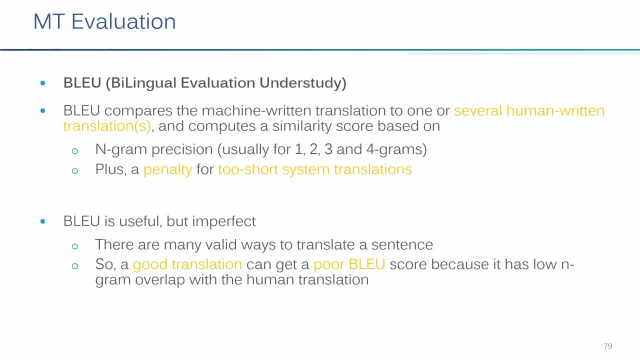 i'll make a, i'll make a reminder for me, reminder for me, reminder for me: um, um, um and then, and then, and then. okay, but how we calculate that? let's take okay, but how we calculate that, let's take. okay, but how we calculate that? let's take a look. 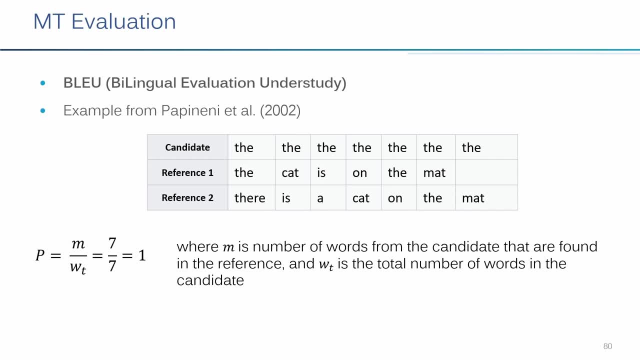 a look, a look. so pretty much, so, pretty much, so, pretty much. we calculate the precision, we calculate the precision, we calculate the precision between m and wt. right here, where m is between m and wt, right here where m is between m and wt, right here where m is the number of words for our candidate. 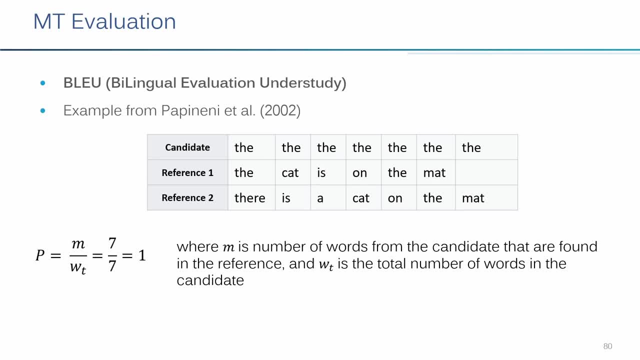 the number of words for our candidate, the number of words for our candidate, and this here is our sequence that we are, and this here is our sequence that we are, and this here is our sequence that we are, providing that we're machining, providing that we're machining. 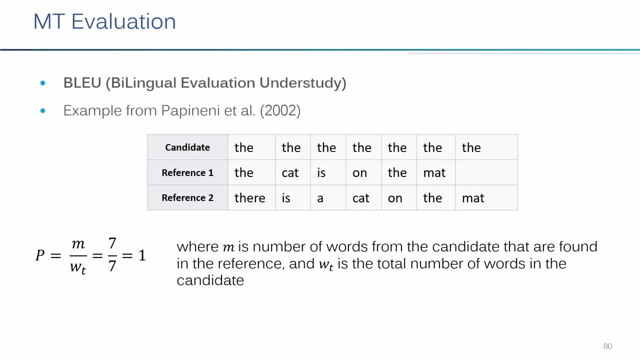 providing that we're machining machine- uh translating- with some machine, uh translating with some machine, uh translating with some reference that we have right here. so reference that we have right here, so reference that we have right here. so we divide the number of words, uh that. we divide the number of words, uh that. 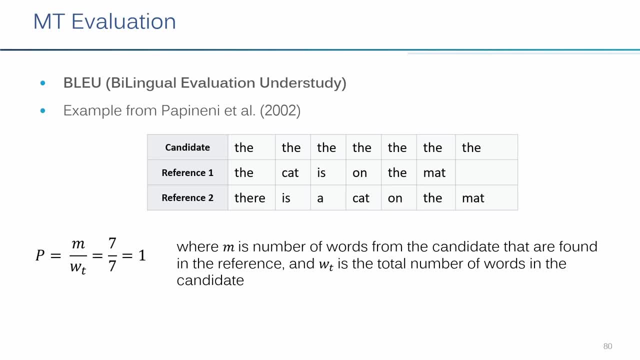 we divide the number of words, uh that from our candidate appear in our. from our candidate appear in our, from our candidate appear in our reference reference, reference divided by the total number of words, divided by the total number of words, divided by the total number of words that we have in our candidate, and this 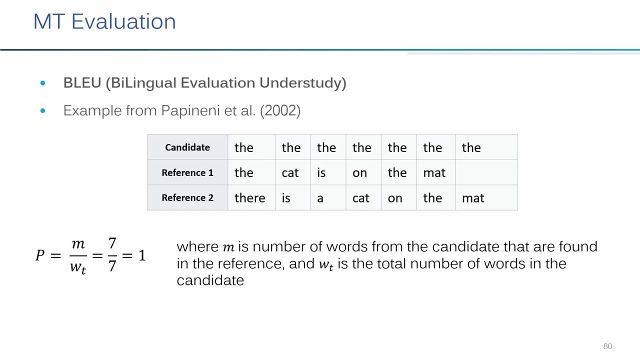 that we have in our candidate and this that we have in our candidate- and this is a really good example- is a really good example, is a really good example how a metric can mislead you in this, how a metric can mislead you in this, how a metric can mislead you in this case. right here we have a candidate. 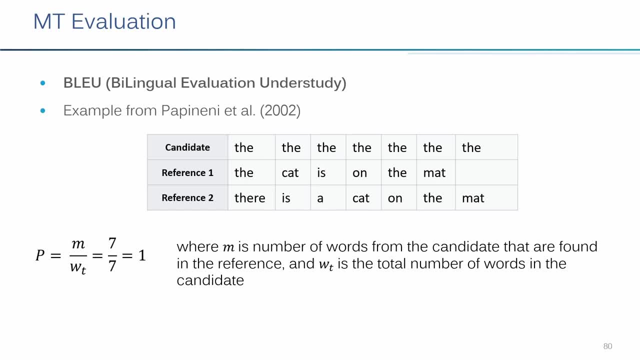 case. right here we have a candidate case, right here we have a candidate, and then, and then, and then, uh, by taking into account uh uh, by taking into account uh uh, by taking into account, uh, our reference and how many words from our, our reference, and how many words from our. 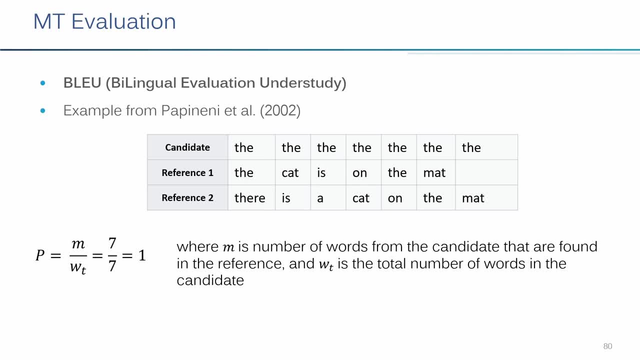 our reference and how many words from our candidate appeared in our reference candidate appeared in our reference candidate appeared in our reference. we get a score of 100 on this translation. we get a score of 100 on this translation. we get a score of 100 on this translation- awesome, right. 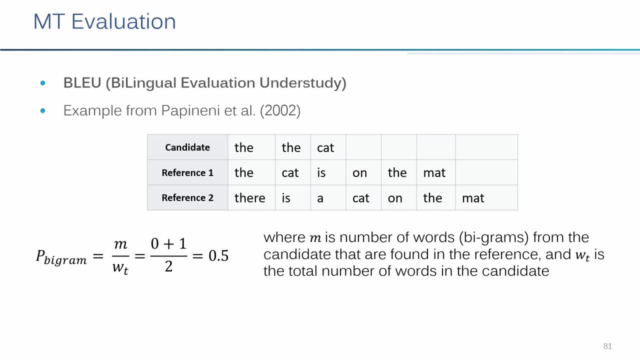 awesome right, awesome right. uh, not really. there is modifications on the blue score. there is modifications on the blue score. there is modifications on the blue score in which you can have biograms, in which you can have biograms, in which you can have biograms, trigrams, four grams, and so on, and so 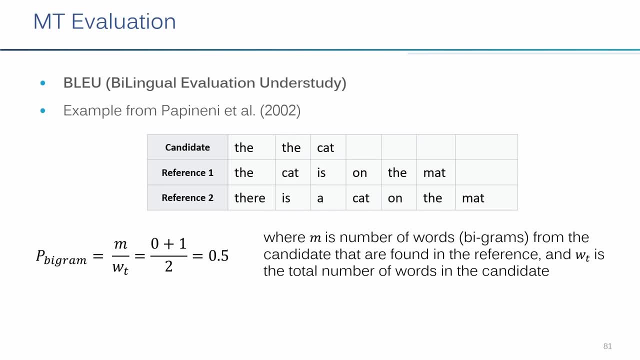 trigrams, four grams, and so on, and so trigrams, four grams, and so on and so forth, but they all suffer from kind of forth, but they all suffer from kind of forth, but they all suffer from kind of the same problem, the same problem, the same problem, uh, in a way that, in this case, right here, 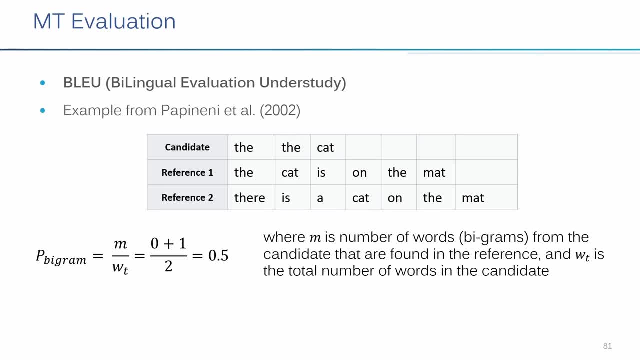 uh, in a way that in this case, right here, uh, in a way that in this case, right here, we are considering all the biograms, we are considering all the biograms, we are considering all the biograms, uh, that we have in our candidate with, uh, that we have in our candidate with. 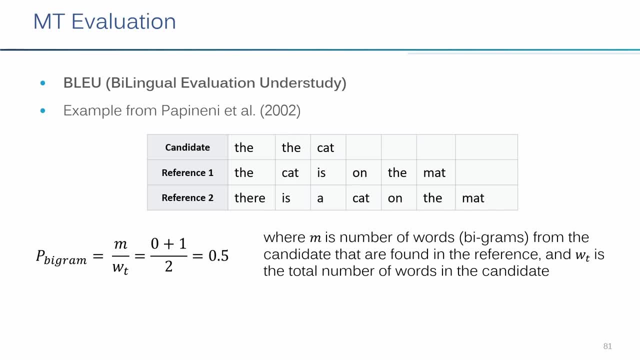 uh that we have in our candidate with respect to our reference. so, in this case, respect to our reference. so, in this case, respect to our reference. so in this case, uh, we have the, uh, we have the, uh, we have the. and, of course, this never appeared in our 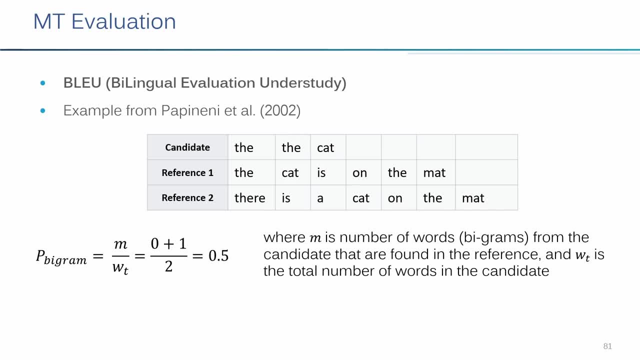 and of course, this never appeared in our and of course this never appeared in our reference and the cat reference and the cat reference and the cat appeared in this year. we're using the appeared in this year. we're using the appeared in this year. we're using the first reference as a, as a reference. 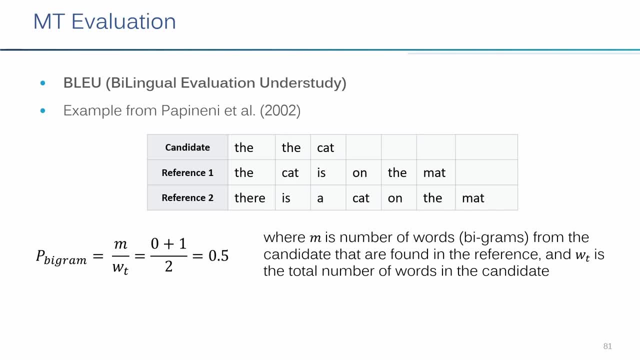 first reference as a as a reference, first reference as a as a reference, and then we see here that the score is, and then we see here that the score is, and then we see here that the score is still 50, which is pretty high, still 50, which is pretty high. 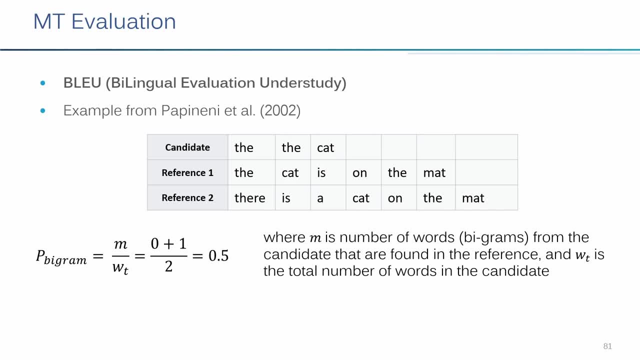 still 50, which is pretty high. uh, if you ask me needless to say uh, uh. if you ask me needless to say uh, uh. if you ask me needless to say uh. this here can generate some problems. this here can generate some problems. this here can generate some problems, especially when you trans, when you're. 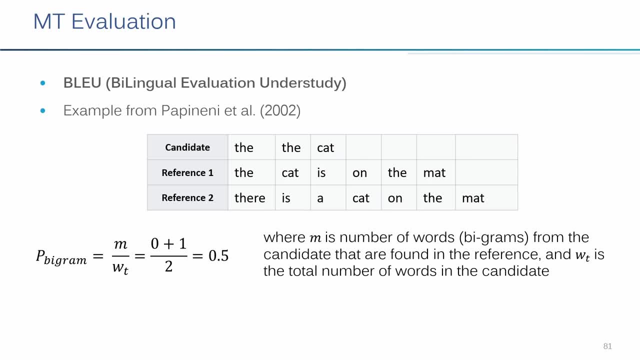 especially when you trans, when you're, especially when you trans, when you're using a system that's not that easy for using a system that's not that easy for using a system that's not that easy for you to track those errors and you're you to track those errors and you're. 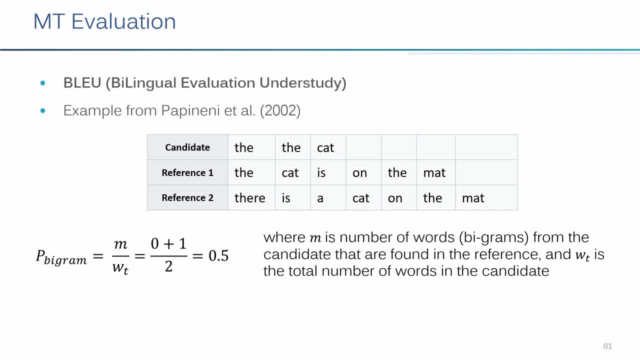 you to track those errors and you're relying on this automatic measure to relying on this automatic measure, to relying on this automatic measure to take a look on how good your take a look on how good your take a look on how good your translation is. translation is. 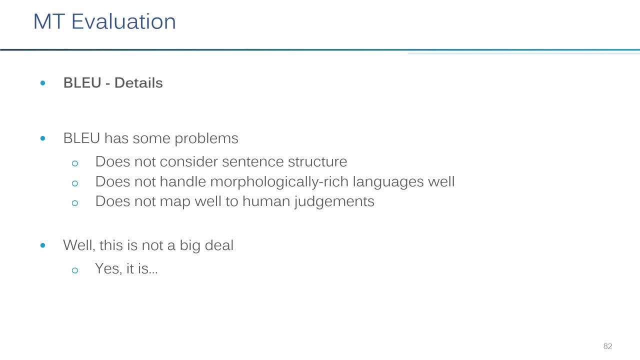 translation is: uh, uh, uh. as we saw, blue has some problems aside. as we saw, blue has some problems aside. as we saw, blue has some problems aside from the metric not being a faithful from the metric not being a faithful from the metric not being a faithful proxy. 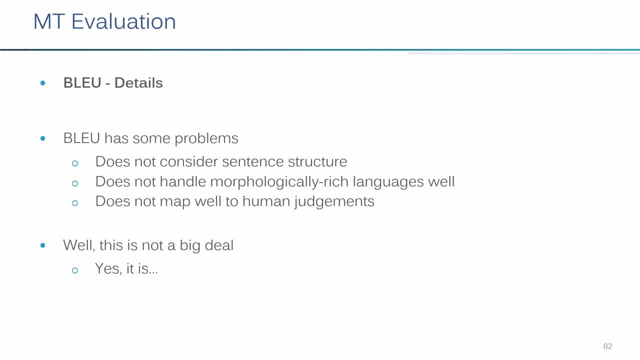 proxy, proxy. in this case, specifically, translation. in this case, specifically translation. in this case, specifically, translation is not that simple. how many times you is not that simple? how many times you is not that simple? how many times you had to translate something from german, had to translate something from german? 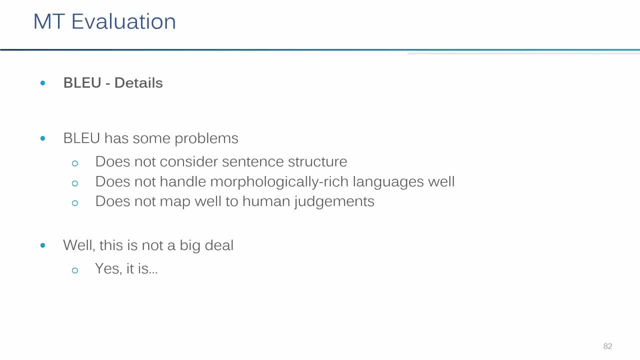 had to translate something from german to english. you simply say nah, there's to english. you simply say nah, there's to english. you simply say nah, there's not a direct translation to this. so not a direct translation to this, so not a direct translation to this. so imagine for you to code that into an. 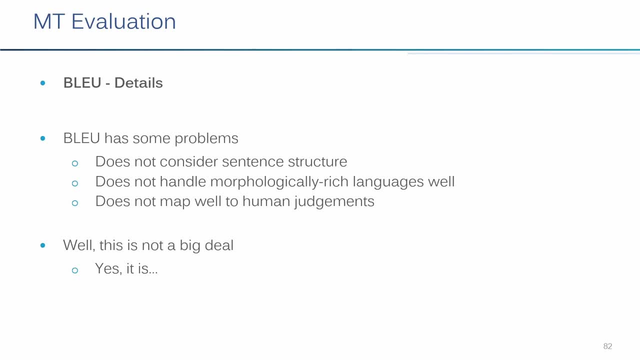 imagine for you to code that into an. imagine for you to code that into an automatic metric, automatic metric, automatic metric: um, um, um. yes, so you'll see this virtually in every. yes, so you'll see this virtually in every. yes, so you'll see this virtually in every single paper using this kind of metric. 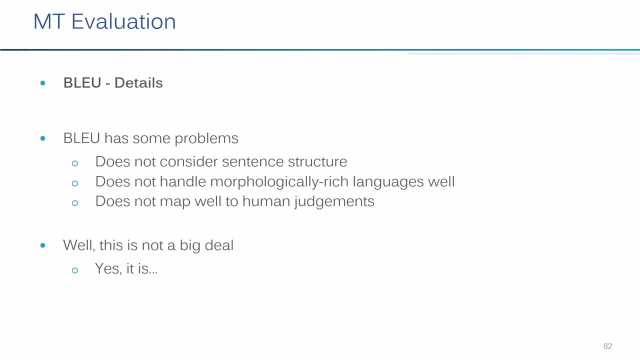 single paper using this kind of metric, single paper, using this kind of metric, and you might think, well, okay, it's not a. and you might think, well, okay, it's not a. and you might think, well, okay, it's not a big deal, it's just a score for sentence. 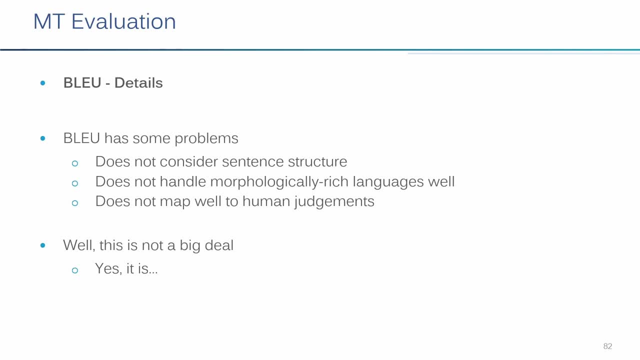 big deal, it's just a score for sentence. big deal, it's just a score for sentence. the thing is the moment that you have. the thing is the moment that you have, the thing is the moment that you have those automatic translations doing by, those automatic translations doing by. 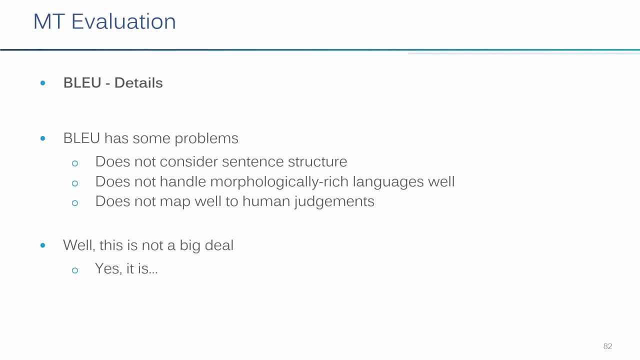 those automatic translations doing by the systems you have to score. what is the systems you have to score? what is the systems you have to score? what is the most probable uh sequence, the most probable uh sequence, the most probable uh sequence, and stuff like this happened and stuff like this happened. 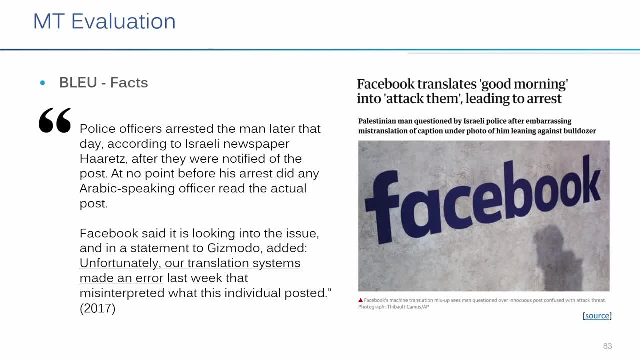 and stuff like this happened. so this was in 2017, so this was in 2017, so this was in 2017. uh, that facebook translates good morning. uh, that facebook translates good morning. uh, that facebook translates good morning into attack them, leading to actual, into attack them, leading to actual. 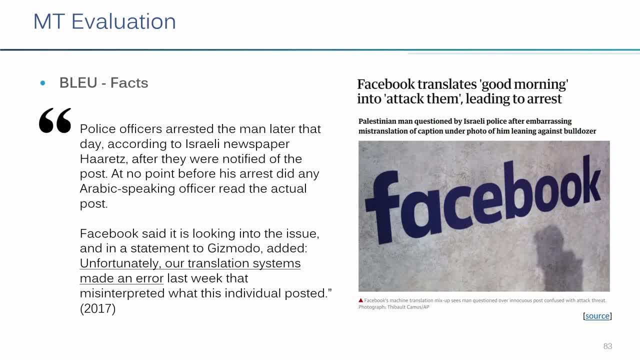 into attack them, leading to actual arrests and, needless to say, this is arrests and, needless to say, this is arrests and, needless to say, this is quite problematic, quite problematic, quite problematic. so just just an excerpt from this news. so just just an excerpt from this news. so just just an excerpt from this news. so polis police officers arrested the. 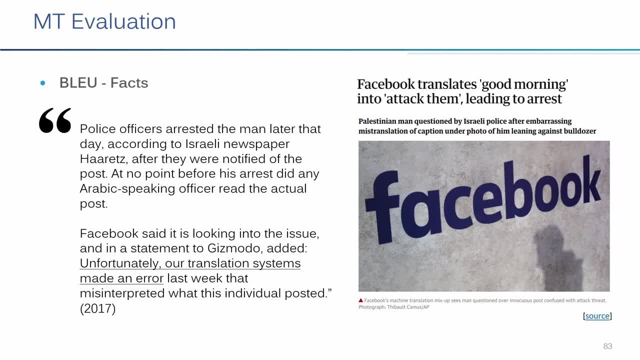 so polis police officers arrested the. so polis police officers arrested the man. later that they according to israeli man, later that they according to israeli man, later that they according to israeli newspaper, after they were notified of newspaper, after they were notified of. 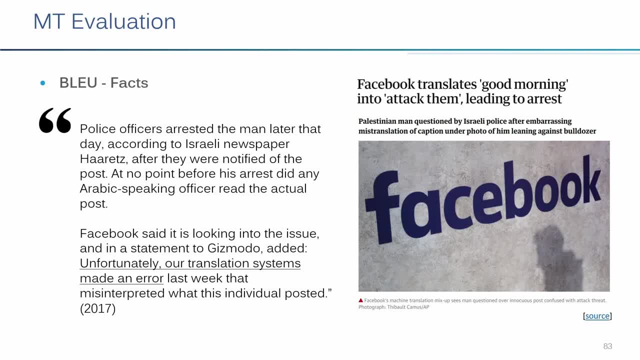 newspaper after they were notified of the post at no point before his arrest. the post at no point before his arrest. the post: at no point before his arrest. did any arab speaking officer read the? did any arab speaking officer read the? did any arab speaking officer read the actual posts? this is, by the way, is. 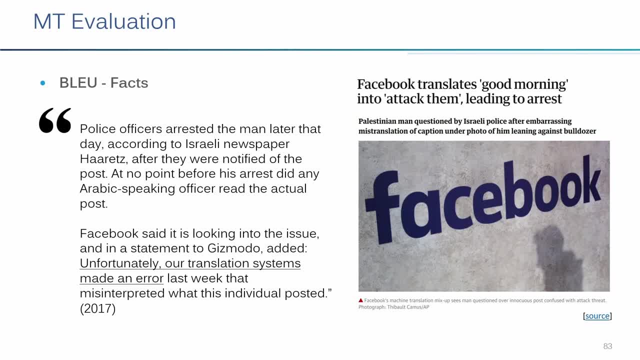 actual posts. this is, by the way, is actual posts. this is, by the way, is automation bias in a way that you simply automation bias, in a way that you simply automation bias, in a way that you simply agree whatever automatic score output, agree whatever automatic score output, agree whatever automatic score output you have. because you say: well, 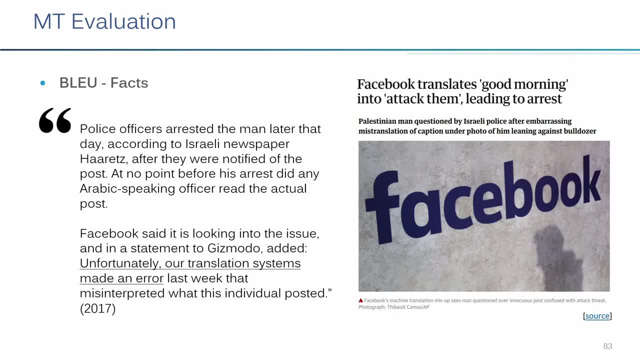 you have because you say well, you have because you say: well, that is generated must be true. right, it's that is generated must be true. right it's that is generated must be true. right, it's on the internet. it must be true, so it's on the internet. it must be true, so it's. 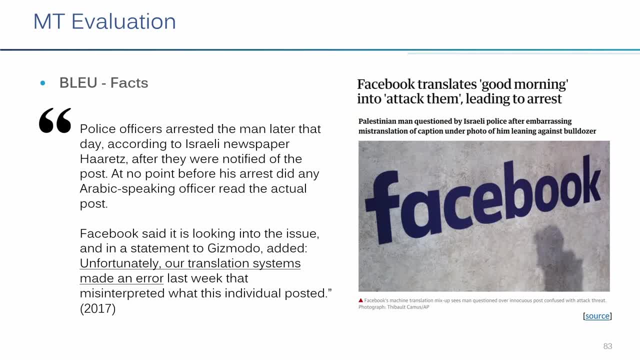 on the internet, it must be true. so it's pretty much the same idea, pretty much the same idea, pretty much the same idea. uh, and of course they took care of the uh and of course they took care of the uh and of course they took care of the matter. but you can see how this can be a. 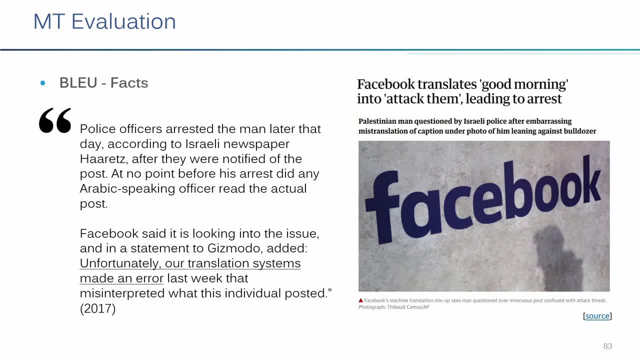 matter, but you can see how this can be a matter, but you can see how this can be a problem, problem, problem, all right, all right, all right, and then you might think okay, and then you might think okay, and then you might think okay, the metric is, the metric is. 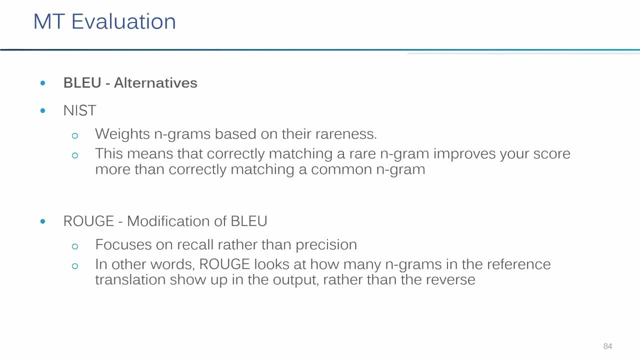 the metric is pretty much terrible what we do. pretty much terrible what we do, pretty much terrible what we do. there are other alternatives. so usually there are other alternatives. so usually there are other alternatives. so usually, when you're working with either machine, when you're working with either machine, 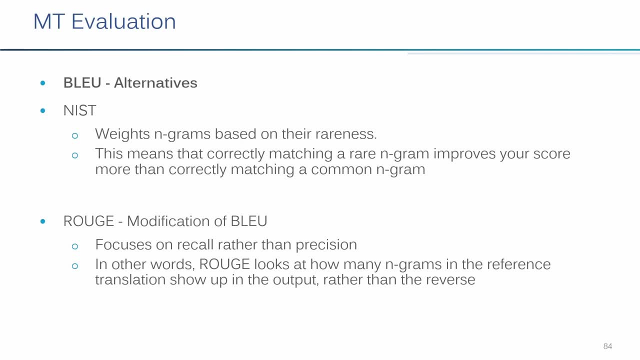 when you're working with either machine translation or again translation, or again translation or again text generation. you have a bunch of text generation. you have a bunch of text generation. you have a bunch of metrics being used, metrics being used, metrics being used- blue, nist, rouge, meteor f1. now you have 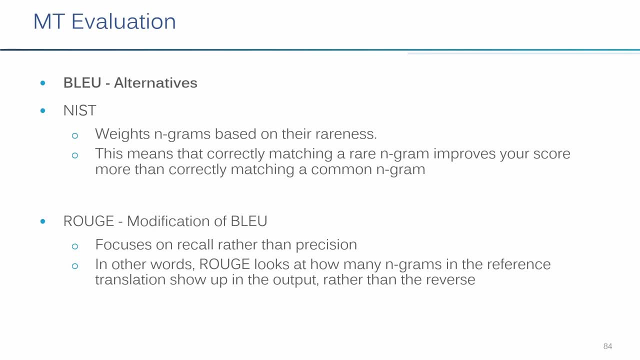 blue nist rouge meteor f1. now you have blue nist rouge meteor f1. now you have kind of a bird score and bart score, kind of a bird score, and bart score kind of a bird score and bart score, which it's kind of a way to introduce. 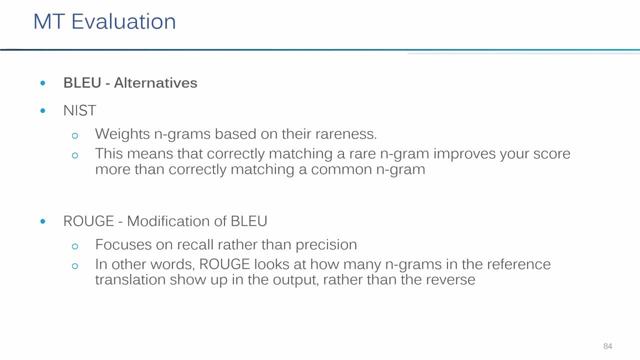 which it's kind of a way to introduce, which it's kind of a way to introduce cosine similarity to those measures, cosine similarity to those measures, cosine similarity to those measures. they do work to some extension, but they do work to some extension, but they do work to some extension, but still they're far from perfect. 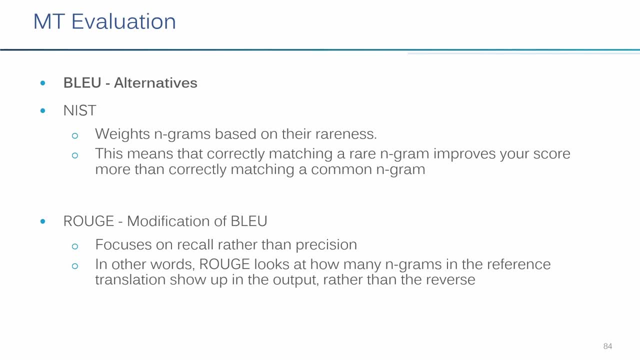 still, they're far from perfect. still, they're far from perfect. we have, we have, we have. nist, it's a national institute for nist. it's a national institute for nist. it's a national institute for statistic technology. it's the same name. statistic technology: it's the same name. 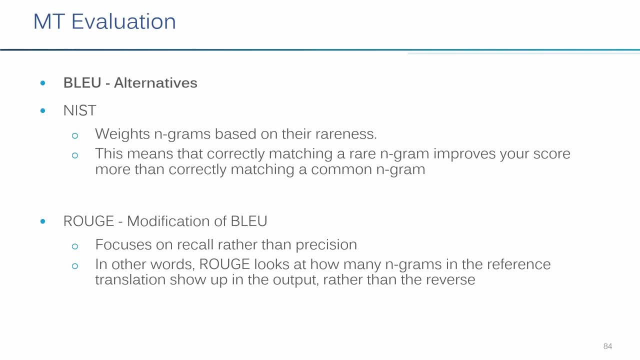 statistic technology. it's the same name as the institute in the us. as the institute in the us, as the institute in the us. we have rouge, which is a modification of. we have rouge, which is a modification of. we have rouge, which is a modification of blue. instead, instead of taking care, 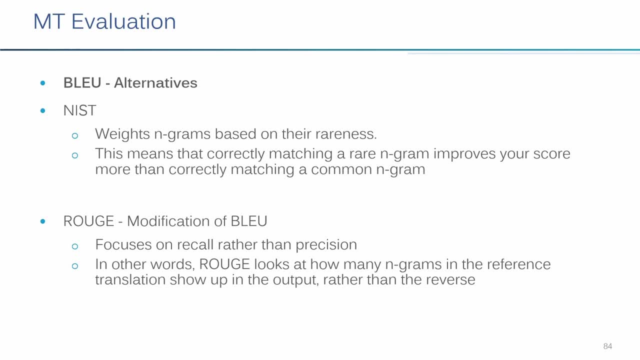 instead, instead of taking care, instead, instead of taking care, instead of looking to the enneagrams in, instead of looking to the enneagrams in, instead of looking to the enneagrams in the reference translation, the reference translation, the reference translation. uh, you look, sorry, in the reference. 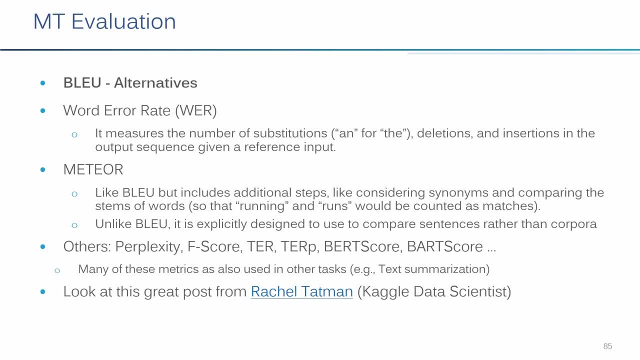 uh, you look sorry in the reference. uh, you look sorry in the reference. translation instead of the other way translation, instead of the other way translation, instead of the other way around, as we did for blue around, as we did for blue around, as we did for blue. by the way, we will revisit those metrics. 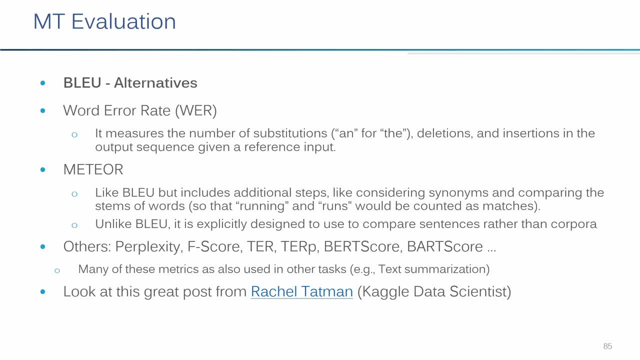 by the way, we will revisit those metrics. by the way, we will revisit those metrics when you talk on um, when you talk on um, when you talk on um text generation in the lecture, with text generation in the lecture, with text generation in the lecture with frederick there. 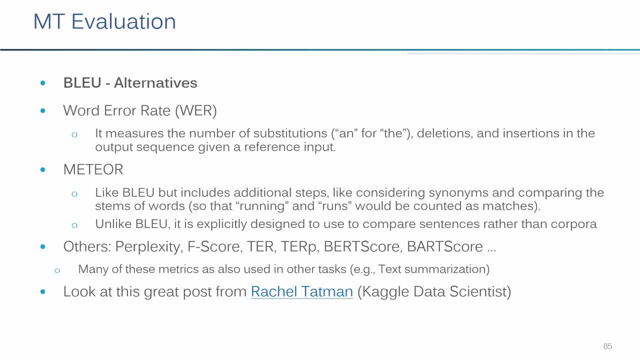 frederick there. frederick there, he uses more. uh, it's called rouge one. he uses more. uh, it's called rouge one. he uses more. uh, it's called rouge one. two, three, l for the longest sequence. two, three, l for the longest sequence. two, three, l for the longest sequence. large score: bird score. we'll take a look. 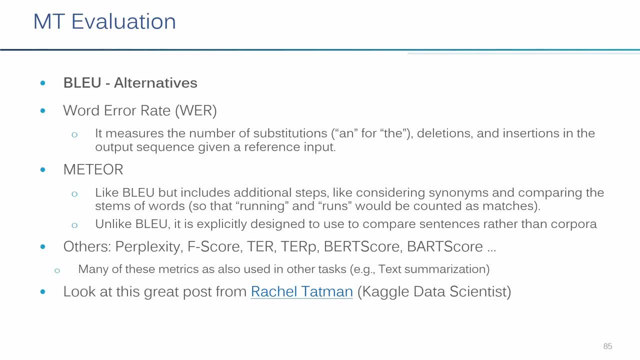 large score- bird score. we'll take a look. large score- bird score. we'll take a look on this later on this, later on this later. uh, we also have word error rate which. uh, we also have word error rate which- uh, we also have word error rate which accounts for substitutions. 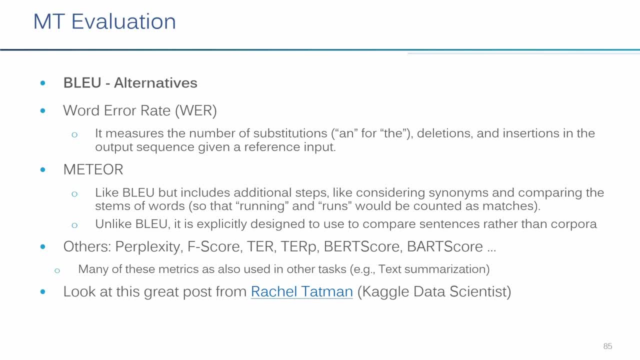 accounts for substitutions. accounts for substitutions: um we also have the meteor score. um we also have the meteor score. um we also have the meteor score, and, and so on, and, and so on, and, and so on. um there is this actually really nice. um, there is this actually really nice. 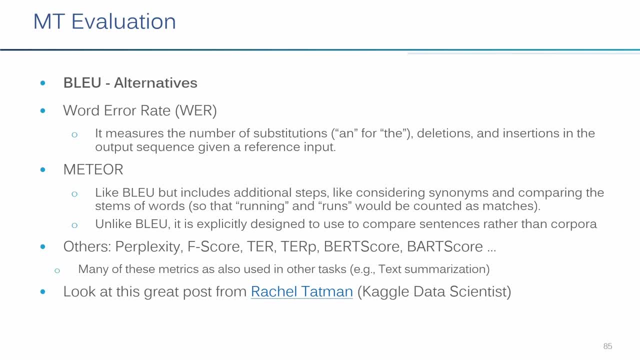 um, there is this actually really nice post about rach rachel tatman. in which post about rach rachel tatman? in which post about rach rachel tatman? in which she goes and give examples why you she goes and give examples why you.